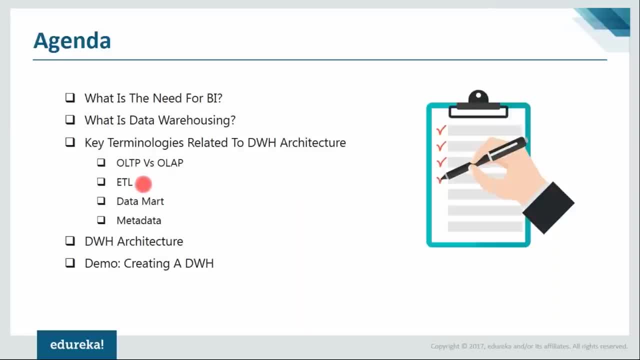 So that's about these two topics, and then we'll talk about ETL. So ETL stands for extract, transform and load. ETL is a strategy to convert your data from your database onto your database, Right, so moving the data from one place to another. that's all done by ETL. 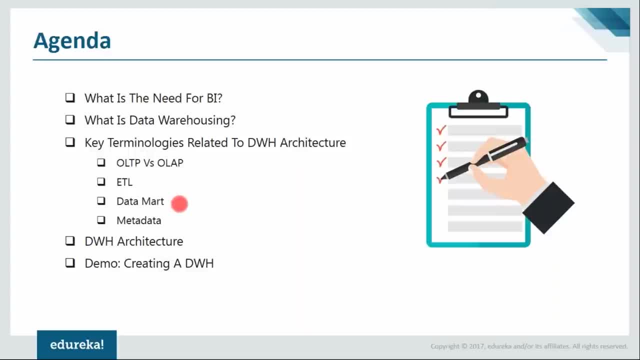 So we'll talk about ETL in detail, All right, and after that I'll talk about what a data mart is, and then what's at metadata. Now, these two things are two topics which I can only explain once I have given you an introduction to the other topics. 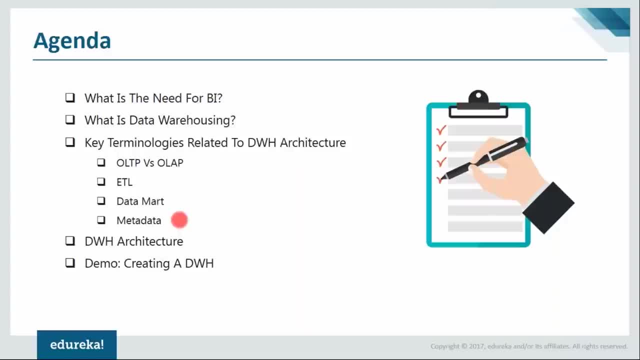 All right. So any of your tiny doubts that you have during the session, you can ask me at that time and I'll clear them right away. And once I'm done teaching about all these four different topics are related to data warehousing architecture. I will show you the complete architecture and the complete lifecycle of data. 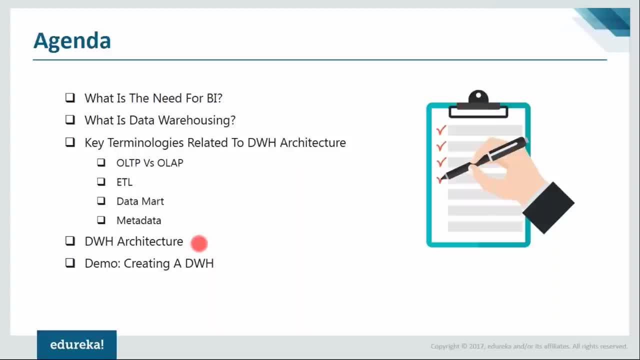 and What kind of insights your company can get and what kind of advantages you can get out of data warehousing right. So data warehousing architecture will be the last topic in my presentation, and after my presentation I will show you a demonstration of creating a data warehouse. 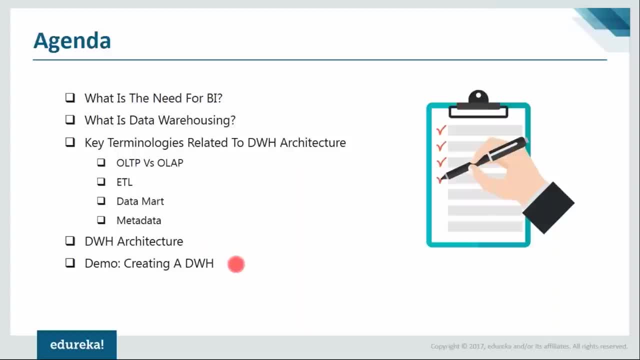 Where I will import data from a database and store it in a data warehouse right. So this will be the topics of today's session. I hope the agenda is clear to everyone. if you all agree with me, Please acknowledge that, and also do acknowledge the fact- if you can hear my voice and see my screen, 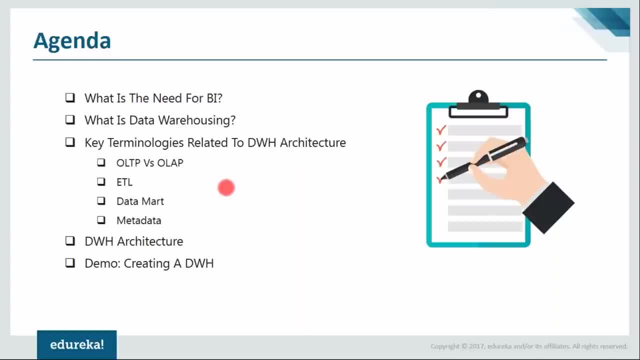 So if everything is fine, I can get started with this session. You can acknowledge and put any of your doubts or queries during the session inside the chat box that you see on your right side. So I'm getting a couple of acknowledgments from everyone. All right, so Rodney says yes. 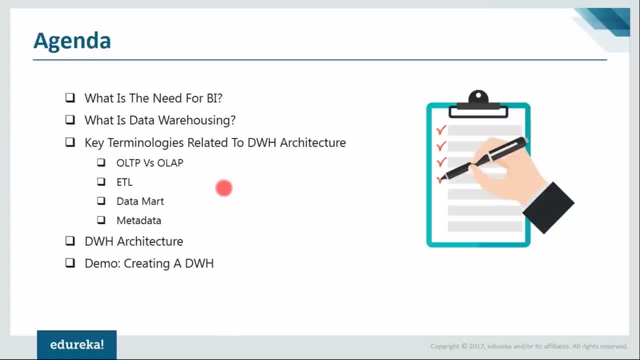 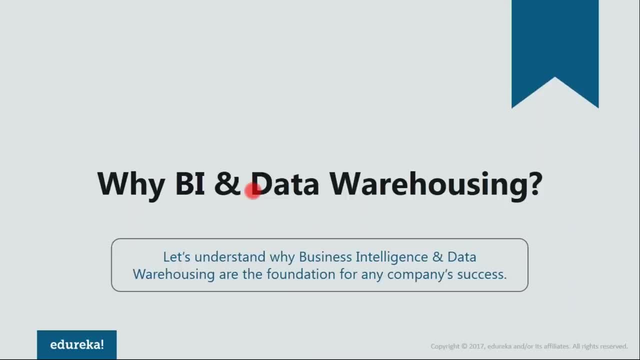 Rajesh says: yes, All right guys, and a couple more people are also able to hear my voice and see my screen. great. So since the agenda is clear, everyone, let me get started with the first topic, That is, what is the need for business intelligence? 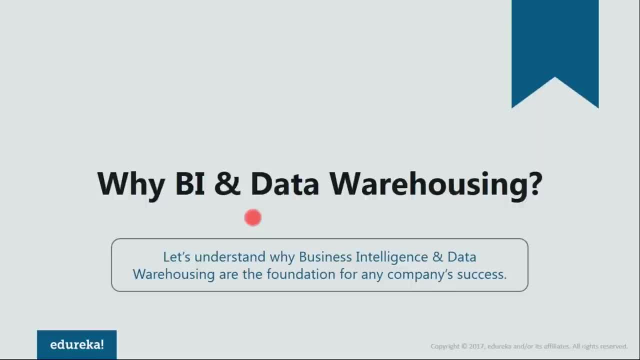 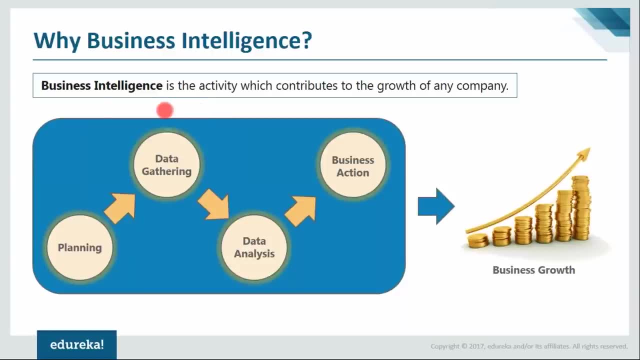 Okay, so we'll understand why business intelligence and data warehousing are among the fundamental and the foundation for any company success. So why do we have to go for business intelligence, right? Business intelligence is the activity which contributes to the growth of any company, and there are also so many MNC's which have been established. 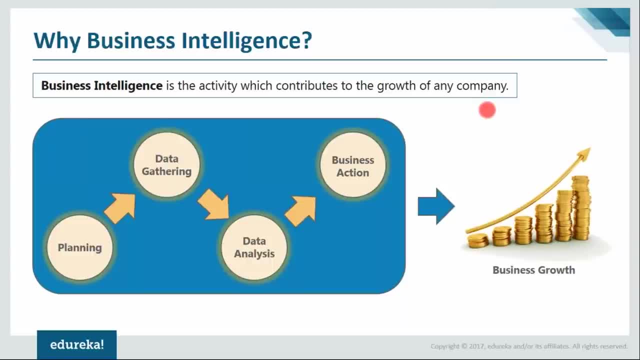 Over the past few decades now. how did that happen? They just didn't happen by luck, right? So they were all small ideas. There are small companies that start with a small idea and then they grow bigger. So that's what any company that wants to do good, That's what they do. 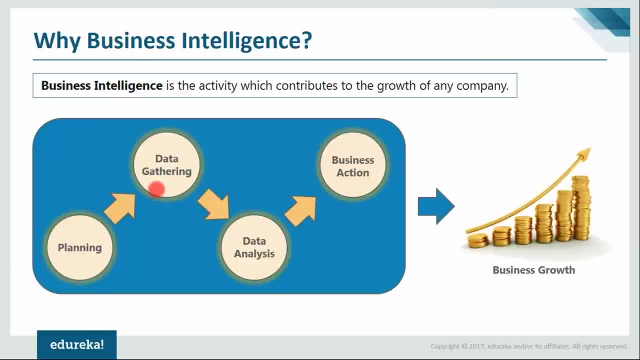 The first thing is they plan what they want to be and, depending on that plan, then they start gathering data. Okay, Now, once they gather data, they know they are in the right direction now, So they know what to do and how to do it, and then they do further data analysis on that. 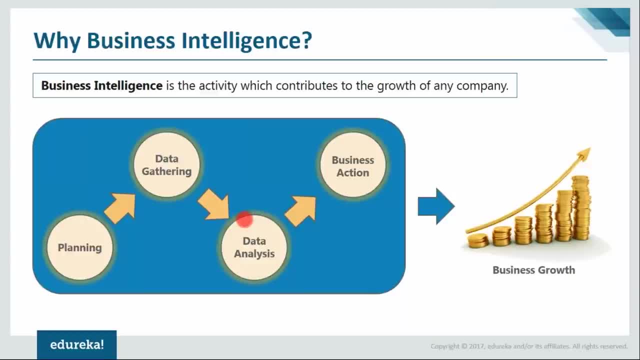 They make up their plans and they come up with strategies, They come to know what is the important thing that needs to be done, and all these things. So when they finally have a concrete plan, then they execute it into business action and once those actions are taken, then they're all good. 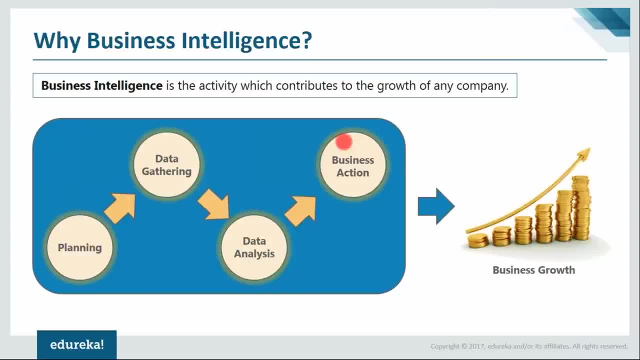 Right. That's when the business starts to grow. That's when the company gets back all their investment and that's how actually any company grows. So any company that has done well over the past Few decades beat Microsoft or Google or Facebook or Amazon sales force. all of these companies that have all grown from small ideas. 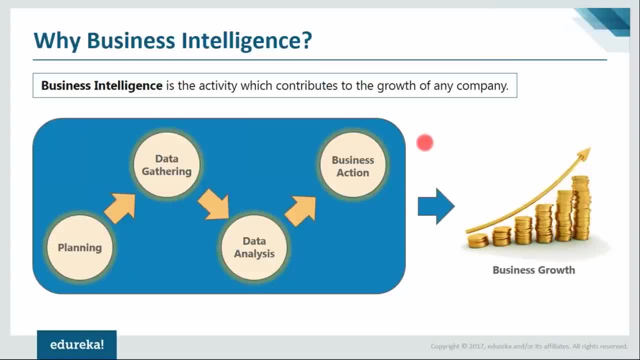 And they've become something big. right, and any startup that's also trying to do great nowadays. Even they have got off the same strategy and the same plan. This is a very common thing and this is something that everyone knows. Okay, But this is not what I've, you know, come to teach all in this session. 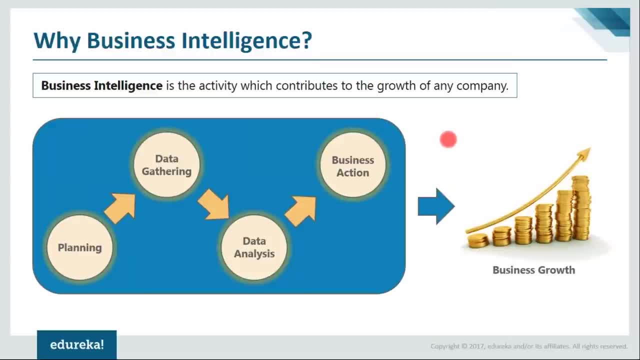 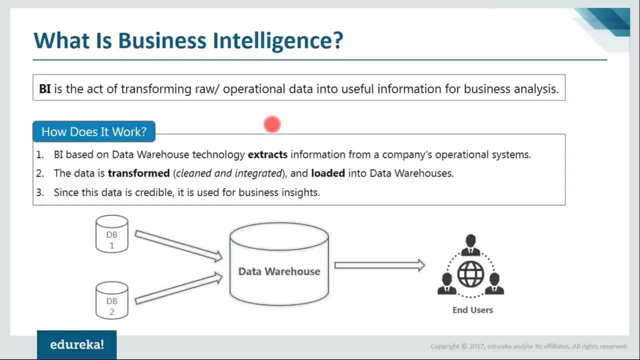 What I've come to teach all is something about data warehousing, and that is one of the most important strategies or activities, Which is part of business intelligence, right? So before I talk about Data warehousing, let me go into details of a business intelligence. So what exactly is business intelligence? 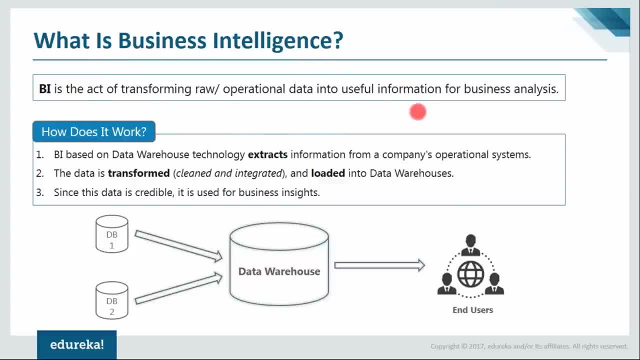 Bi is the act of transforming raw or operational data into useful information for business analysis, right? So bi here stands for business intelligence. That's the short form And, yeah, it is the act of transforming any raw or operational data. So when we say raw or operational data, it's basically the data that you've collected, the data that you have about your business. 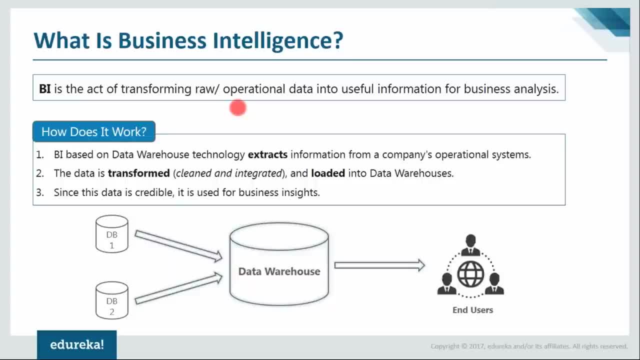 So it can be, even if your company is starting from scratch, then whatever data you've gathered. So you've kind of got to take that Data and convert that into useful information right so that you can plan and make strategies. and if you are a company, that's well. 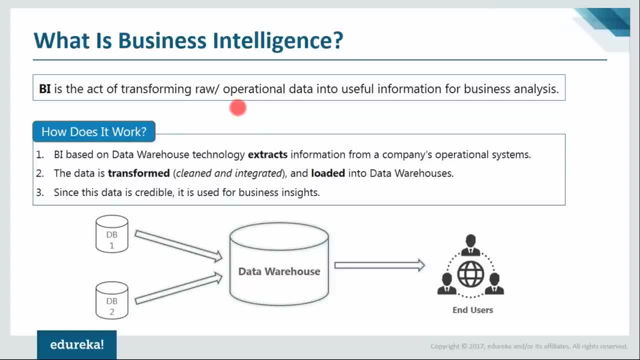 Established, then you have to look at your past results, How your company has done over the past six months or the past, the last quarter or the last year or two, and then make Come up with proper plans for your future. So when you do this, then this entire act is called as business intelligence. 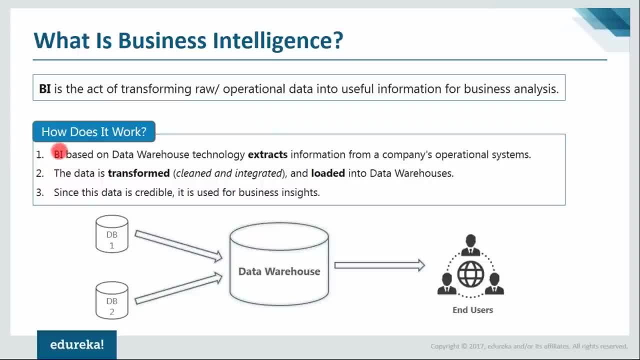 And how does it work? and this working of business intelligence is with respect to the ID technology. Okay, so bi, which is based on data warehouse technology. Okay, this is the key term that you got to remember. The bi is based on data warehouse technology. It extracts information from a company's operational systems and 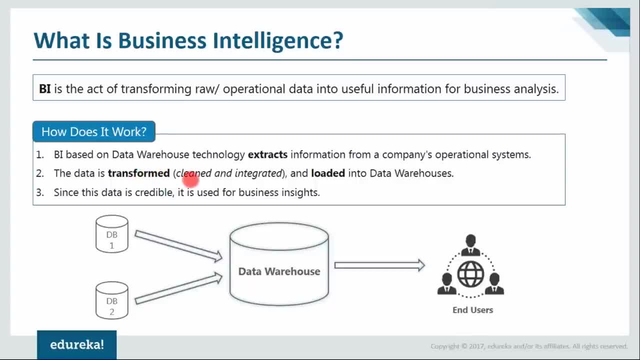 The data that is extracted is first transformed, and when we say it's transformed, It's cleaned and integrated and then it's loaded into data warehouses. Now the thing here is there'll be data in many forms. It can be the form of flat files, It can be in the form of databases. if it's a running company and if you're trying to do good, 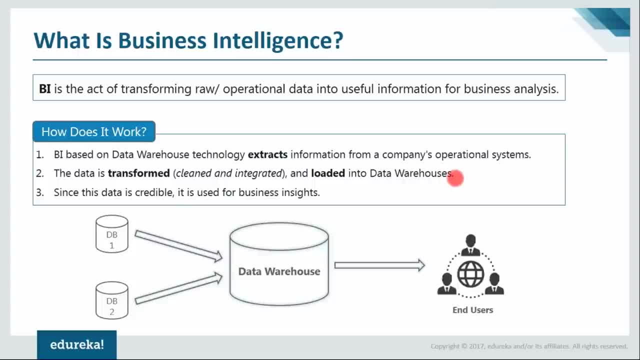 Okay, If you've been working for a number of years, Then you'll have data about your past success, about your sales data, your marketing data, your expenditure, all these things You might have stored in any form, maybe in the form of databases, maybe in the form of, for Excel's- flat files. 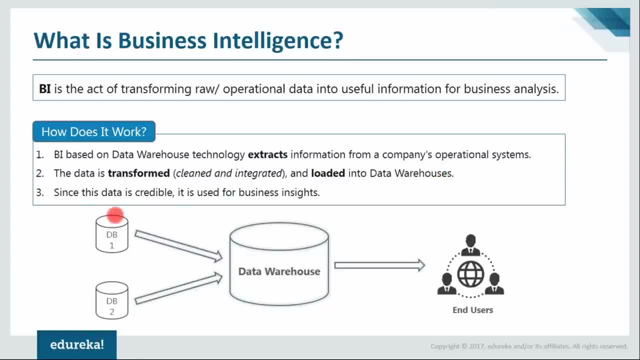 So all these things, so these make up your data source, right? So you have this data over here and this data is first transformed. Okay, it's of course. it's first extracted, Then into the data warehouse, it's transformed, which is cleaned and integrated. 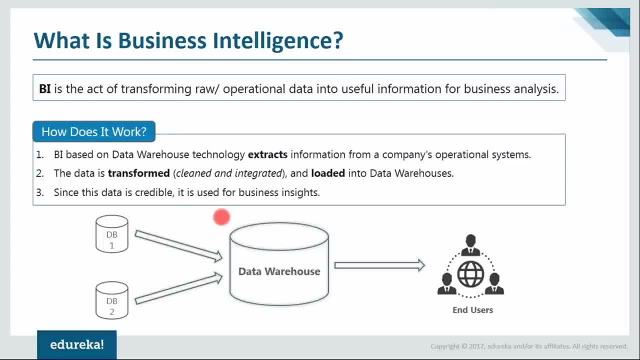 Okay, so once it's transformed, then it's ready for you to do your data visualization or data analysis. It's in a form in which you can get insights and this is the data which the end users will be using. So you will have your data analysts in your company, right? 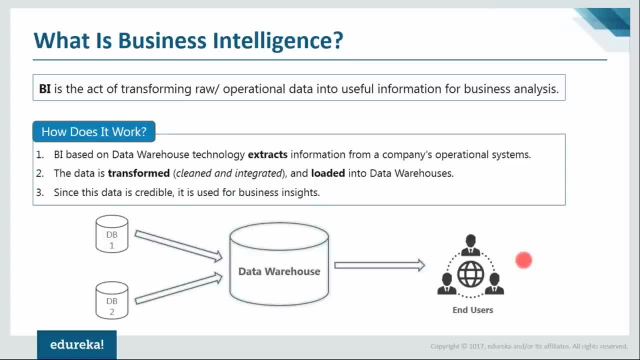 Your data scientists, your data analysts and all the other people, your managers, your rub and the other guys who call the big shots In your company. so all these people they'll be getting, they'll be using this data to make your analysis, and that's the role of data. 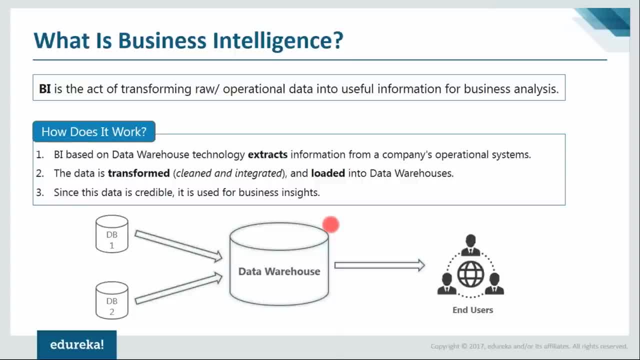 Warehouse. it is sandwiched between these two endpoints, and this serves as the basis or the springboard for success. And finally, since the data is credible, it is useful. business insights- Yeah, this is again something that I just spoke about, right? So now you'll have a better understanding of how business intelligence works, right? 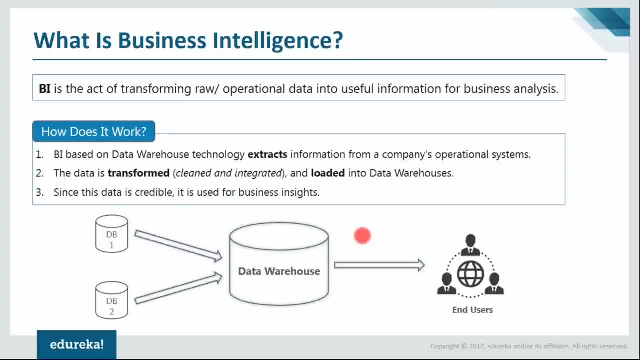 So you all know that business intelligence is something important, And how important and how good it is, how does it work, is what I've explained in this slide. So you all guys, all agree with me here. Anybody has any doubts. Rodney Rajesh Jacob. 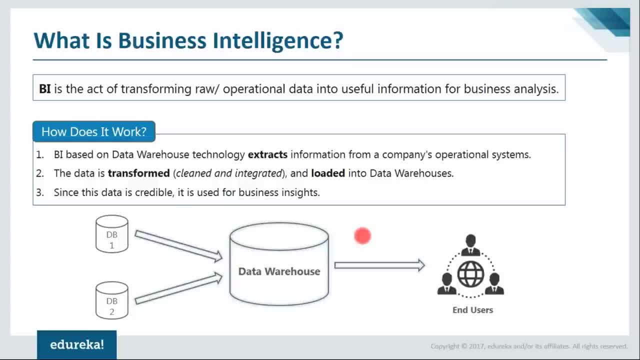 Okay, pretty good, All right, Nice. Okay, so I have a question from Jacob. Jacob is asking: is it ever? I was the only thing that's needed? Okay, Jacob, This is just an overview of business intelligence. Okay, the rough diagram, and it's actually not just data warehouse. So data warehouse is something that I'm concentrating on today's session. 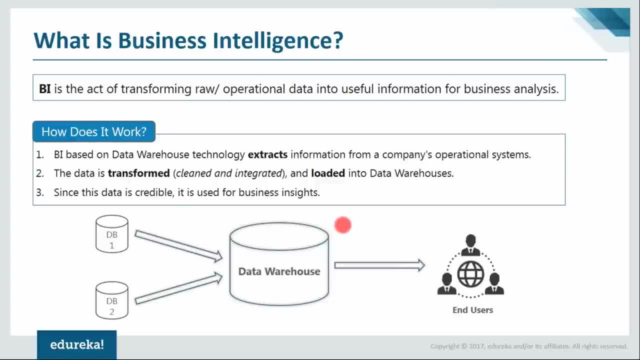 Okay, So that's why We have data warehouse. There's another important step called as data visualization, So that visualization is done by end-users. right, since it's done over here. It's not mentioned this diagram, But what you got to remember is data warehousing is probably the springboard. without data warehousing, 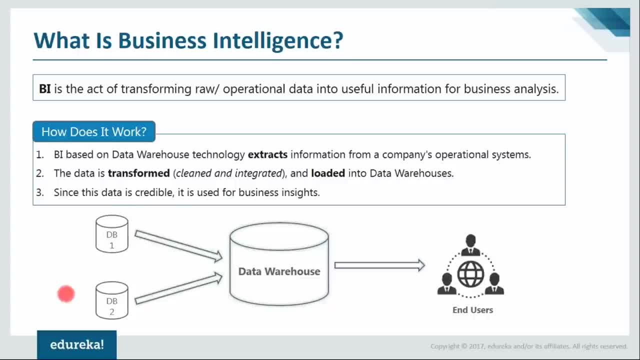 The visualization cannot be done and the data from the sources right from here. It cannot be directly used for any other purpose. So that's the rule of data warehousing. So that's what a data warehouses. And yeah, I clear Jacob now. Okay, great, That's fine. 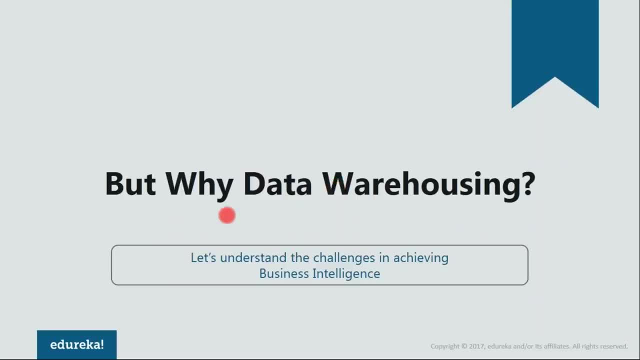 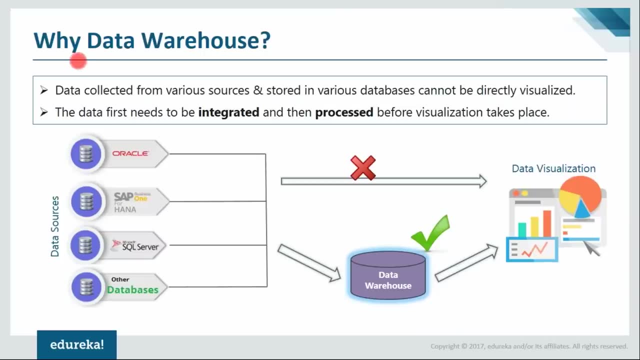 So let me go to the next slide then. Now you know what exactly is business intelligence. let's go to religious of data warehousing. That's sounds on the challenges in achieving business intelligence, business intelligence. So, first of all, why should we use the data warehouse? 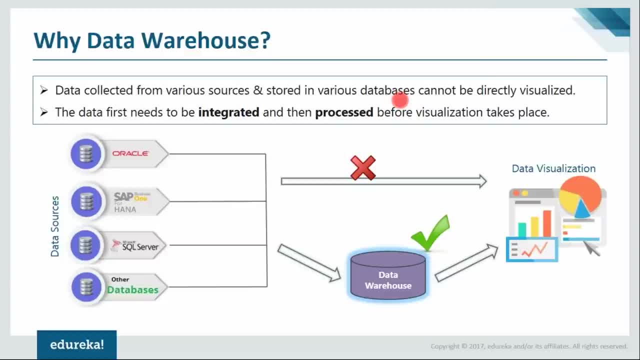 Because data collected from various sources and certain various databases cannot be directly visualized. Okay, Now look at this image. here in this diagram, We have different databases like Oracle, You have the sap BASE, You have the Microsoft tools over, and then your other databases like 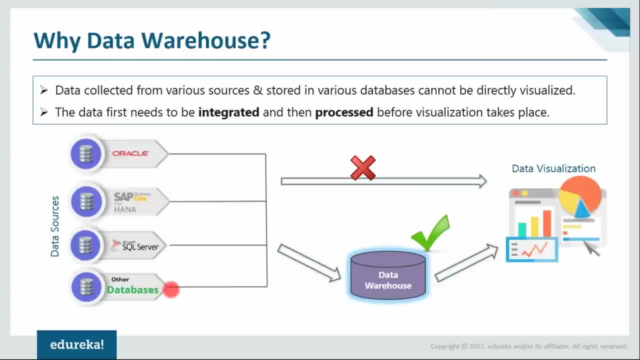 SQL databases and all these things. Okay, you can also have flag files in this list. So all these make up your data sources. you as a company can so data everywhere. So if you're a small company, you might just deal with Microsoft Excel and you might just use small analysis tools. 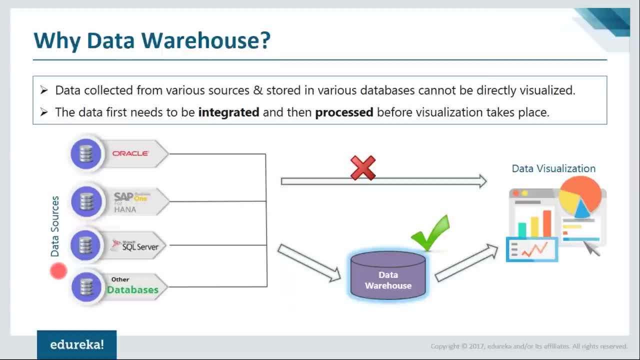 Okay, but if you're a big company, that has a lot of data coming in, So if you're a retail company, then you'll have to store details about your sales, your marketing and what's been your growth. So for all these purposes, you need big databases, right? So all the data will be stored in all these databases. 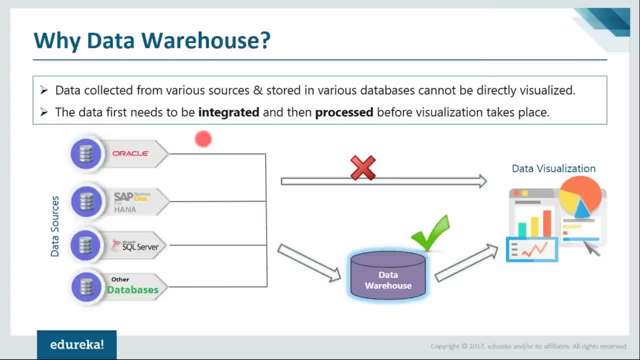 Okay, Now the problem is some teams in your company might be using one database and the other teams may be using another database. now the biggest problem that people would find while they are doing visualization or doing analysis, data is there in different databases and they'll have a. 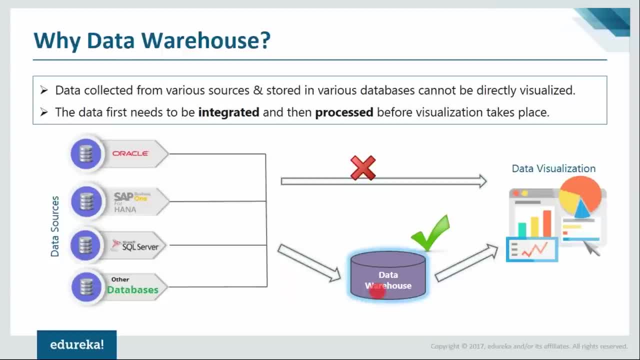 Tough time integrating them right now. That's where data warehouse comes in and that's where data warehouse course data Warehouse. it integrates data from all these databases and then processes that data and brings it in a form. It's very easy to do: visualization. Okay, that's what the second point says. 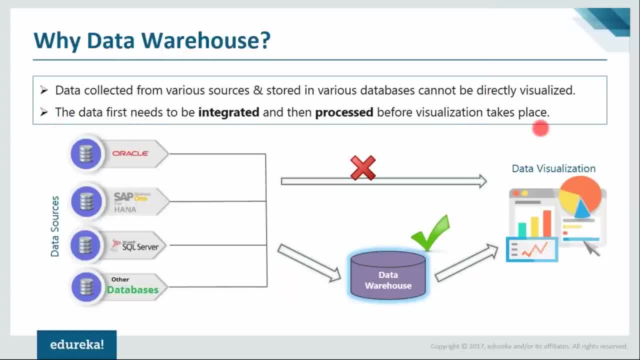 The data first needs to be integrated and then processed before visualization takes place. Now, this is the problem that you have with the regular databases. Okay, the data from here. They cannot be Directly used for visualization. and since data warehouse can do that, since it can integrate data from multiple data warehouses- 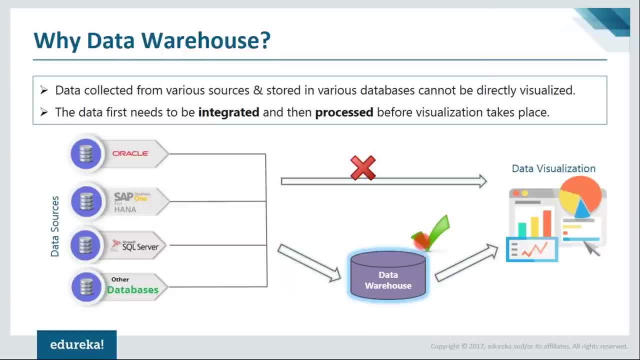 And since that data can be processed easily, since it brings the data in a form which can be easily visualized, That's where data browse has the advantage, That's where it scores. So that's the problem with database and that's the advantage that data warehouse has. In fact, data warehouse is more like an act. 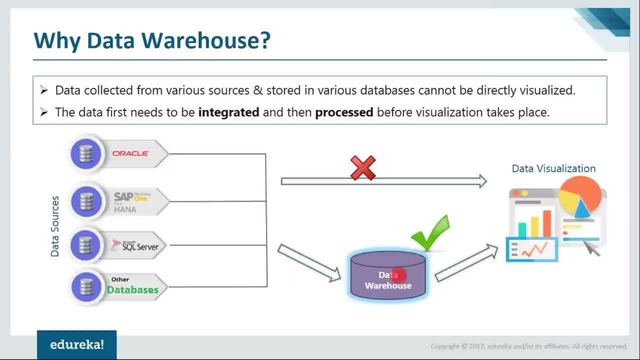 It's a discipline which is followed by people. Okay, these are actions which are adopted and strategies which are taken. Okay, that's what rate of warehouses, and that is the role it plays in Us doing very good visualization. All right, So now this should be a little more clear for people as to why data warehouse plays the key role in the whole bi aspect. 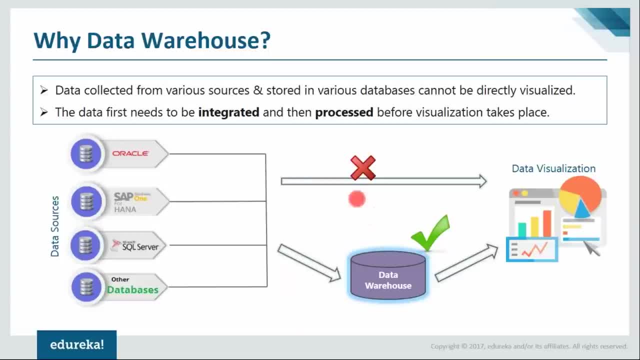 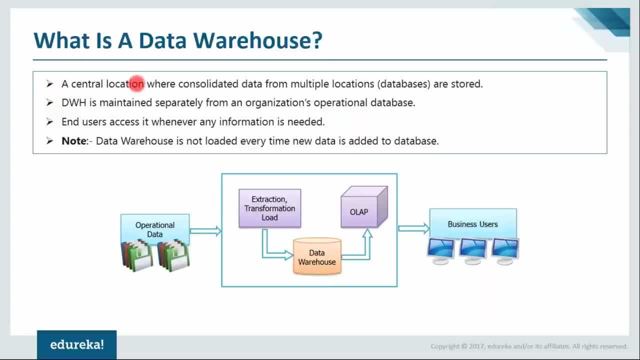 right, Okay, great, Let's go to the next slide then. now Let's understand in detail What data warehouse is now? a data warehouse? It's a central location where consolidated data from multiple locations- Okay, or databases, That's what locations mean- from multiple locations- are stored. Now, This means this is exactly what I explained earlier, right? 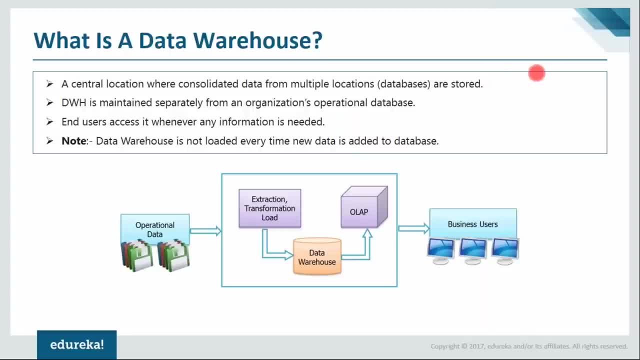 So you have a data that's coming in from multiple data sources, You have all the data, you consolidate all the data into one single place and the data warehouse is maintained separately from an organization Operational database. now, DWH here stands for data warehouse, All right, So, and here it says that data warehousing is maintained separately from an organization's operational database. 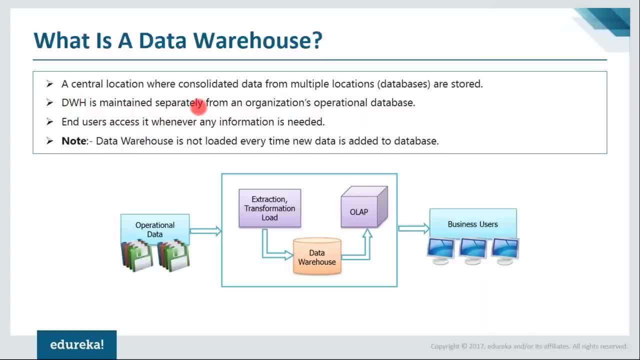 Okay and yeah. The DWH here stands for data warehousing, and the reason a data warehouses are stored separately from the operational database is because the data should Not get affected. So you will have your operational data and one end Okay, Where all your legacy data will be stored, where all your- even probably in your- real-time data will be stored. 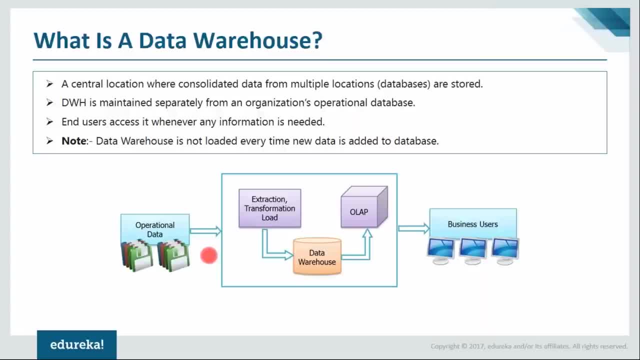 So all your transactions, all your sales, all your marketing, all your operations, data, All these will be stored in one place and in during the act of data warehousing. Where you're doing that, when you're making analysis, when you're using that data, you don't want that to get corrupted right. 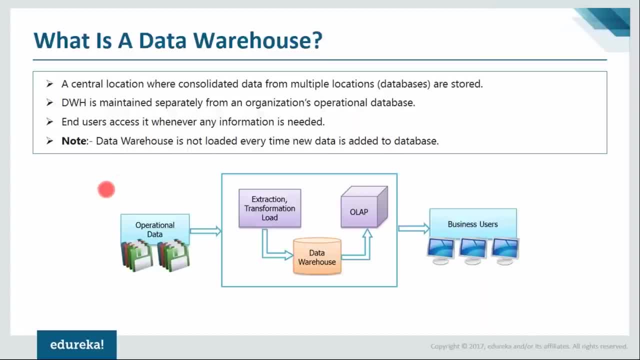 So it's more like a backup. So for backup to our purpose, your operational data is separated. So you have your operational data, you keep it in one area and then you create a new database. Okay, In fact it's called a data Warehouse. Okay, So you get all the data from multiple sources, or maybe from a single source, get it into a data warehouse and from here you 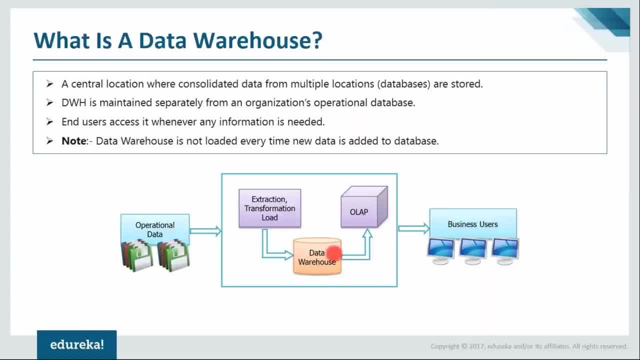 Do your analytics, So the process of getting the operational data into your data warehouse, that's called extraction, transform and loading. Okay, Now, when you've done these three things, you form your data warehouse, and from your data warehouse, you use the OLAP strategy. Okay, so OLAP stands for online analytical processing. 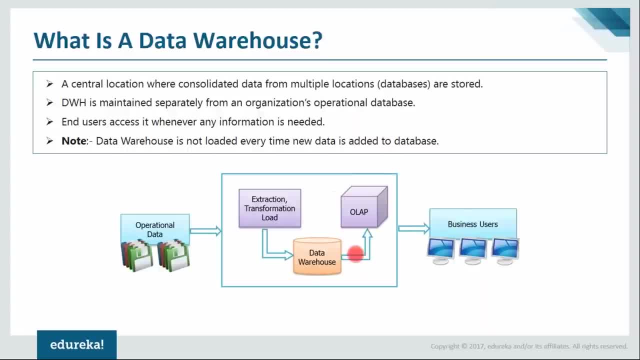 So you use this OLAP strategy or well, this analytics processing for the business user, Just to do analysis. So it's there in the name, right, It stands for analytical processing. So the business users, what are analysis they want to do? they do it because there is the option of OLAP and then, along with the 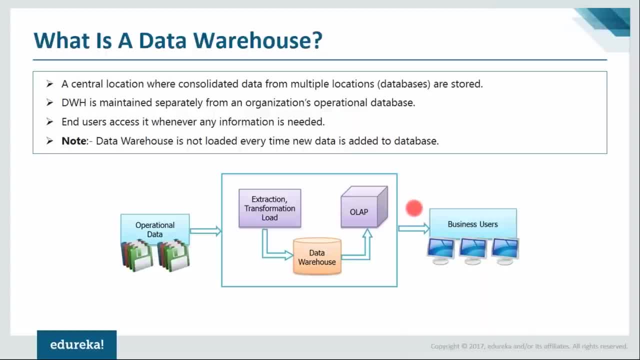 Analysis. they can also do visualization. for visualization, You have various the tools like tableau and click to you right. There are some amazing tools so you can get this data. You can get it into the data warehouse and the data warehouse also it can be stored in some kind of database. 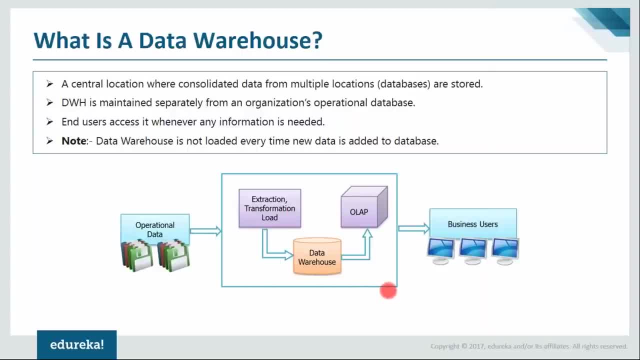 You can store this data back into some kind of oracle or sequel server or maybe even an excel, and when you've stored There, then you can do your OLAP activities there. And also you can import that data into your various visualization tools like tableau or click view, and thus you can, you know, get insights. 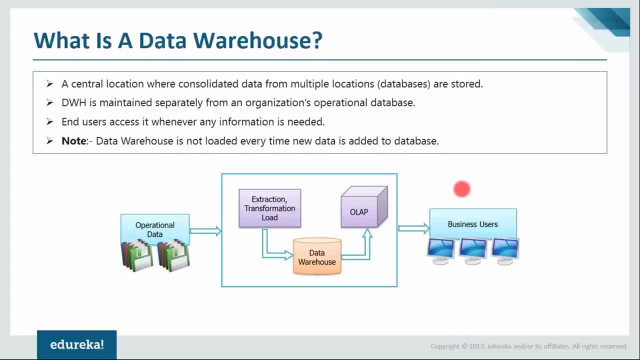 You can get insights into your data, You can deliver presentations during your board meetings, You can show your findings to your superiors or your managers. You can do all these things. So that's what a data warehouses Okay. and then the next point: we have yours and you just access it whenever any information is needed. 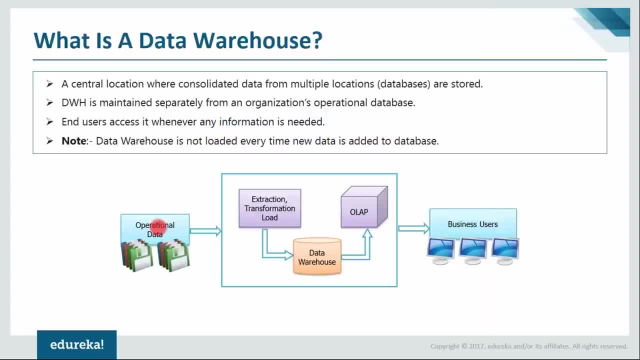 Yeah, so this is again the same thing, right? So once the data Comes in from the operational system, it's stored in the data warehouse. It stays there. So this data is not going to change. So whatever change you want to route your operational data, that can be done. 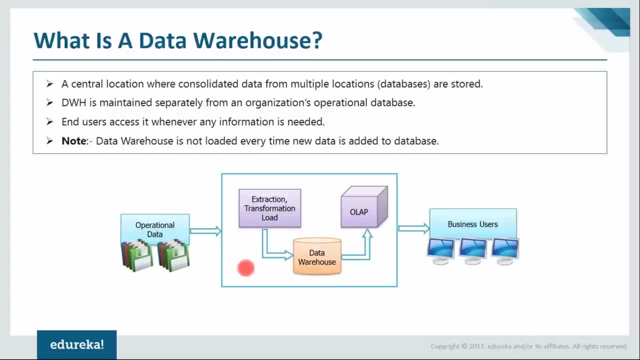 Okay, you can modify this data, You can update it, You can delete data here. You can do all these things, but once your data comes into your data warehouse, it cannot be deleted. Okay, you can maybe modify things. the worst case scenario: You can modify data here. 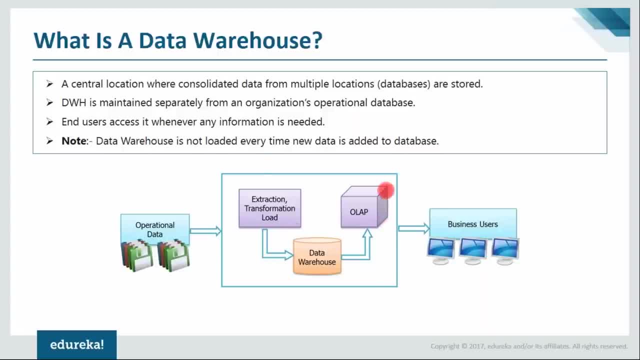 Okay, but it's highly advisable not to. but of course you can. so that's the thing. But yeah, the key point you gotta notice, the end users can use it anytime. They can probably access a data that has 10 years old or 20 years old and all these things. and how can they do it? by using OLAP. 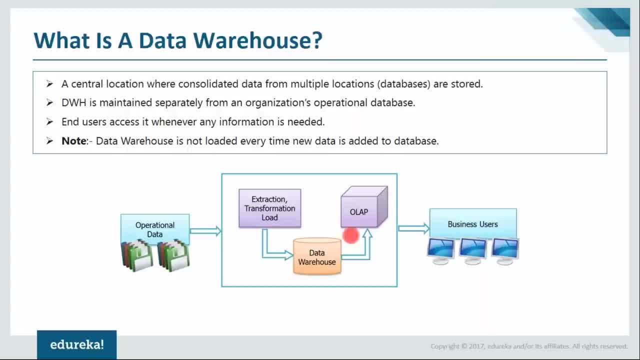 So they can do the analysis and they can run it over different times, right? So these are a series of snapshots, So, based on you can find data analysis like what happened at this particular day, on this particular year, all these things. You can see what kind of product was sold. 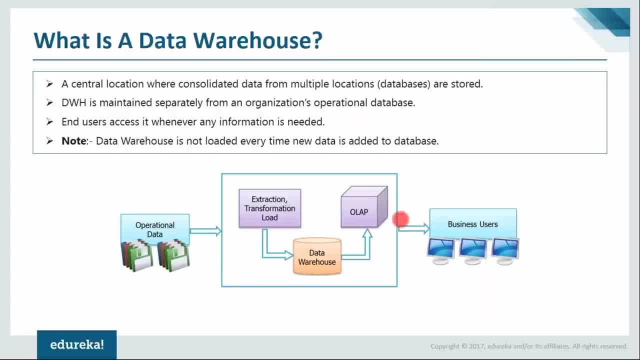 How many customers bought which product. all these details can be easily gathered and access from here. So that's what we say: when you know The data can be accessed at any time by the end Users are the business users. So the business users here are typically those of managers. 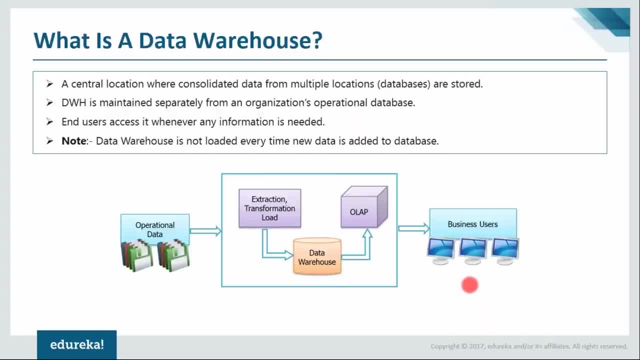 It can be managers or people who are leading board meetings, who are making a plan for the next quarter or the next Half year, or the next one year, on all these things. So, guys, yeah, that's, that was a question which Jacob asked guys. So, Jacob, as will be the end users, who will be the business users, So that's what they are. 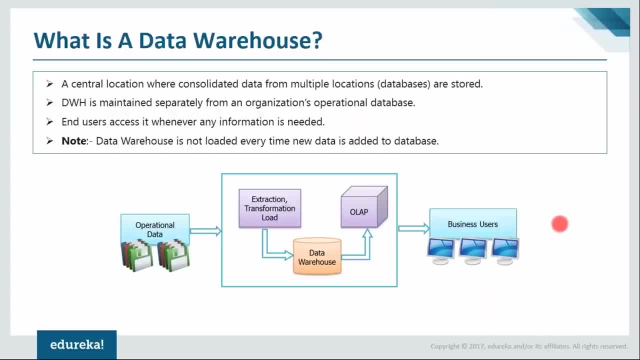 Okay, people will be using this data. It can be even data analysts or data scientists and all those people. right guys? Are you clear, Jacob? Okay, great, and there's a note. Okay, the data warehouse here. It is not loaded every time when new data is added to the database. 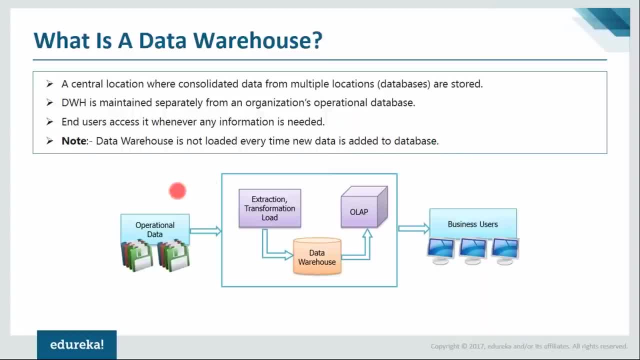 So what this means is you have data coming in your operational data. Okay, This operational data will get updated every minute, probably every second. if you have a 24-7 working sales team, Then they'll be making sales around the clock, right? So as in when any sale happens, the data will be added to your database, your operational data. 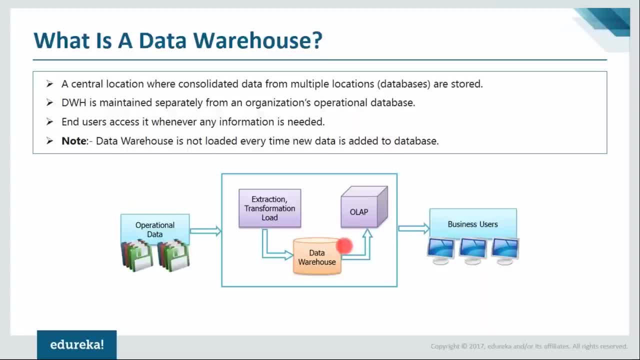 But that not necessarily needs to be added to your data warehouse also. So what you find in your data warehouse is legacy data, right, It's historical data which you can use to perform analysis or all those find insights, the operational data, If you have new data coming in here. 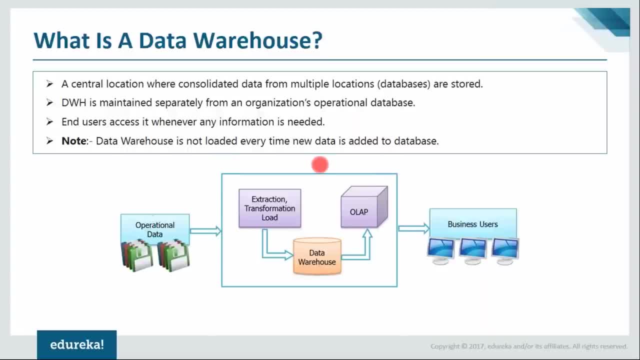 This has be important, and this has to be moved to your data warehouse first, And then, once it's smoke your data warehouse. from here It can be used for analysis and all these things by your end users. So that's what this diagram here means, and that's what the last point also means. 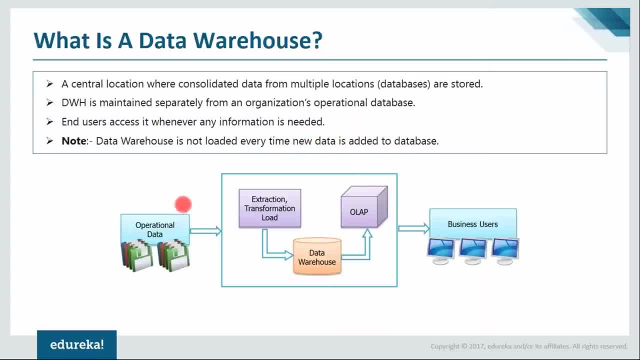 Okay, data where ours is not loaded every time new data is added to this database. okay, so, So I hope it's all clear. Rodney, Rodney and Rajesh: Okay, great, so fine, then, If you guys have understood what a data warehouse is. 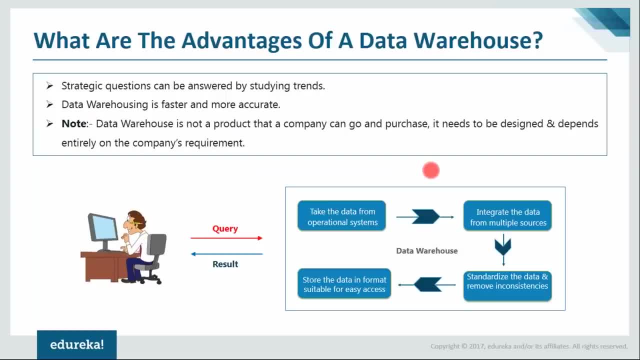 I can go to my next slide and talk about the next topic. So that was about data warehouse. Now let's look at the advantages of a data warehouse when we compare it to any database or just regular flat files and all these things. The first advantage is that strategic questions 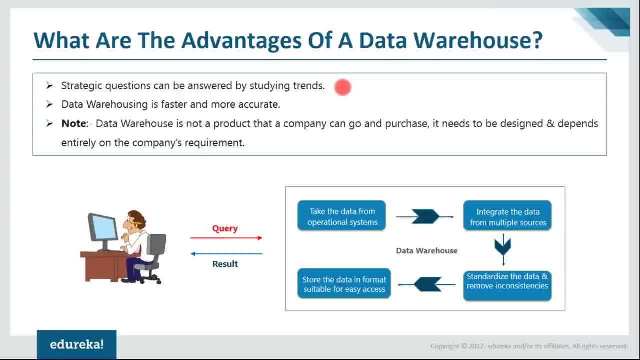 can be answered by starting trends. So this is the biggest benefit that you can get right: Your data analysts and data scientists. they can answer strategic questions. they can read the past data. they can predict your future also by coming up with. 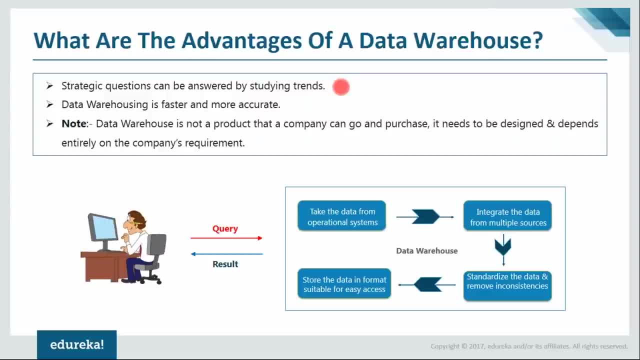 by having their strategic questions be answered, Because trends can be analyzed using the data warehouse. It's basically the data that is stored in your operational data also, But it's just that it's easier to study trends on your data warehouse rather than database. okay, 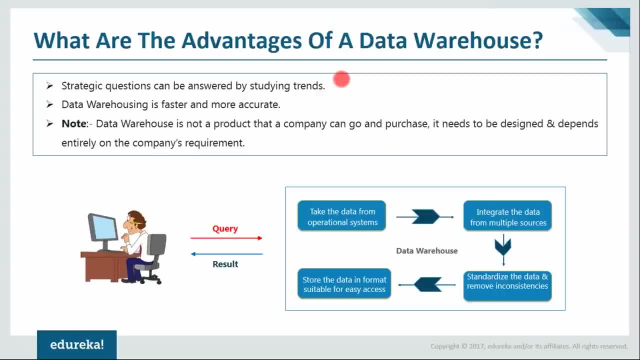 Because Rajesh here has a question. guys, Rajesh is asking: why not a database? What is it that a data warehouse can do that a database cannot do? So, guys, that's what I was answering, correct, Rajesh, remember? the first thing is: 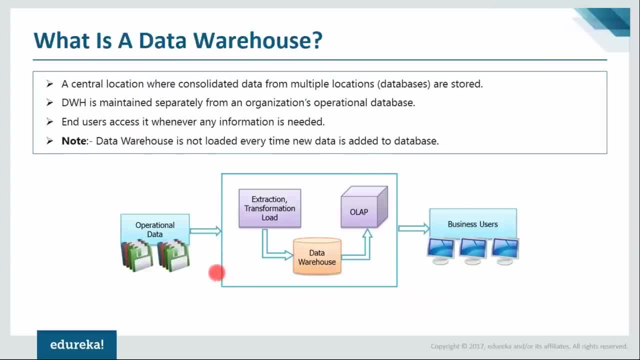 let me go back to my previous slide for this. okay, So you have your operational data here. So you have all your data here, which is probably legacy, which is even real-time. All these things will be present here, But in your data warehouse. 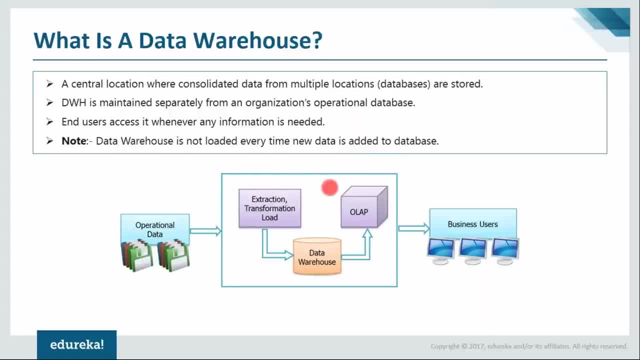 you'll only have your legacy data, You'll only have the historical data. You won't have real-time data here, But that doesn't mean it's any lesser than operational data. Since you have your data completely here, you have the freedom to do your analysis. 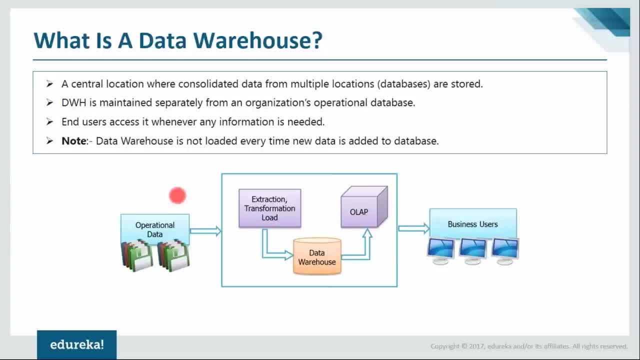 and you also have your freedom to do your data visualization. Okay, so that's one advantage, And the other advantage with the data warehouse is that your data will be coming in from multiple sources. right, We'll have data coming in from multiple sources. 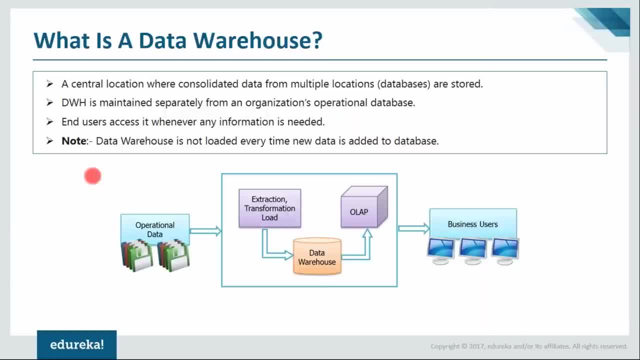 Your tables will not be related to each other, Even if it's from the same database. you'll have multiple tables for multiple teams, right, And you can't easily integrate all these tables because they'll be separated. okay, That is one big problem that you will face. 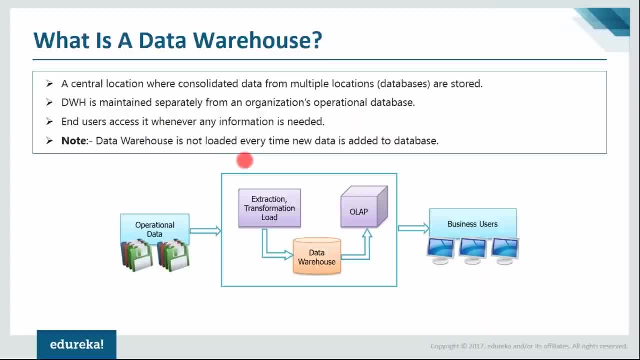 when you're doing the analysis or visualization In a data warehouse. it'll be stored such that all the data will be interlinked right. It'll be related by using schemas or all these things, So you have different schemas, like star schema. 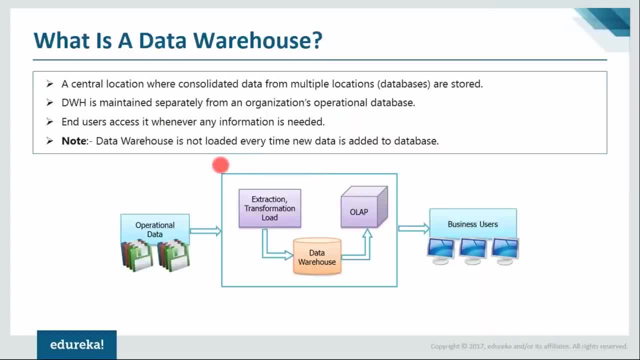 snowflake schema, galaxy schema and all these things. So you have all these dimensions and facts, all these concepts using which you can relate your tables, You can relate your data, So all your rows and all your columns here which are unrelated, which are stored in separate databases. 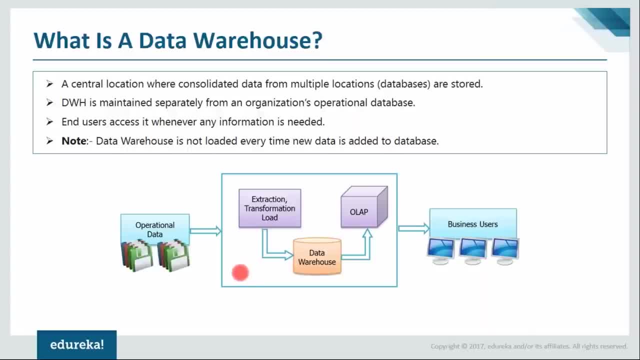 or in separate flat files, separate tables. they can all be integrated, They can all be stored together. So there'll be a relation. So every single row or every single table will be linked with each other. And when you do an analysis like that, 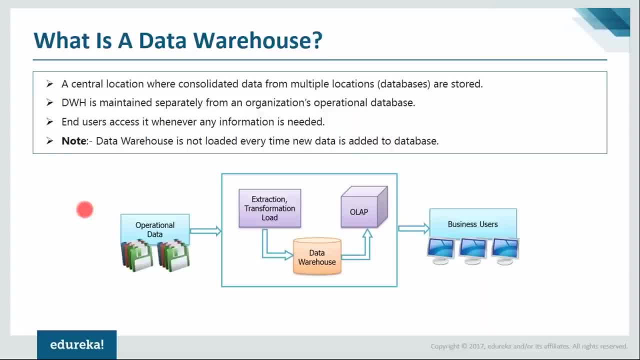 then you can probably pull data across the database, right? So whatever data is stored across the various databases, you can put all that data and link them all together by running one query, and you can get all those details in just by just running one single query. 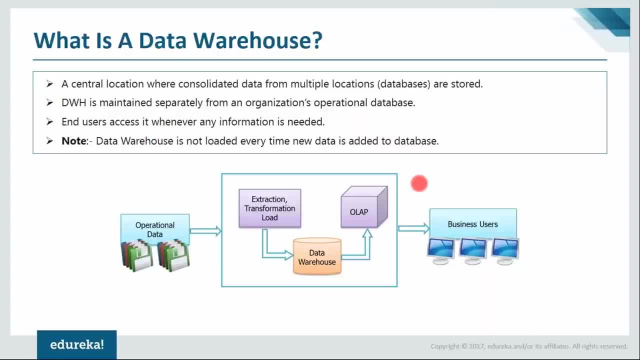 using your data warehouse. So that is the advantage, Rajesh. right, So did you get it, Rajesh? This is the second advantage. okay, That's why business users, they prefer to use data coming in from a data warehouse. 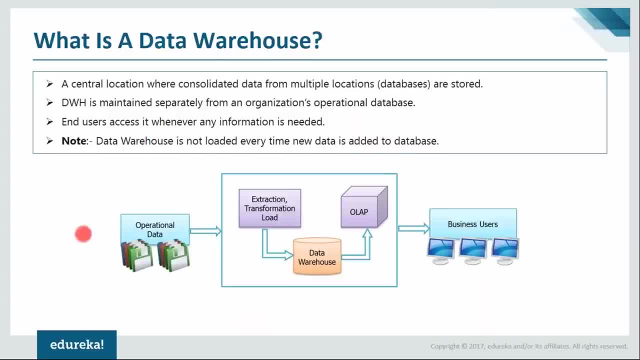 So this is a more structured and this is a more related data when you compare it with the operational data and the basic data source. all right, Fine, fine, fine, very good. very good, Rajesh, I hope you've cleared your doubts. 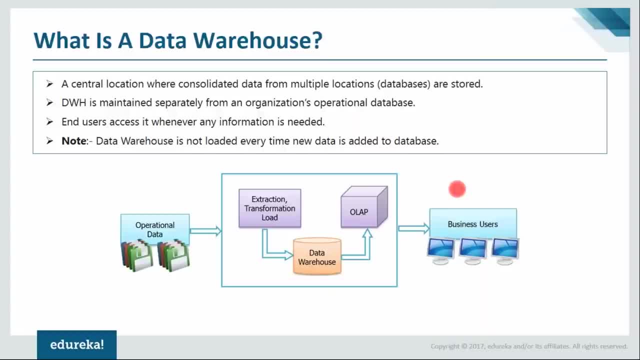 I hope that the same thing with even others. right, Okay, even more clear. great great Rodney's telling. now I've got it even more clear. Fine, fine, very nice. That was a very good question. Good you asked me that. 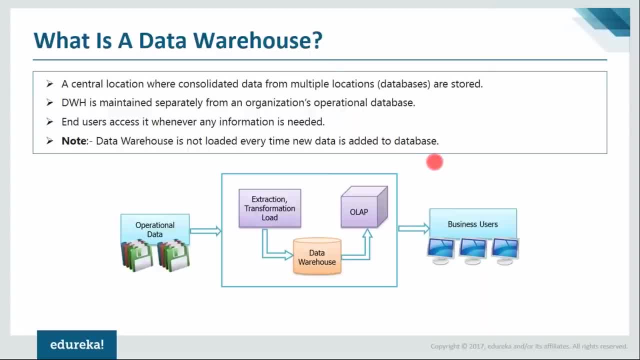 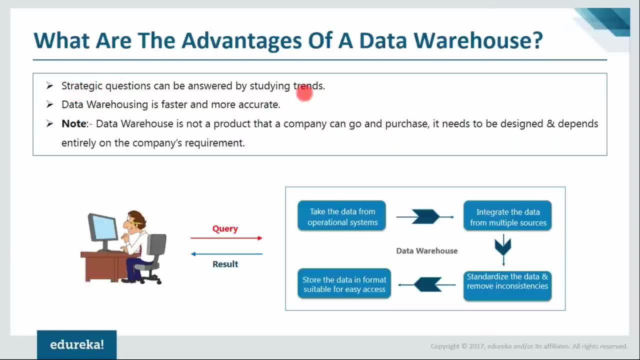 And yeah, I'm glad you stopped me because I could explain it in a better way. So, anyways, moving on, that was about data warehouse And talking about the advantage of data warehouse. I spoke about the fact that you can answer strategic questions by studying all the trends. 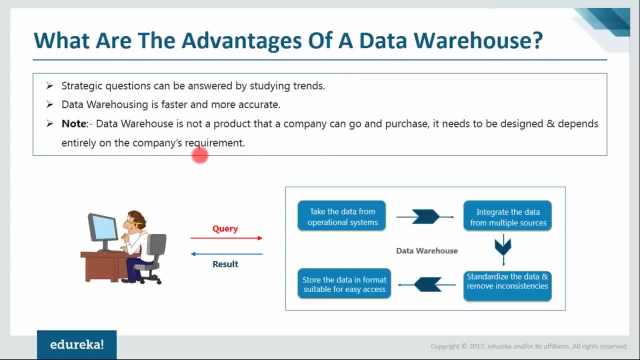 by studying your past data, You can have all the graphs. You can have the pictorial representations right. You can see whether the trend is growing or not, which product is getting sold, how better it's getting sold. All these things you can easily read. 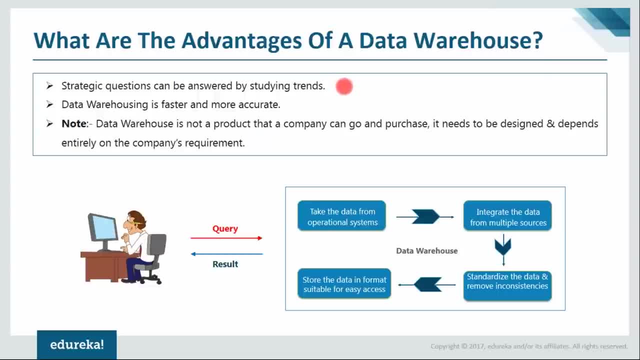 by using a data warehouse, because data warehouse makes your data more readable- information. So that's the thing. So you guys must know the difference between data and information, right? So information is something that is processed. Processed. data is called information. So information is easier to understand. 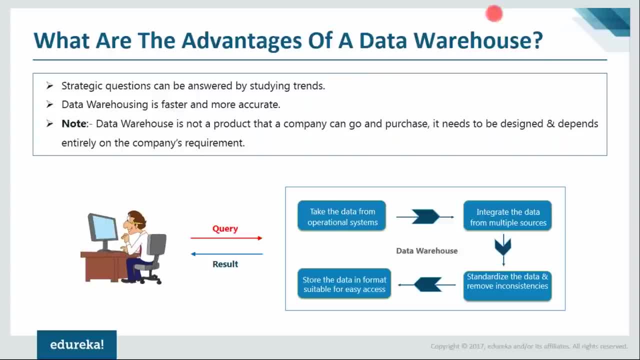 easier to relate to and easier to use. Now, that's what data warehouse does. It takes you one step closer to information, right? So that's the advantage. And yeah, the other thing is data warehousing is faster and it's more accurate. 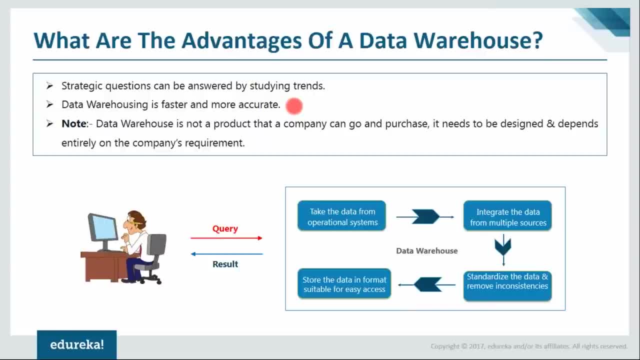 Yes, this is something that's completely true, because in your database you'll have loads of data. Of course you'll have historical data and real-time data, but the thing is it's not gonna be as fast as data warehouse. Data warehouse- you'll have links there. 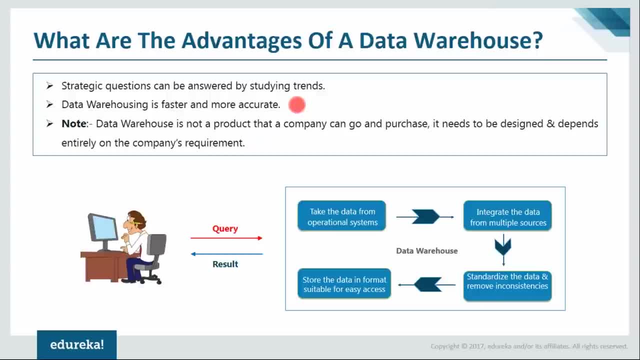 you'll have links, you'll have tables, you'll have relations between the various tables and because of all these things, you can easily gather and you can easily access data here And the data that is gathered from here. it's also more accurate. 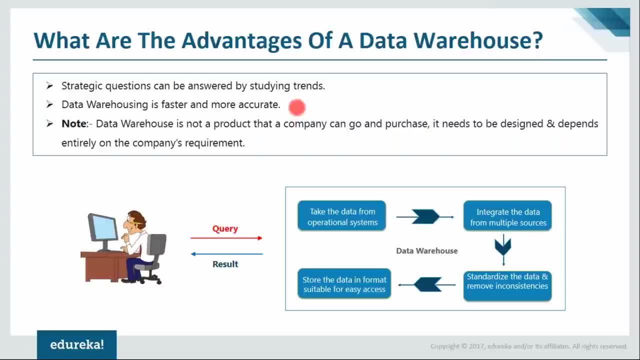 because there won't be much change, because there's not gonna be any question of real-time data coming in and changing things around. All right, so you made it. So, whatever you know process you're using, right, You know processing or analysis. 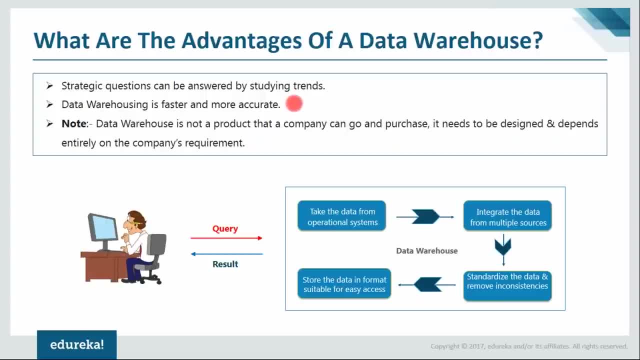 it's done based on the past data that is stored in the data warehouse, and that makes this data more accurate. It makes it more stable. So stability is the key word here, and stability is not something that you can have all the time in database. 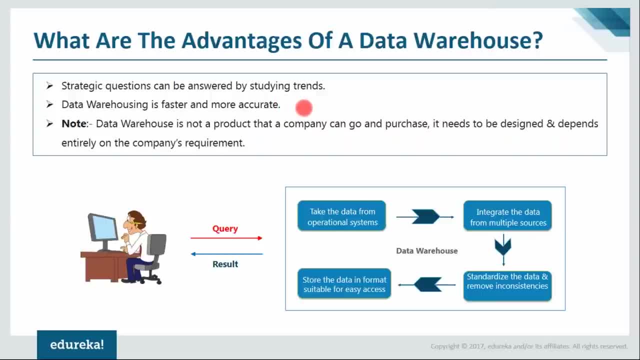 but you will have it with the data warehouse. So that's the second big advantage, And in fact, there are many more advantages, right? So data warehousing is something that you guys will understand when you start implementing. So in the demo session that I'll show you later today, 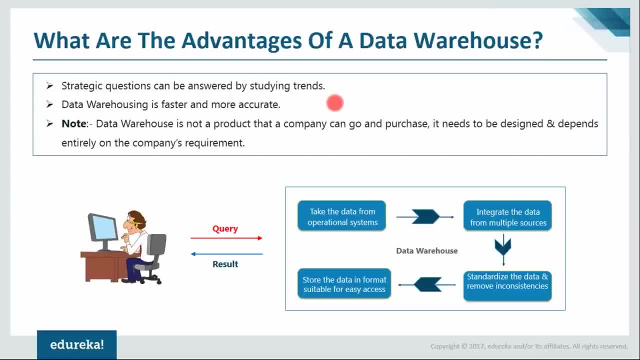 that time you'll understand, you know, you'll understand- the other advantages with data warehousing. okay, And one important point that you need to notice: that data warehouse is not a product that a company can go and purchase. okay, It needs to be designed. 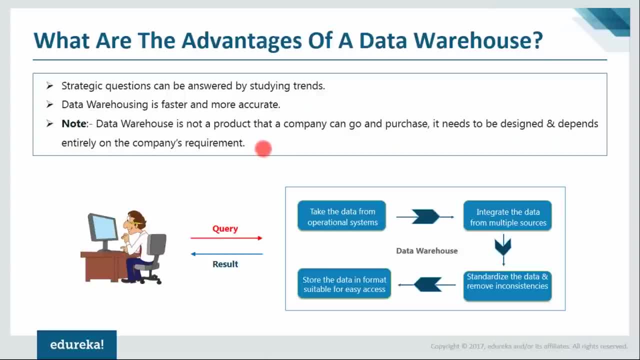 and it depends entirely on the company's requirement. So, like I said, your database is something it's a necessity, right? Your database, or where you're storing your data, Your data source, is something that you have to have, and then your data warehouse is something that is designed. 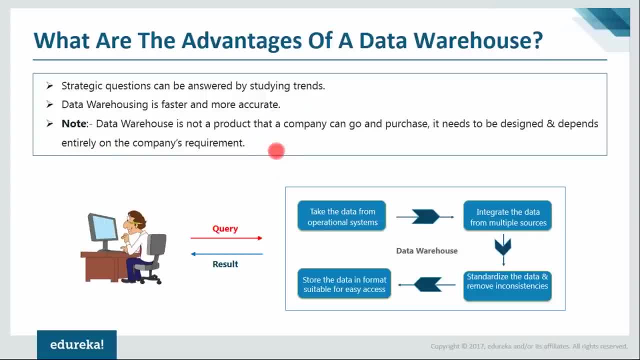 and which completely depends on your company's requirement, Based on your data source, based on the requirements that you want to get of your data source, out of the data that you have in your data source, you can come up with a way to design your data warehouse. 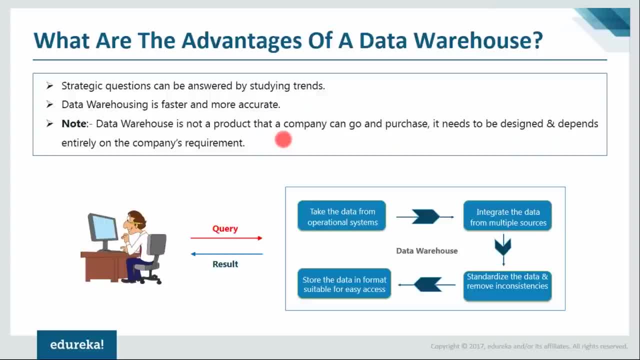 So data warehouse is more of a concept and it's a strategy and it's not an end product. It's not a tool or something that you can use. You have multiple tools to implement data warehousing and the thing you gotta notice- 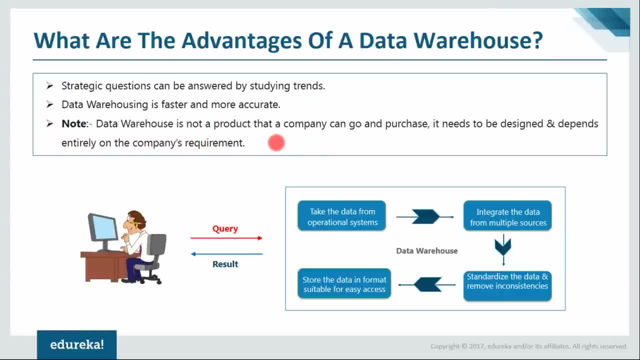 data warehousing is not a product. okay, So it's a strategy that you adopt to make your data more readable and make your data in a better fashion. Okay, so that's the biggest advantage with data warehouse. So look at this guy here. 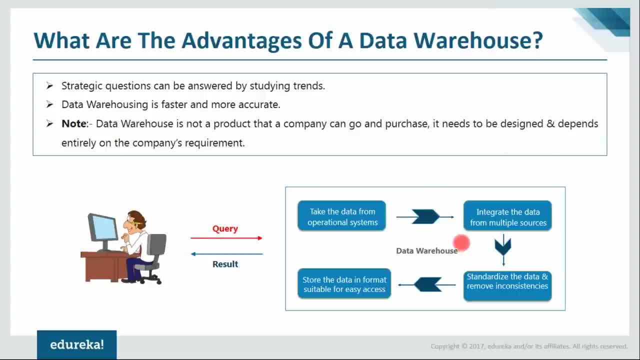 Okay, he'll just run one query on the data warehouse. Okay, now what the data warehouse will do. the data is taken from the operational systems, all right, And in fact, if there are multiple operational systems, then all those multiple data. 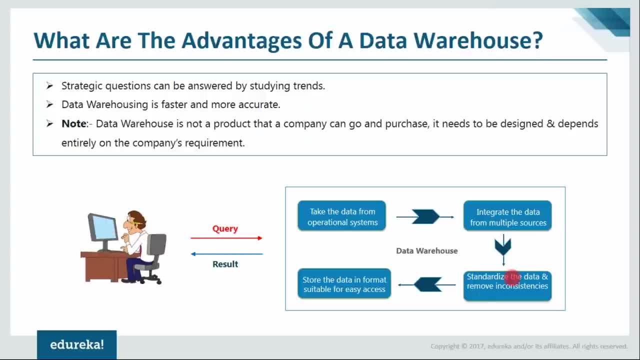 from multiple operational systems will be integrated together and then that will be standardized and any inconsistencies there in that data will be removed. Okay, now, these are the three important things: The data is taken from the operational systems and that data if there are multiple operational systems. 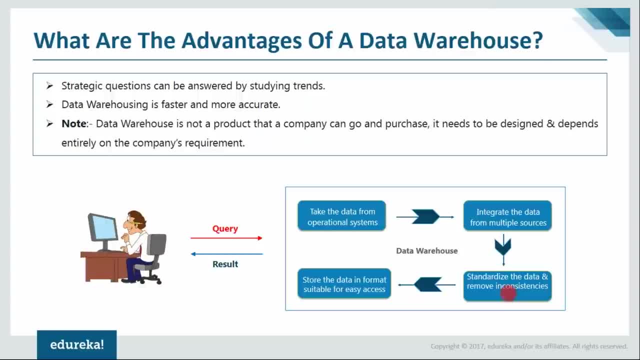 those will be integrated, okay, And then the data will be standardized and any inconsistencies will be removed, And once all these three things are done, then it can be stored in an easy format which is very suitable for analysis and access, And that is what a data warehouse is. 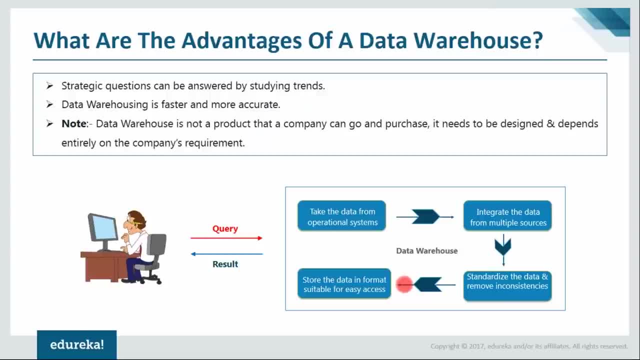 So whenever he runs a query on this kind of data warehouse, which is a process and which is ready in such a fashion, you can get the result quickly and this result will also be more accurate. all right, So this is the big advantage with the data warehouse. 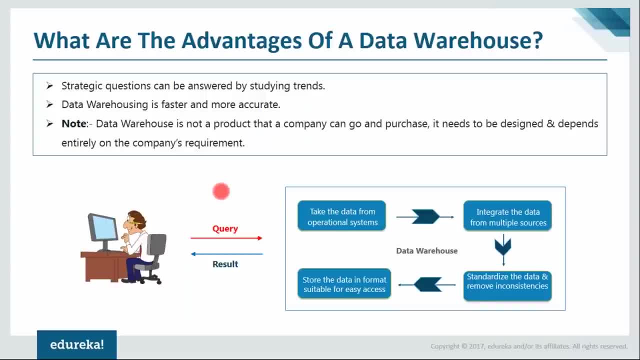 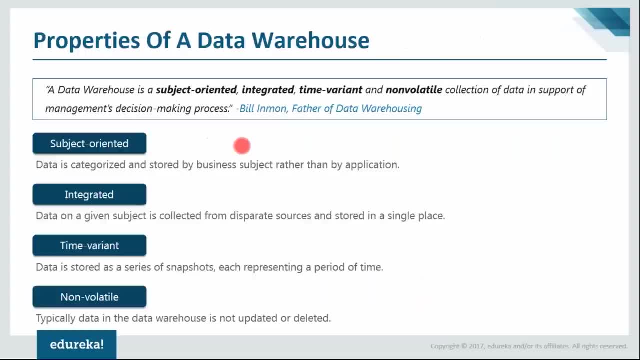 So I hope this is clear. It's a pretty simple concept here and it's just an overview of what I explained in the previous slides. right, Right, Jacob Rajesh Rodney. All right, Okay, so moving on, There are four important properties. 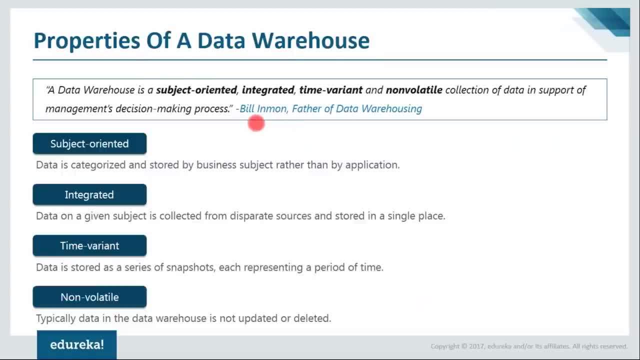 that a data warehouse has. okay, And these four properties are based on what Bill Inman said. Bill Inman is the father of data warehousing and initially he defined data warehouse as a subject-oriented, integrated, time-variant and non-volatile collection of data. 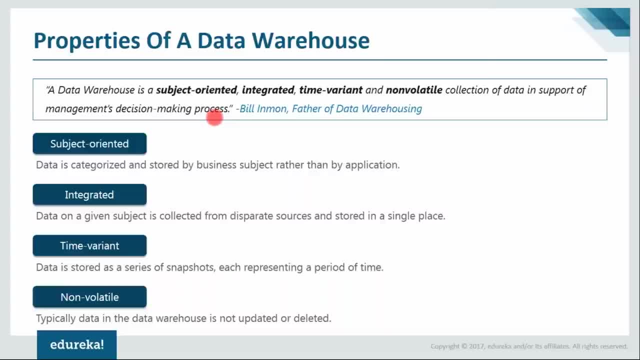 in support of the management's decision-making process. okay, So when we say subject-oriented, it means that the data will be categorized and stored by the business subject rather than by the application. Now let me get back to this point after I finish these three. okay. 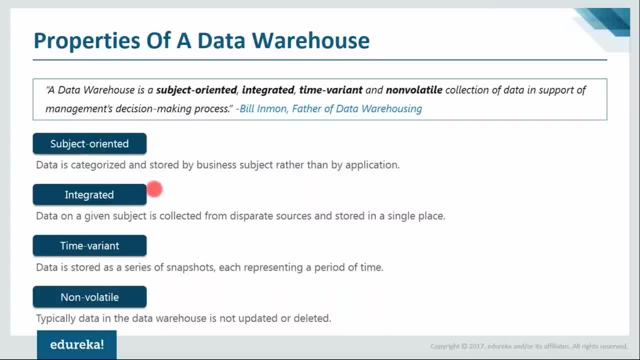 Now, this is the most complicated point. okay, Now, talking about integration, right, He said that data's integrated. So the meaning here is data on a given subject is collected from disparate sources and stored in a single place. So this is something you people know. 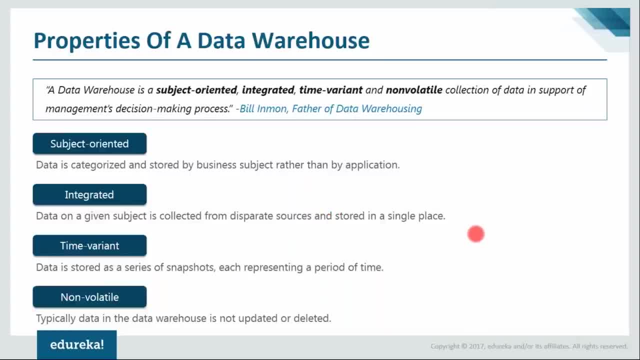 Data's collected from multiple sources and they're all stored in one single place, So you don't have to, you know, go about searching for data in different tables or different sources and all those things And then your data. it is time-variant. 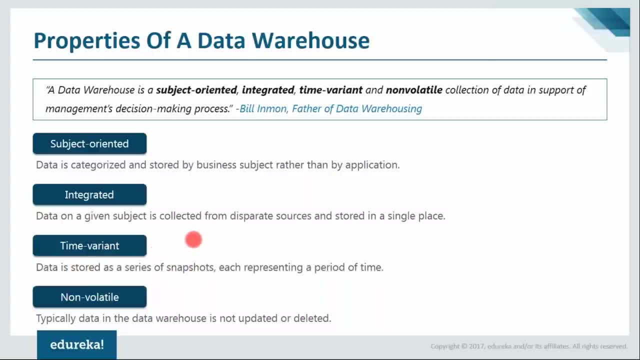 It is stored as a series of snapshots, each representing a period of time. So when you do your analysis, you can do it based on a series of snapshots of time. okay, You can see what was your company status on this month that year or on this month this year. 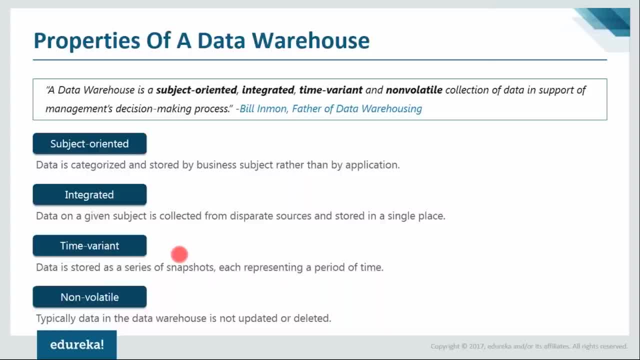 What is the progress that's been made, Or if it's not a progress, if it's the same, if your growth hasn't stagnated, then you can find out what are the metrics, what are the reasons why that has happened. You can find all these things. 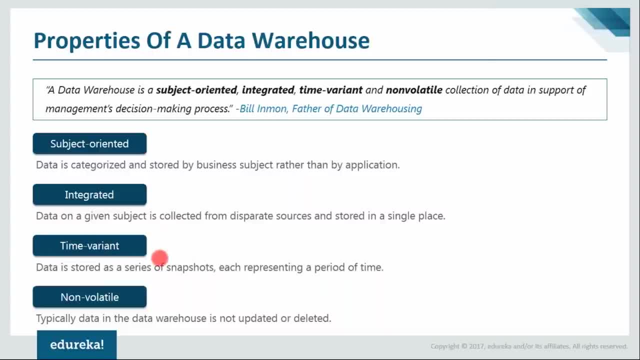 and you can look at all those details from a time approach, right from a time-variant approach. So that's what a data warehouse the advantage here is okay, That's one of the properties and the advantages that you have, And then data is non-volatile. 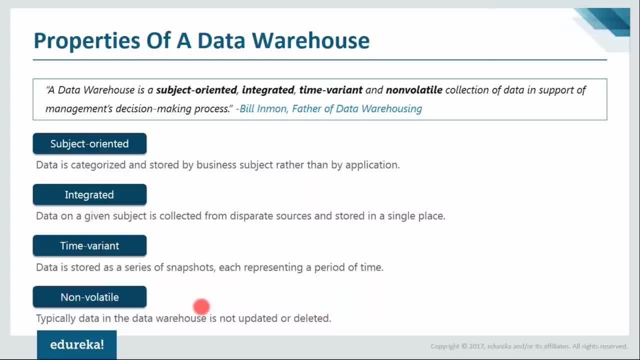 The data in a data warehouse is not updated or deleted. So this is what is the other property that I mentioned earlier: Once a data comes into a data warehouse, it cannot be deleted, or neither can it be changed. In fact, it can be updated. 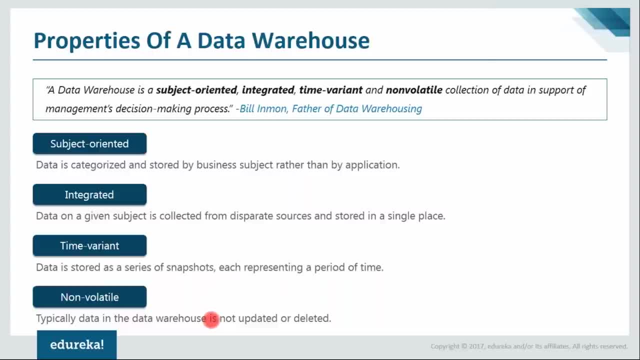 but the process of having to update it is a little complicated, okay, But of course it can be updated and deleted, So that's the thing. But it's highly recommended not to update, okay, So that's the advantage with the data warehouse. 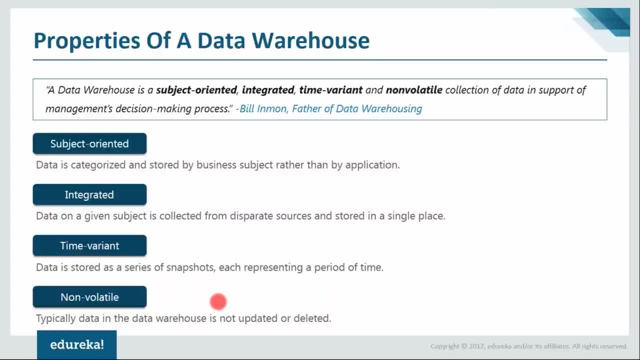 And since it will not be changed, there's no question of it getting corrupted, and that's why doing analysis and all these things are a better option. Now, getting back to the first point, we've said that it is subject-oriented, right. 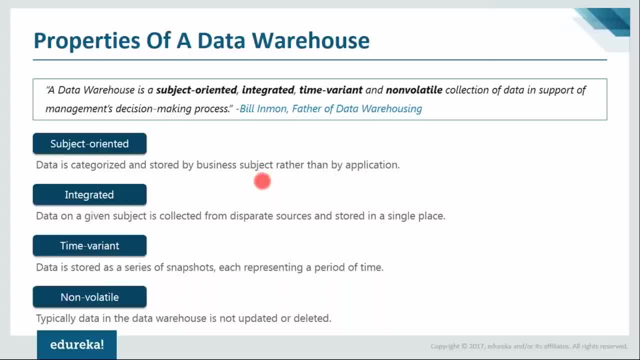 Data is categorized and stored by business subject rather than by the application. Now, what this means is the data here will be stored, or the data that you retrieve from a data warehouse right. You will get it in the form that you want it to. 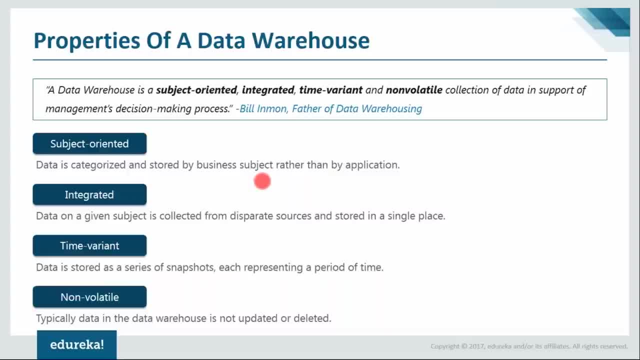 Now, if you want to give me an example of that, let's say that we are dealing with a retail company And in my retail company I have a marketing team, I have a sales team and I have an operations team And my sales team kind of keeps track. 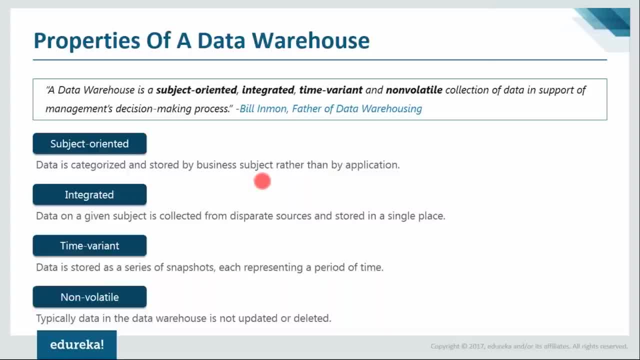 of all the sales that happens over a period of time, Okay, let's say the last one month. whatever sales they have done, they have stored all those details And then you have your operations team, which will make sure there is a smooth running. 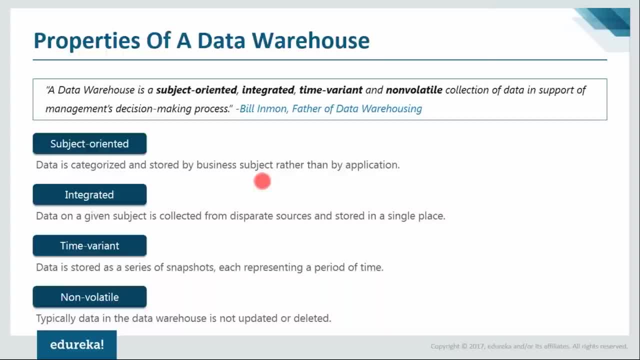 of all the process. Once a sale is done, there are various other activities involved, right, Like shipping the product and all these things- shipping and coordinating the transferring activities and all these things- And then your marketing team is- someone is probably that team- which would take care of your sales. 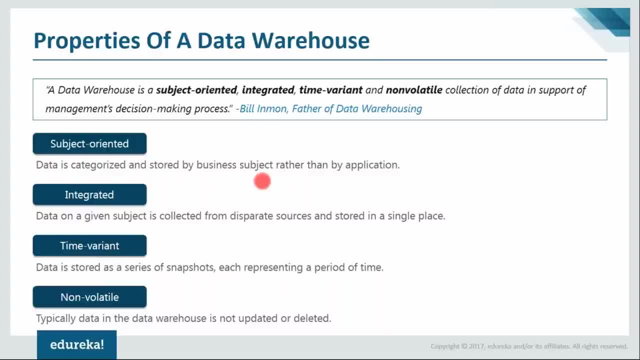 which would ensure that the right leads come in, to ensure that the right people get the right kind of service, And it's all about acquiring more such sales right. So your marketing team is on top of the funnel and they do all these things. 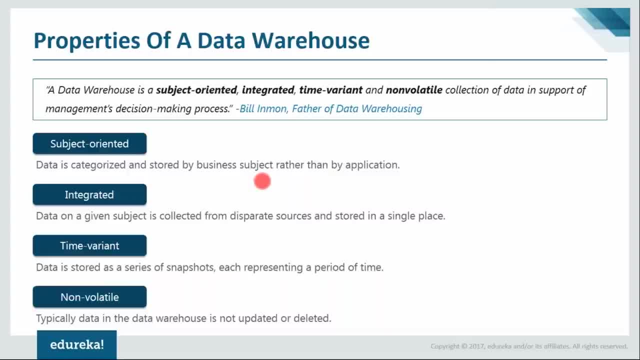 Now, if you want to integrate all these details, if you want one single view of them and you want to find details such that in this particular month, what was your sales And what was the kind of operations that was done right, 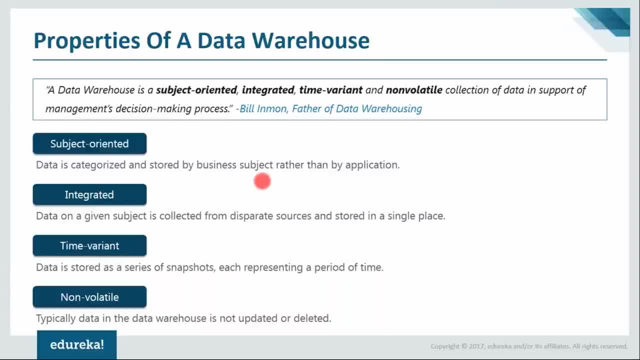 What kind of service was given to those customers And from how they became our customers. So when we the question of how they became something related to marketing. So if you have a question like this, where three factors are involved, Then at that point of time, 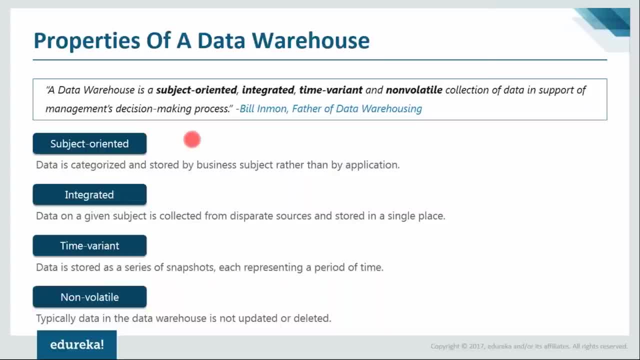 it's your data warehouse which comes to the rescue, Because when your question is related to this particular time and these three different metrics- sales, marketing and operations- then all these things can be integrated and you can get one single view from your data warehouse. 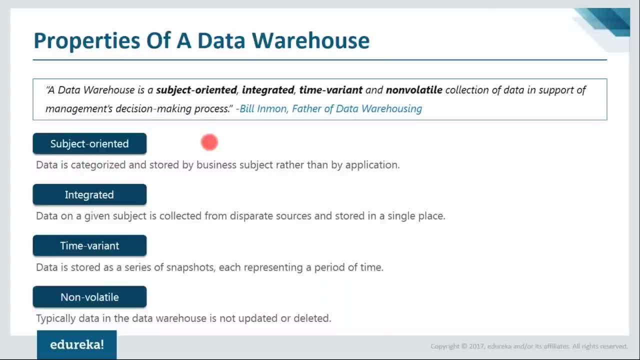 This is what a database lacks, correct. So integrating all your different data sources and storing them together and making them ready for anytime access is the biggest advantage and the most important property of a data warehouse. So if you guys had any problem in the previous slides, 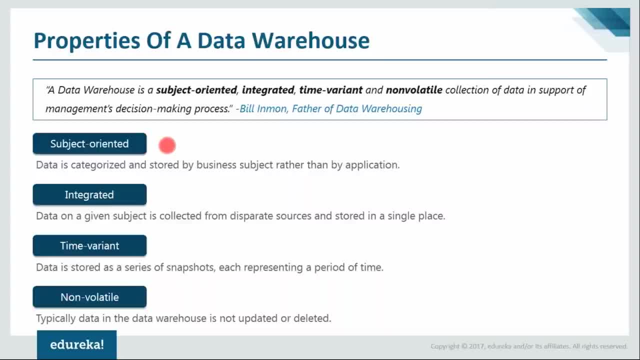 then I'm pretty sure this is something you have really understood after this slide, Because this is probably the epitome of data warehouse right. These three properties. if you understand these four properties, then you're pretty much ready to understand the next part. 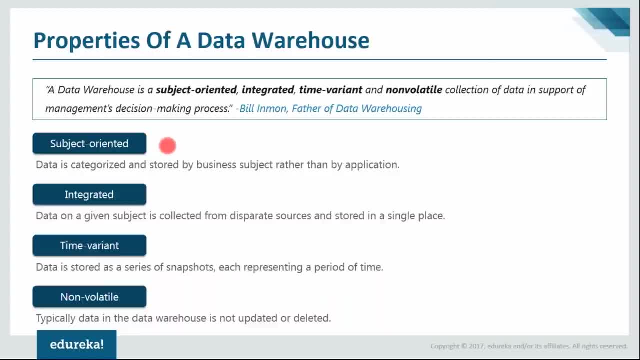 the next, you're ready to go to the next step in data warehousing right? So by now you should have understood how important all this is, Why I know how important business intelligence is and what kind of role this data warehouse plays. 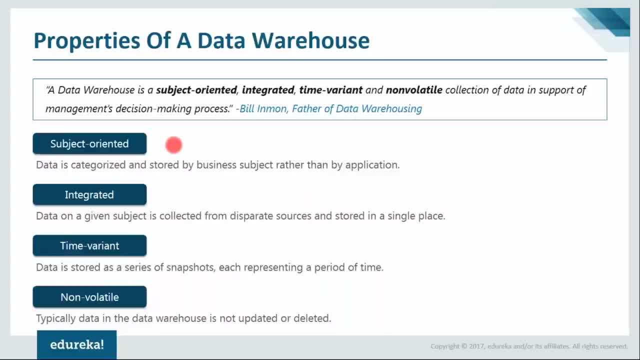 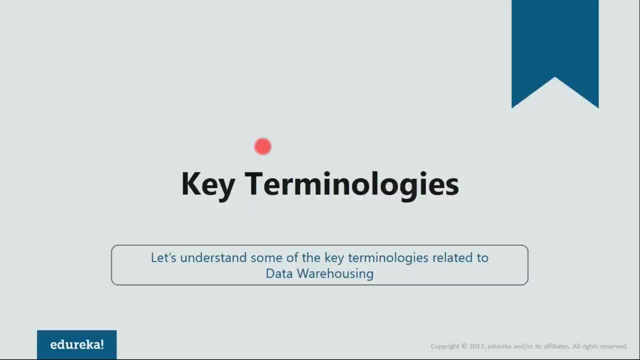 You can just think of how humongous a deal a data warehouse is correct, Yeah, So a couple of people are satisfied with that. So now that we've spoken about the properties, let's go to the next slide, and okay, Now we have to talk about key terminologies. okay. 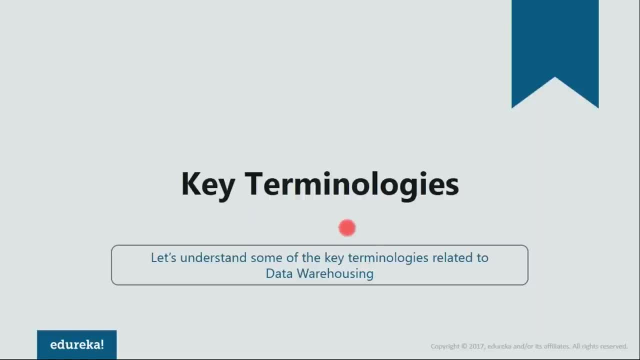 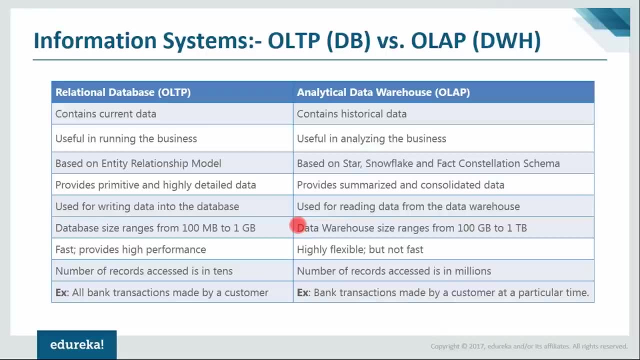 So right now we've understood data warehousing from a higher level. okay, Now let's dig deep, let's go to more basics here. okay, Let's understand the key terminologies that are related and that are involved in a data warehousing. 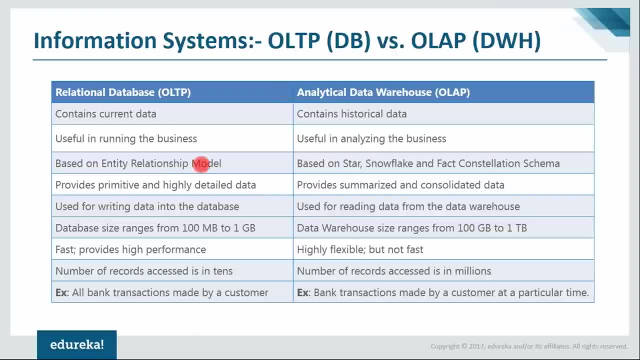 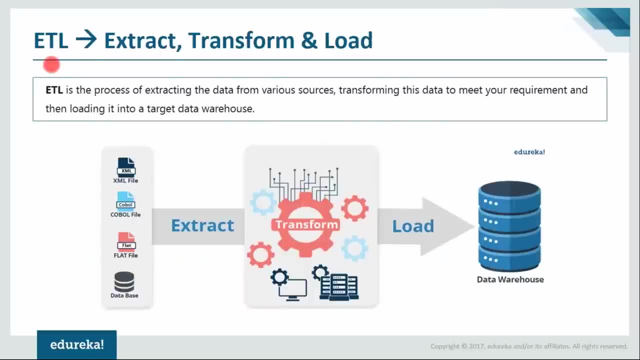 So first of all, we have OLTP and OLAP. okay. Now there are four things. I will talk about The differences between OLTP and OLAP, okay. Then I'll talk about EDL, I'll talk about data mart and then finally, about metadata- okay. 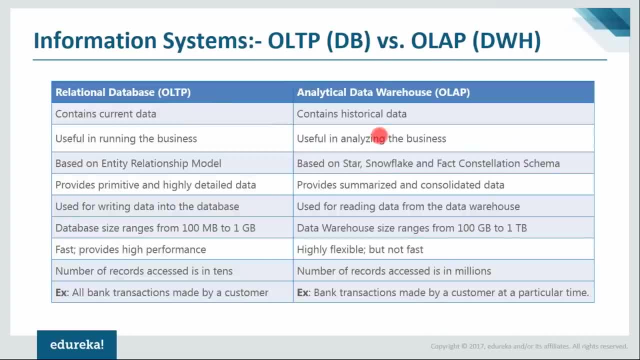 So let me go to the first topic, that is, OLTP versus OLAP. okay, So, in this part, which is OLTP, OLTP stands for online transaction processing. okay, Now, this is something that is a representation of that of a database. 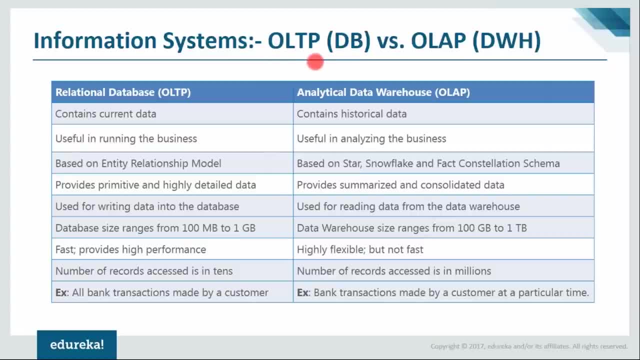 If you're running any kind of queries on your database, then that's called online transaction processing. okay, And then OLAP stands for online analytical processing, and this is the property of a data warehouse. So any kind of query or any kind of analysis. 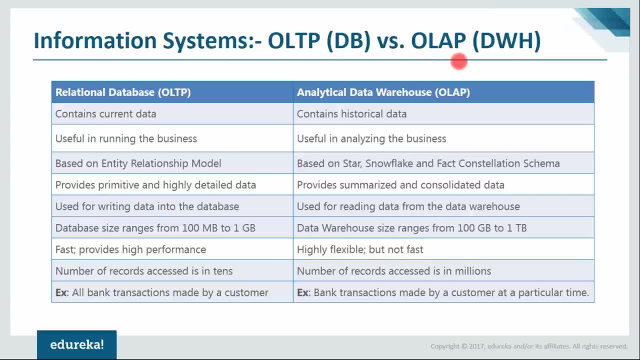 that you run on your data warehouse. that's called as an OLAP activity, correct? So let's go to the differences between the two. So, first of all, any data that is stored in a relational database right In an which involves OLTP. 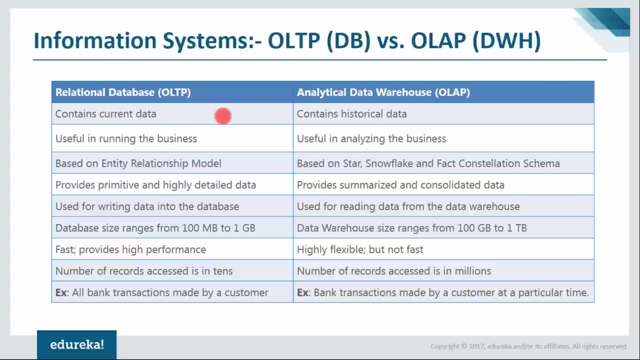 that contains the current data as well as past data. okay, Current data as well as past data, but with respect to a data warehouse and while performing an OLAP, you will be dealing with only historical data here. okay, It contains only historical data. 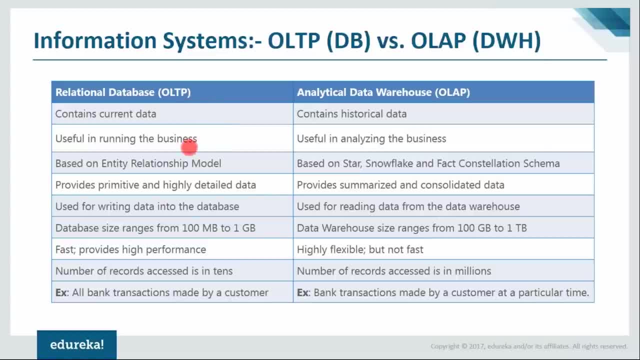 and the data that will be stored in your database. okay, When you use the OLTP, then those queries will be useful in running your business. okay, when you have to run your business, like if you want to store the data of the number of sales that has happened today. 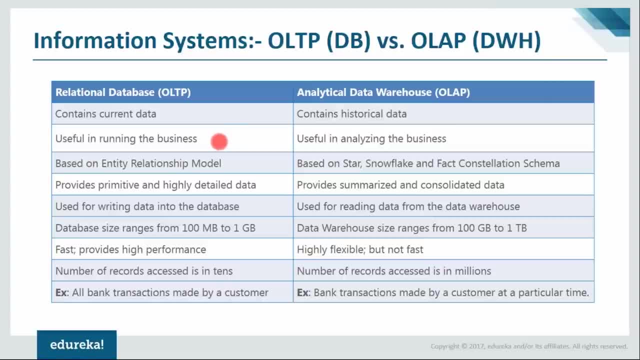 like every time a sales happens, then your records in your database has to be updated, right, So that's what we say. So when you update your record with the latest details of your customer, then that is what is the meaning of useful in running the business, okay. 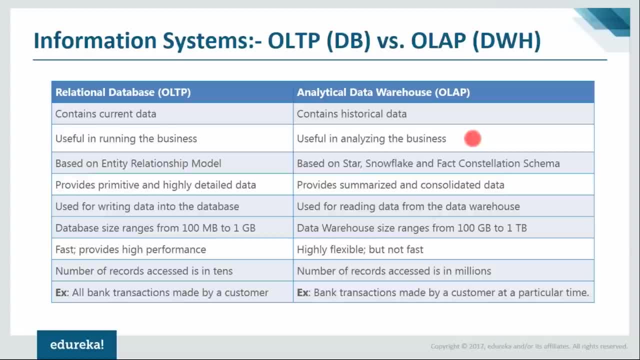 But an OLAP is something that is useful in analyzing the business. So here the kind of activity that you would do is that of finding out details like at what time how many customers bought the products, or at what time which customer bought which all products. 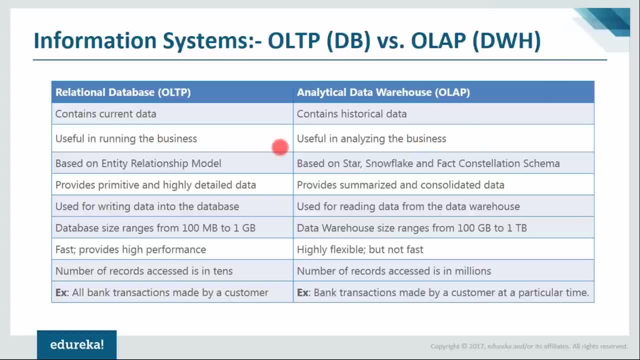 All these kind of questions will be answered with the help of OLAP. okay, And then the whole OLTP model of accessing data, of accessing or querying data on a data. it's based on the entity relationship model, okay, But whereas with the data warehouse, 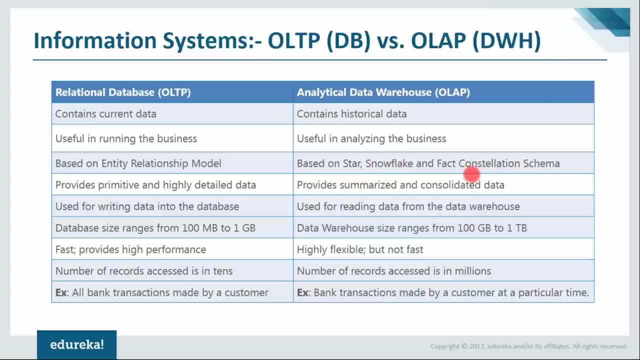 it's based on the star schema or the snowflake schema and the fact constellation schema. okay, So it's also called as the galaxy schema. So all these three things will come into picture, okay. And then your relational database. it provides a primitive and a highly detailed data. 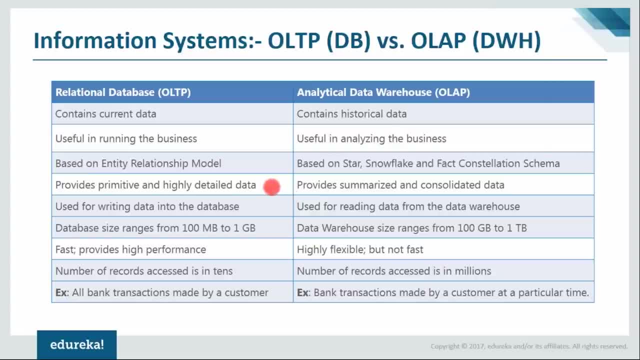 So, since you'll have one database, if you run one kind of a query like a select star from this particular table, then it would give you all the details that is stored right, So you cannot filter too many details with respect to the data that is stored in a database. okay, 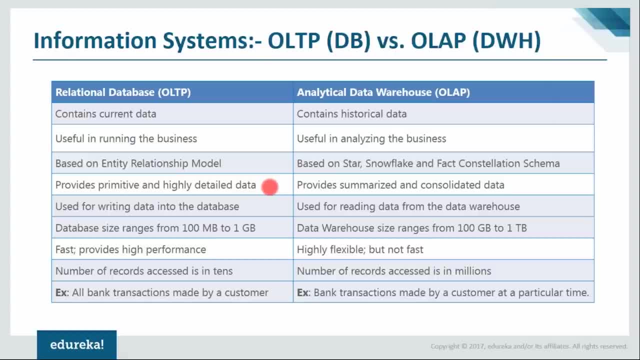 Of course you can, but the level of the filtering and analysis that you can do is not that much. So the data that you will get back from your query- right, The result that you will get back from your query- will be highly detailed, okay. 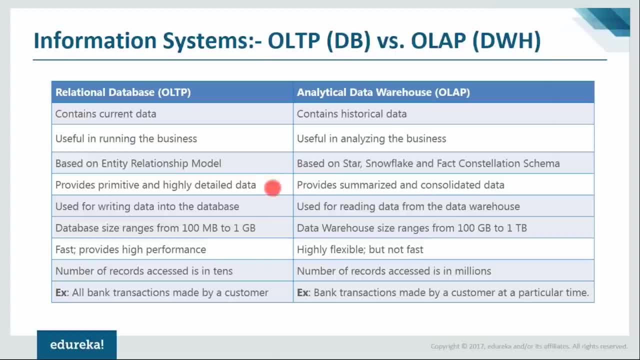 And it will not be exactly what you want, So it will not be that accurate. But whereas with the OLAP, when you do an OLAP on a data warehouse, it provides a summarize and the consolidated data It will point to you exactly what you want to look for. 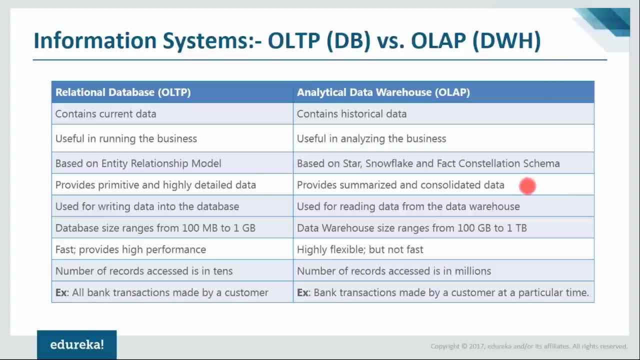 correct. So it's a very processed data and it points to one particular aspect which matters the most. So that's what this is. And then the OLTP: you use this for writing data into the database, okay, So, like I said, the same sales example. 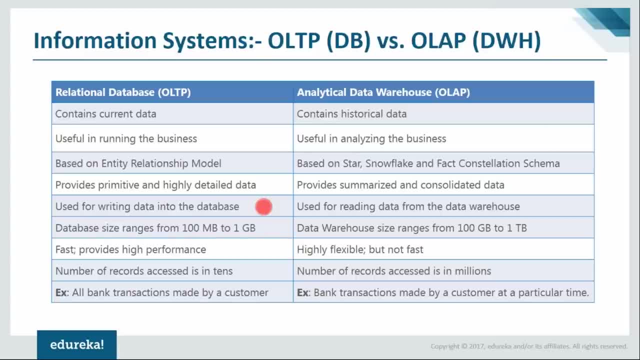 Whenever a new sales happens, your database has to be updated right With the new records of the product sold, of the customer who bought the product and all these things. So you basically use it for writing data into the database, But your data warehouse is primarily used. 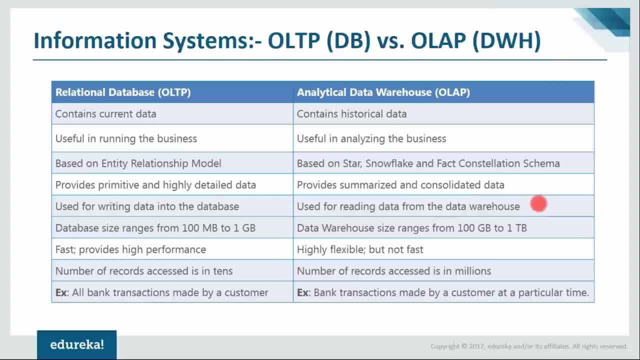 for reading data from the data warehouse. So writing to the data warehouse is something that is done so that you can do the reading from the data warehouse. okay, The primary concept here is to read the data from the data warehouse and to do the analysis. 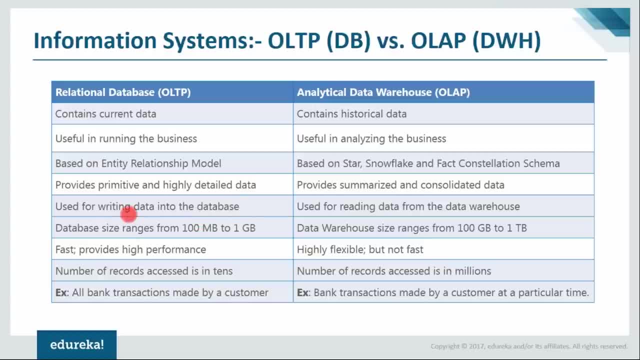 and all the visualization activities, But with the database it's more of writing the data into the database. all right. And the size. so, speaking of the size, a database's size would range anywhere between 100 MB to one GB. okay, 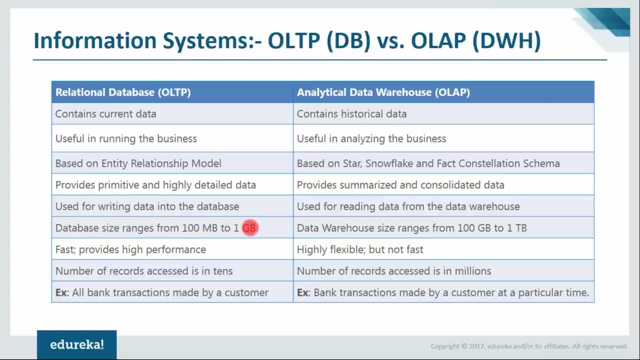 And this is also a very big number. 100 MB is a very less number, I would say, And one GB is also very less. So it would typically be much more than this, But compared to this range, if you look at a data warehouse, 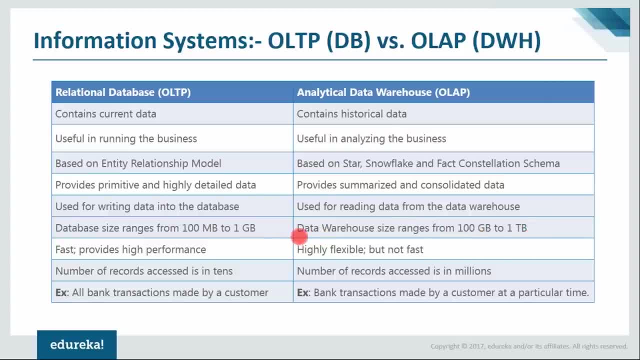 a data warehouse. size ranges from 100 GB to one TB, correct. So your data warehouse will have all the historic data and it will have all the relationships between the different data right, Such that you can do your analysis straight away. So, since it makes all the data more efficient and stuff, 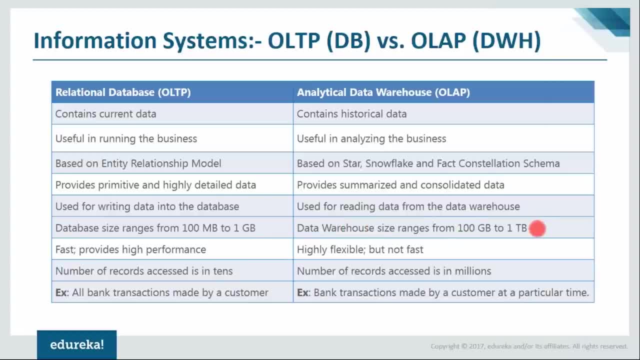 the data here. the size ranges from 100 GB to almost one TB. So that is what a data warehouse is And that's the part of a data warehouse. all right, And I can actually show you the difference between the two in today's demo session. okay, 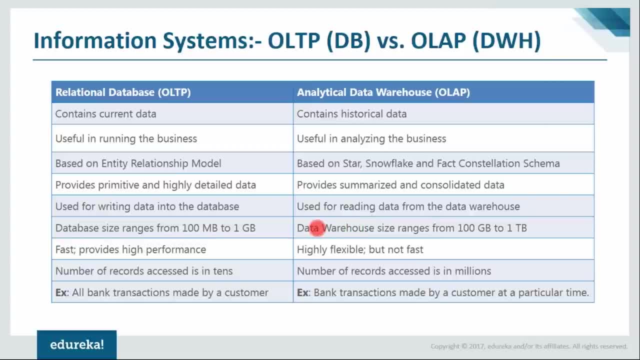 Later during the session I'll show you that The size of the source file that I have. I will show you the different sizes of the two files that I'll be using as a source And then, after they are processed, the data that I'll store in my data warehouse. 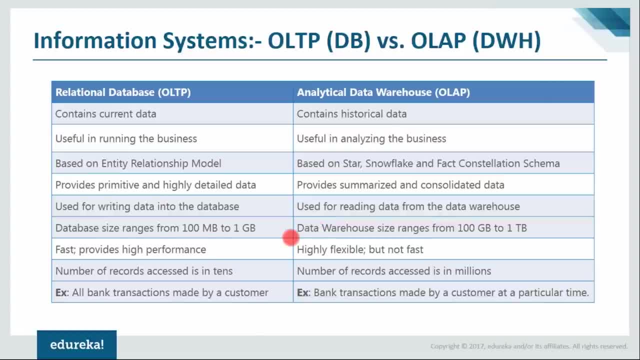 I'll show you what is the size of that data. So there'll be a big difference between the two. okay, And the data warehouse will be more than the database. I will show you that aspect later. all right, So that's about this point. 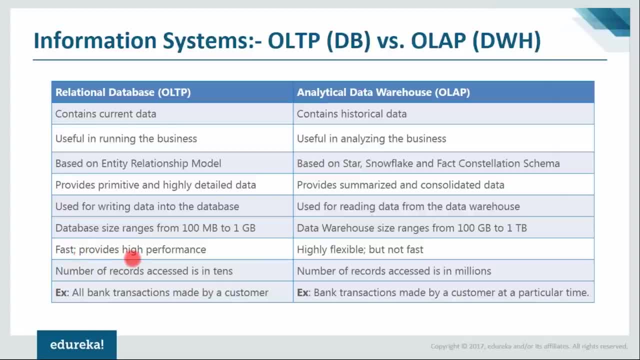 And then, yeah, Of course this will be fast. okay, Database is fast and it provides high performance. all right, So your data warehouse. of course it's not as fast as your database, but it's highly flexible. 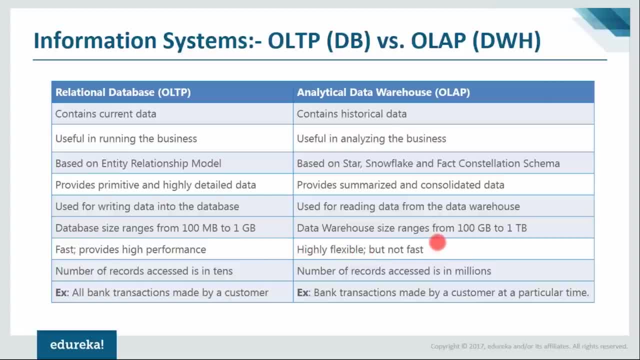 It's highly flexible because it gives you different views, So you have something called as the OLAP cube, right? So using the OLAP cube, you can get the. you can look at insights from different angles, different perspectives and different views. 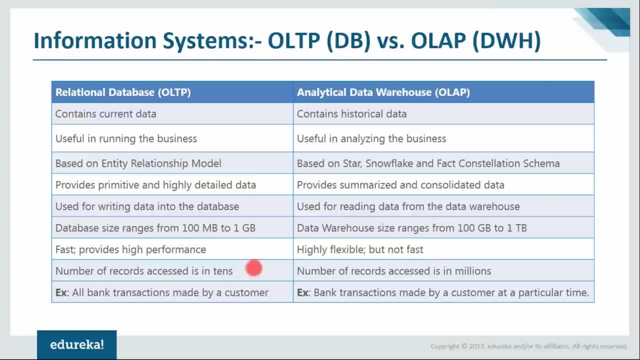 of data you will get. So that is the big advantage here. okay, And the number of records that is accessed. it is intense, But whereas with the data warehouse the number of records accessed is in millions, all right, An example of this can be all the bank transactions. 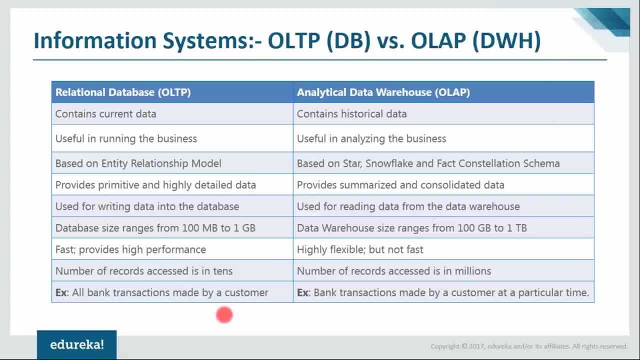 made by a particular customer. So if there is one customer and whatever transactions he's made, he will get all those. you know all those details right. So, supposing take the example of any email statement that you request for any email statement, 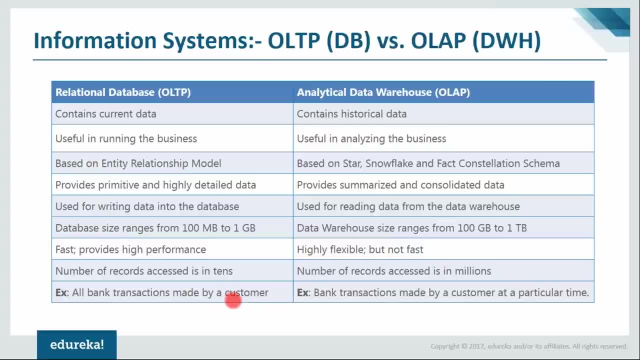 or a bank's account statement, all these things. So they are an example of OLTP. So whatever details are present in the database, those will be given to you, But whereas the bank transactions made by a customer at a particular time- okay, this is a more filtered 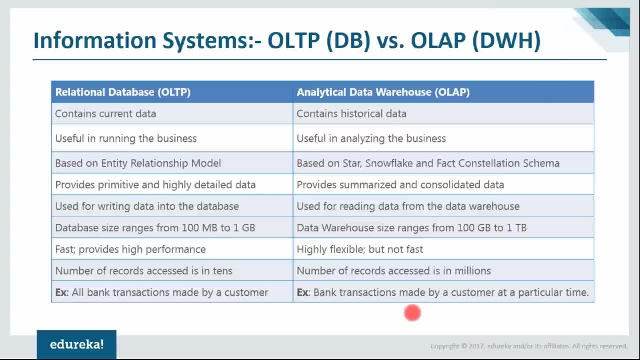 query and the answer also will be very accurate and point you to exactly that particular question. So that's what an OLAP is. So it's not gonna give you an overview here. it's gonna exactly point you to what you want. It's not very much in detail, but it's more accurate. 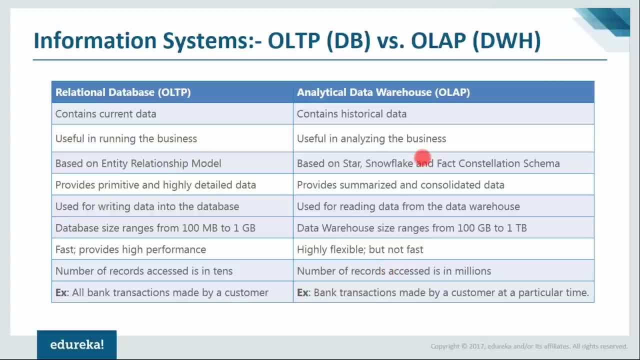 Correct. so that's what an OLAP is and that's the difference between OLTP and OLAP. okay, So these are two strategies that are used for accessing data. OLTP is used for accessing data in a database and OLAP is used for accessing that data. 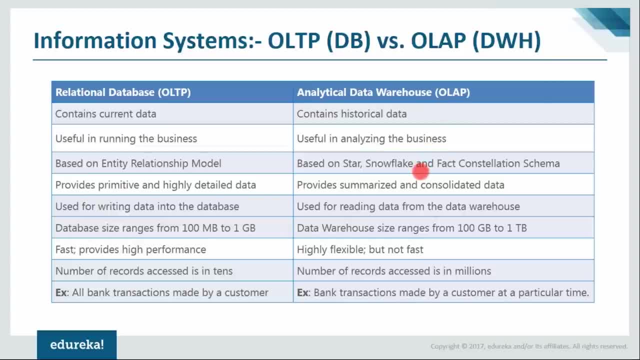 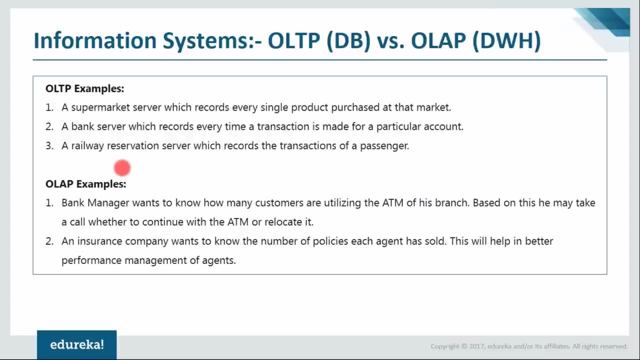 in a data warehouse, all right. So I hope even this slide is clear to everyone. All right guys? Okay, if you have any doubts, then that will be cleared by this slide. okay, Because the examples are there for both these strategies. 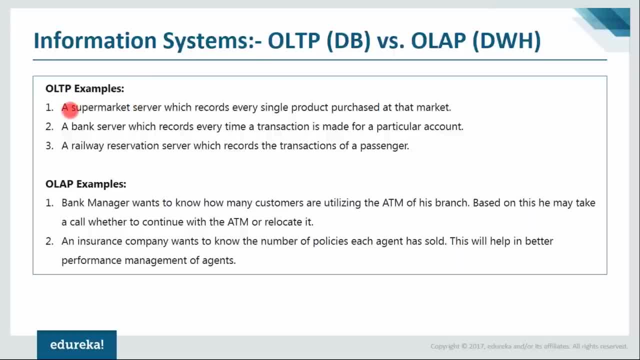 So if you want more examples of an OLTP, then one would be that of a supermarket server which records every single product purchased at that market. Okay, so every single product in their history, or probably in the last one month. all these things can be accessed using your OLTP, okay. 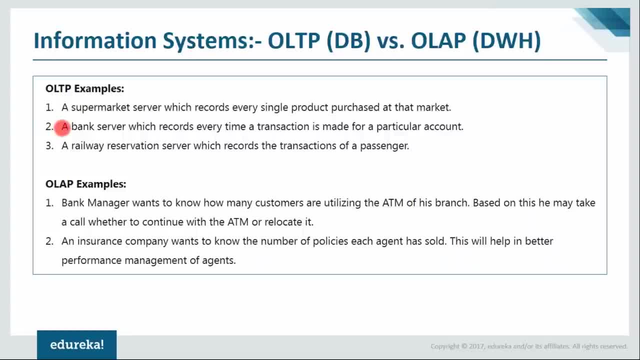 From your database, So you don't have options to do much of filtering here. And then another example is that of a bank server which records every time a transaction is made for a particular account. Okay, every time a transaction is made in a particular account. 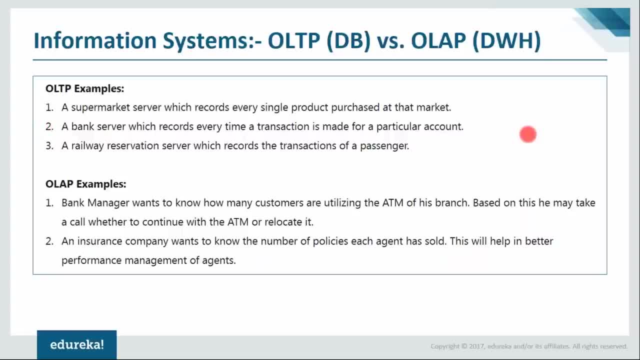 the data will be updated in that table and you can query that kind of data and you'll get that result. okay, Another example is that of a railway reservation server which records a transaction of a passenger, So whatever activities a passenger does, So all these things will be recorded. 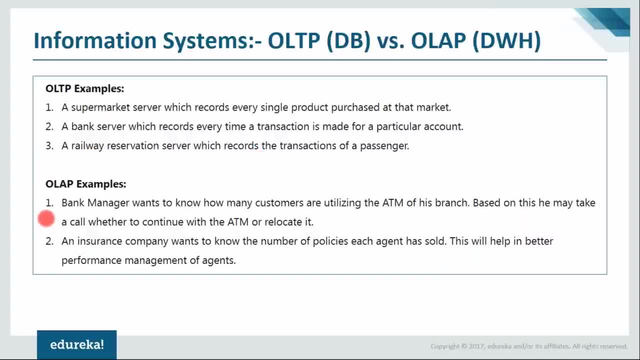 by the reservation server. all right, So this is one example. When you look at OLAP, they will be much more detailed, The queries here will be much more detailed and the answers will be much more accurate and very crisp. okay, So an example is that of a bank manager. 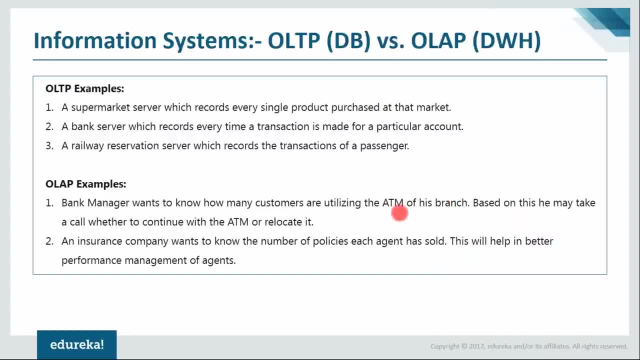 wants to know how many customers are utilizing the ATM of his branch. okay, Because maybe based on that, he may take a call whether to continue that ATM or relocate that ATM to a different place, right? So this guy, this bank manager, would want to. 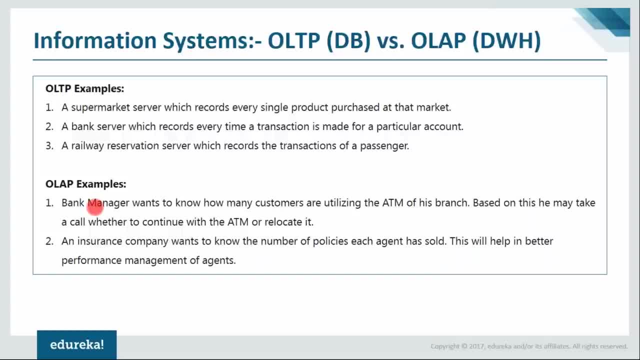 you know, first of all understand if there's any use in having the ATM in that place. Are people using it, correct? If people are using it, then how many people are using it? At what time are they using it? Or would it be better to have the ATM? 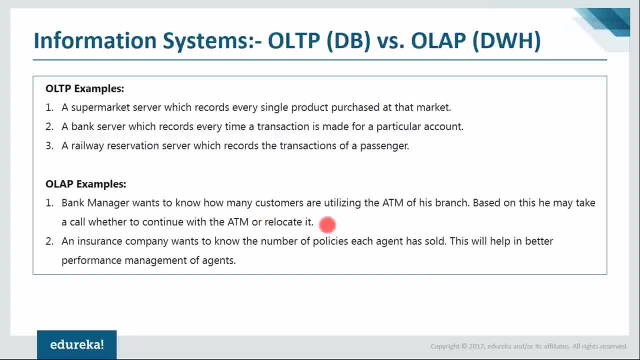 in a different location where it's much more easier for people to access it. So all these kind of questions will be answered. only if you have OLAP in place. okay, Only when you have a data warehouse in place, not with the database. 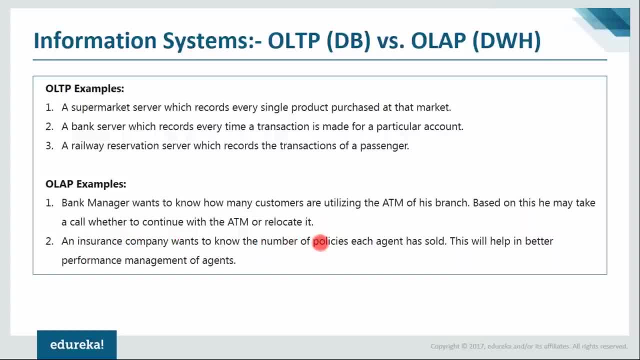 So another example is that of an insurance company that wants to know the number of policies each agent has sold. okay, This will help in better performance management of agents. So you'll have multiple agents in your company and you would want to know what happens, right. 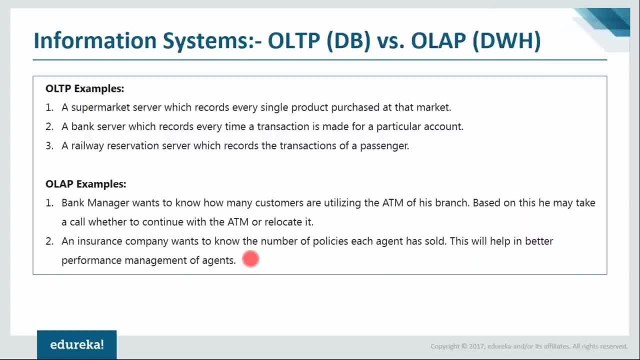 You know, you'd want to know who's the best-performing agent. you would want to know how they're performing. why is this person performing better? You can, you know, optimize each of their performances, So all these things can be done. 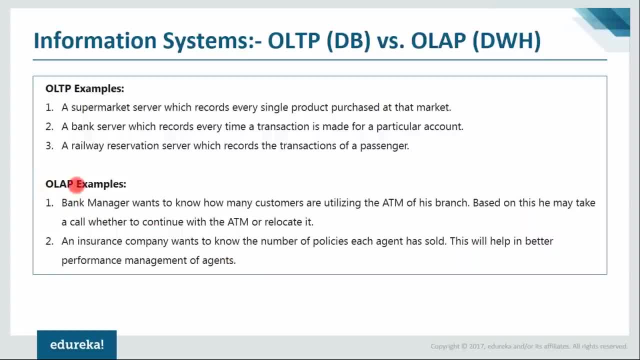 with the help of a data warehouse and they can be done with the help of OLAP right, The OLAP strategy, the OLAP activity that is done on a data warehouse. So that is the difference between the two right. So I hope you're getting the differences here, guys. 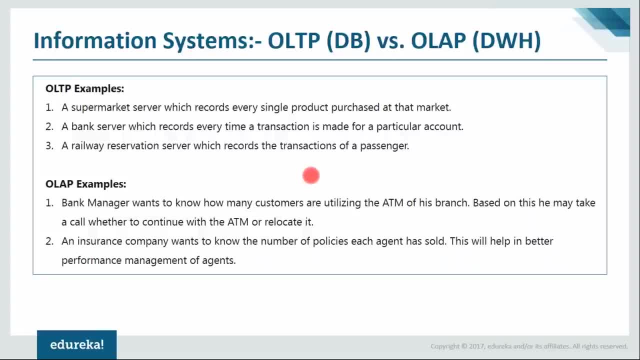 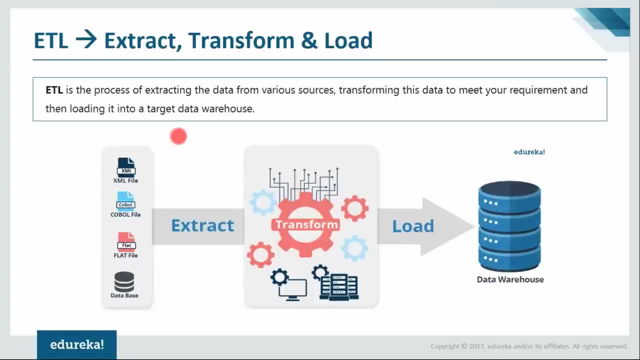 Right, OLAP and OLAP. Okay, since it's all clear, let me go to the next slide. Now, the second important terminology that we have with data warehouse is that of ETL: extract, transform and load. So by going by the definition, 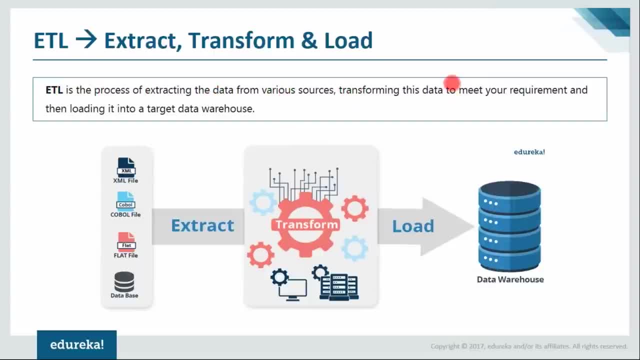 ETL is a process of extracting the data from various sources, transforming this data to meet your requirements and then loading the data into a target data warehouse. okay, You're extracting the data from here, right, You're extracting it and then you're transforming it. 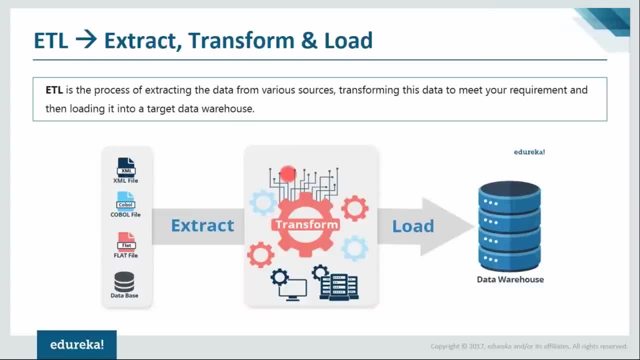 into the way you want, in a more readable fashion, in a more relatable fashion. Then, once that is done, you load that data into a data warehouse And the whole process of getting the data from here data source to your data warehouse. 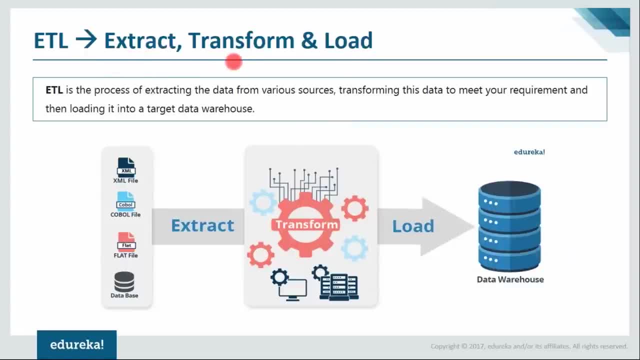 this is done by the ETL, the activities of extraction, extraction, transformation and loading. So we have popular tools for this very process. So you have tools like Talend, Informatica, you have Erwin, all these things, And Informatica and Talend are probably 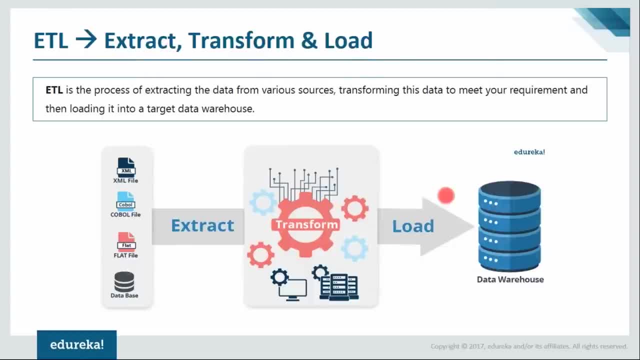 the most popular tools for this process, for extraction, transformation and loading data into a data warehouse right. So this is something that you should have understood by now. Any doubts, guys? Because I don't want to waste much time, I want to go to the next slide. 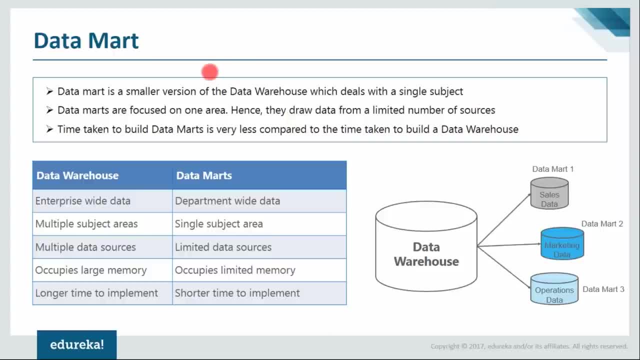 and teach the next concept, okay, Great. so the next one is data mart. okay, Now, if you've understood so far till ETL, then half your job is done, because data mart is something that's very close to a data warehouse. 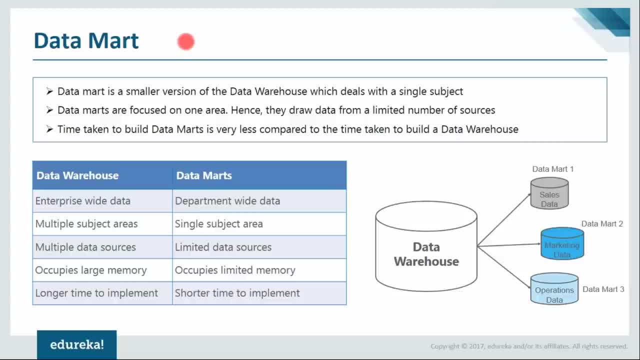 and you don't have that much of a difference when you compare it to a data warehouse. But the basic difference between the two is the data mart is just the same data warehouse itself, but a smaller version. okay, Let's look at the line, the definition here. 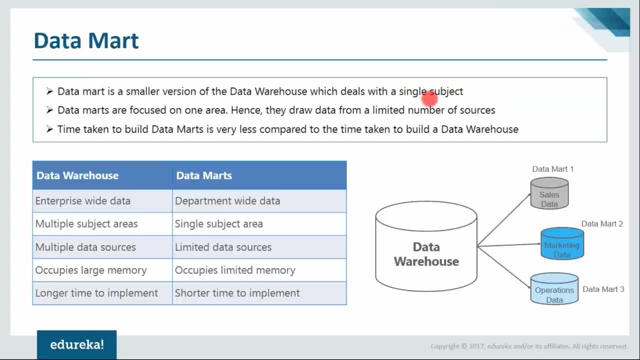 The data mart is a smaller version of the data warehouse which deals with a single subject. okay, The data marts are focused on one area, Hence they draw the data from limited number of sources. And the time taken to build the data marts. 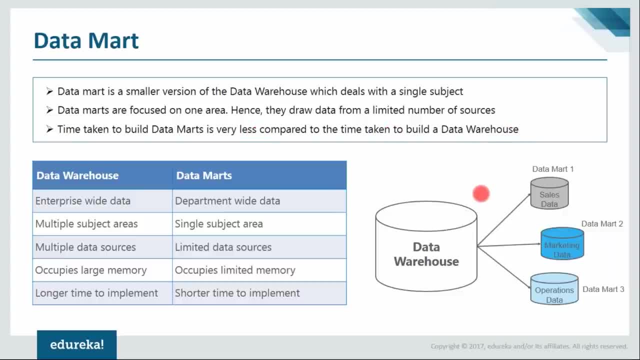 is very less compared to the time taken to build a data warehouse. Now to give you an example or an explanation of this: in your data warehouse you will have all your details, right, all your details that you have. So this itself is more refined, okay. 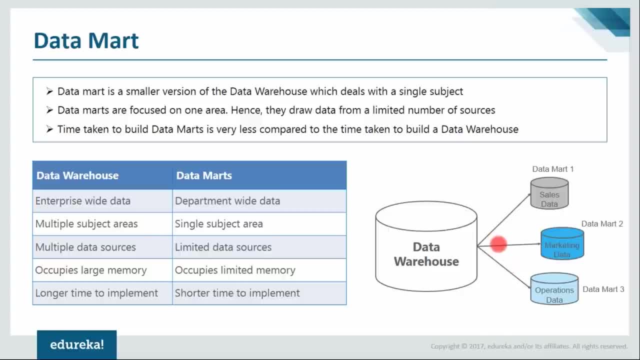 But your data marts are smaller than the smaller versions of that data warehouse which is used to satisfy only certain users. Supposing you have one particular user base, okay, That is your sales team or your sales manager who wants to use only your sales data. 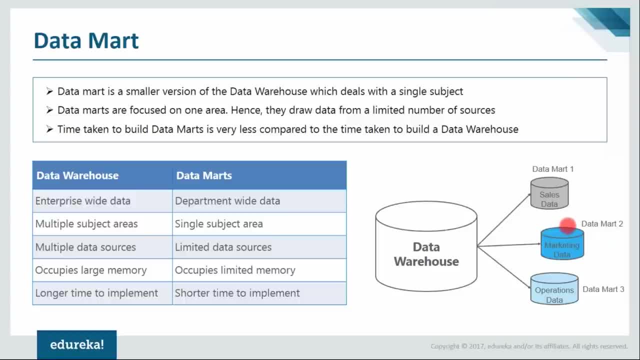 Then that can be done with the help of a data mart. And similarly, you have a marketing team who wants to access all the marketing data, Then that can be done by using a data mart. okay, And then again you have other operations team. 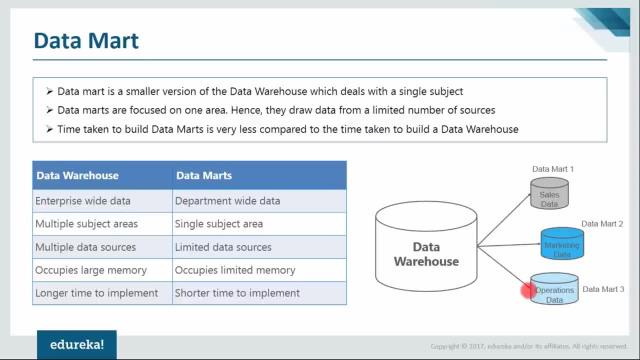 that wants to access the operations data, Then you can give them the access to that data by using a data mart separately. okay. Now the need for data mart is, first of all, your data warehouse will store all the data, okay. 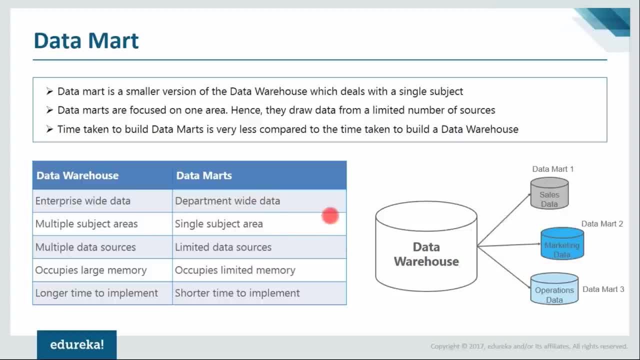 Your sales data, marketing data, operations data- So all the data coming from different data sources, So you'll have multiple data sources, right. All that will be stored in one single place And from here this will again act like separate data sources, right. 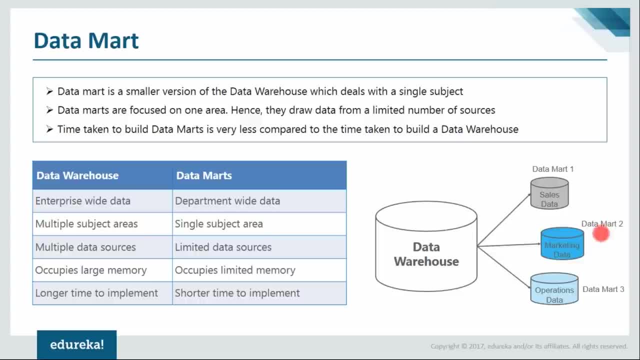 So, for the sales team, this will act as a data source. For a marketing team, this will act as a data source, And then for the operations team, this mart will act as a data source. Now answering the question as to why we need them. 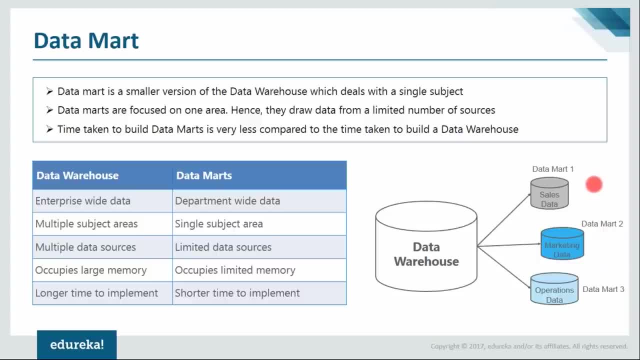 it's to probably give more security, to enable more security and integrity, Because, since all your data will be there in your data warehouse and if you let your entire company access the data warehouse, they'll get access to all the details and all the work that is done by other teams. okay, 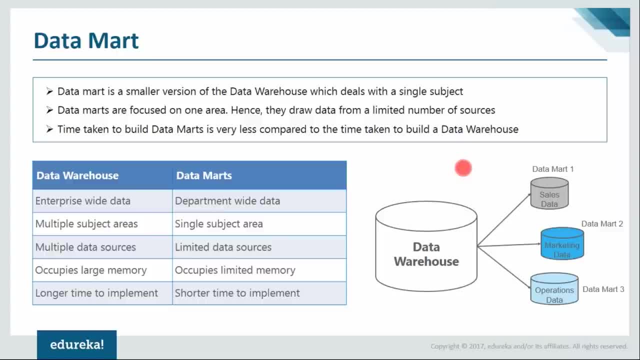 So there might be multiple teams and there'll be multiple strategies which you might not want to reveal to other teams. So at that kind of a time you can divide your data warehouse such that only this particular user- okay, your sales user, or a particular user base. 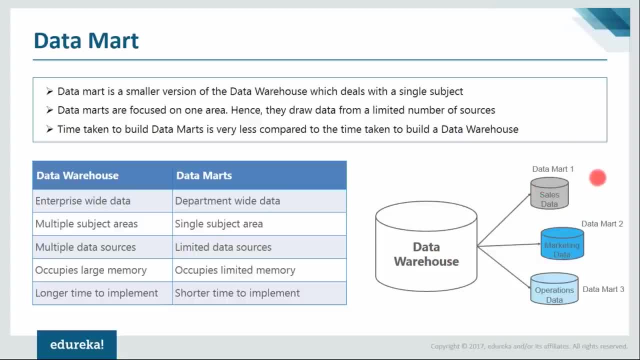 gets access to only certain data from your data warehouse. So at that kind of a time a data mart is useful. Or you can have a second data mart for only another set of user base, For example your marketing users, So they will get access to only the marketing data. 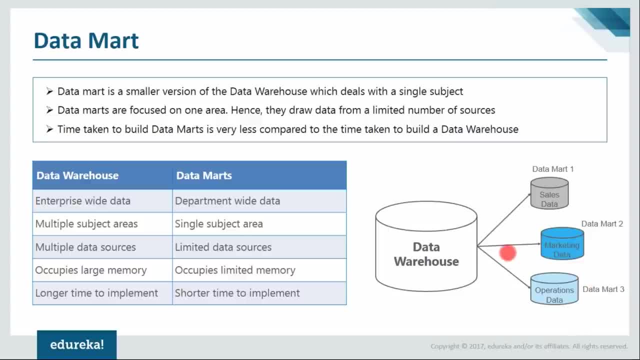 from your data warehouse right And then your operations data Similarly, which can be accessed only by your operations folks. So that's the different advantages that you have. since the data is all divided, It's all stored separately. Different people have access to different parts of your data. 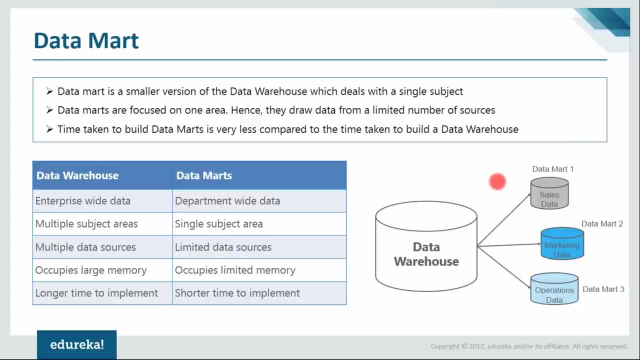 Different parts of your data warehouse. So this probably brings more advantages right? So that's the data mart, And that's why I told you that. you know, if you've understood so far till ETL, then half your job is done. 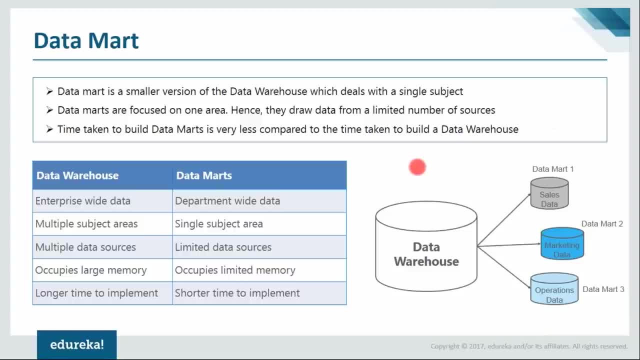 But data mart is something that extends the functionality for data warehouse right. So that is the thing. And speaking of the differences that is there in this table, the data warehouse will store the enterprise-wide data right, The enterprise or the enterprise-wide data. 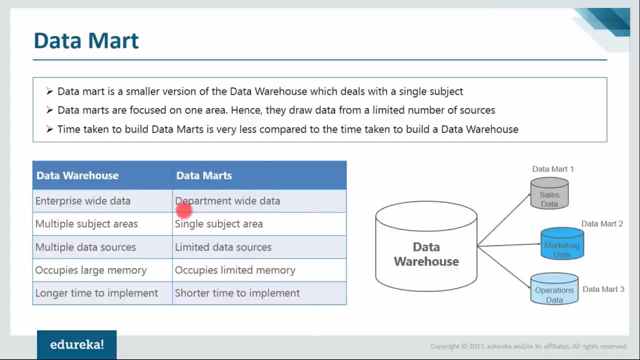 Whereas data marts will store only departments-wise data. There'll be multiple departments in the whole company, in the enterprise, and they will store department-wide data And then the data warehouse. it'll have multiple subject areas- okay, But a data mart will have a single subject area. 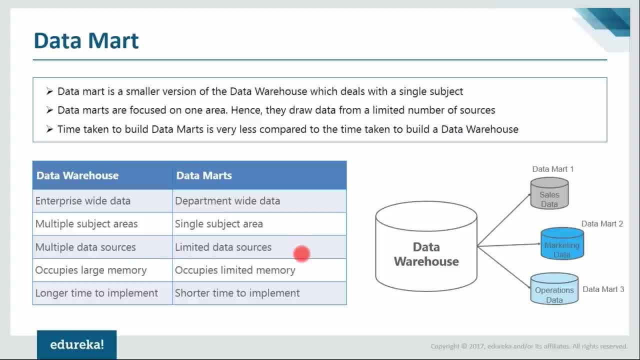 There'll be multiple data sources in case of a data warehouse, okay, But in case of a data mart, there'll be limited data sources. In fact, there can be just one data warehouse, right. This will act as a source to your data mart. 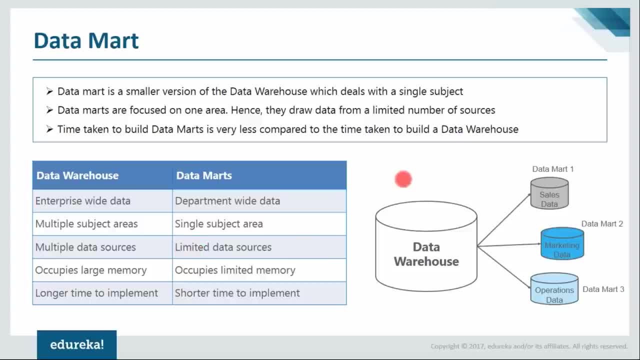 But, however, we have said limited here, because not always do you need a data warehouse. There are also instances where your data source itself acts as an input to data mart. Okay, Now, that is something that you will understand in the next slide. okay. 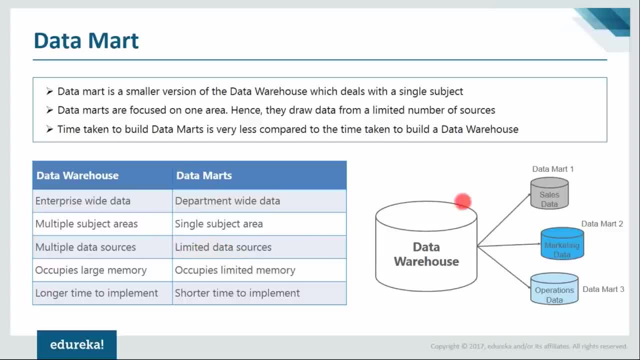 So just don't get confused: when we say that limited data sources, It doesn't mean this is the only source. They can also come from a data, a proper data source like a flat file, or from a database and all these things, all right. 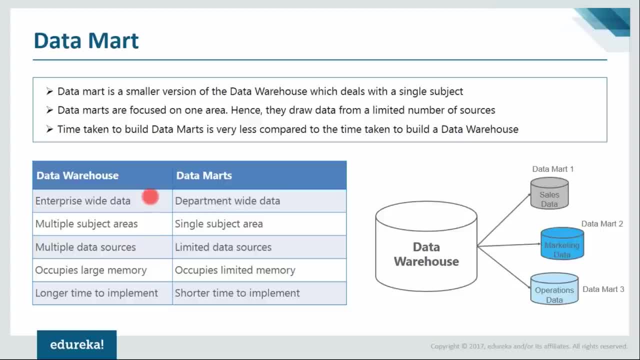 And then a data warehouse. it occupies a large memory. This, of course, because there's a lot of data. Enterprise-wide data will be stored here. Multiple subject areas will be there. Because of that, there's larger data here at stake. 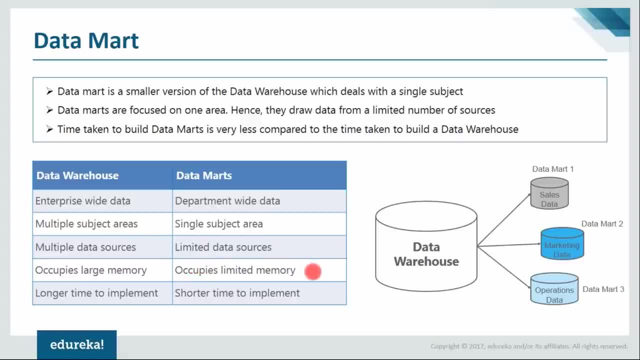 and that's why there's greater memory. that's occupied, okay, But in case of your data mart, it occupies limited memory because it's very crisp and limited to only a particular department, okay. And then the other thing is: data warehouses takes longer time to implement. 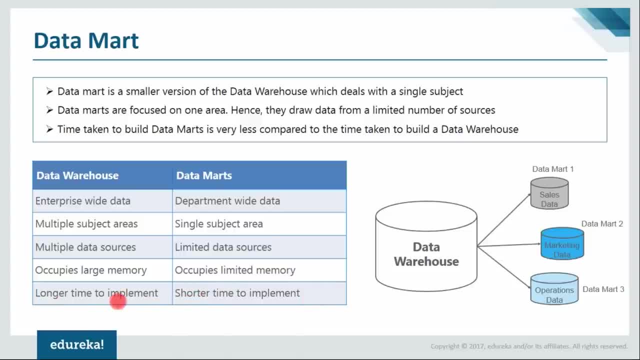 but a data mart takes very short time to implement Because once you have all your data warehouses stuff in place, you can easily divide them by just creating different data marts. okay, So the tough part is your data warehouse. So once you've got your data warehouse sorted, 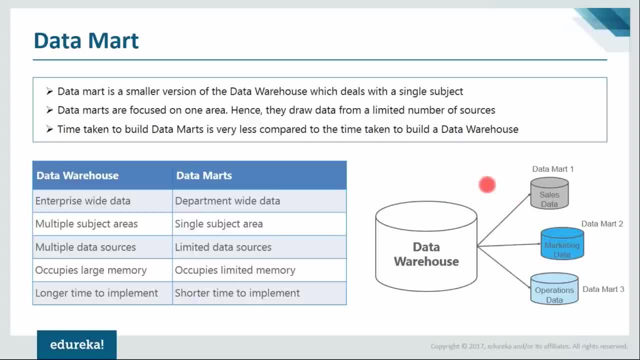 you can easily form your data marts. In fact, there's even the other way. There's also practices where you first build your data marts and once you've done that, after that you create one single repository, and that's when you create a data warehouse. 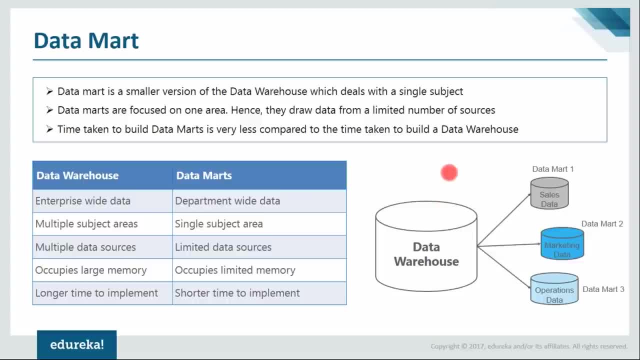 So there's also two approaches here. One is the top-bottom approach and the other one is bottom-up approach. So those are the two things, and I'll go into details about these two approaches in my next session. okay, Of course I can't do it today. 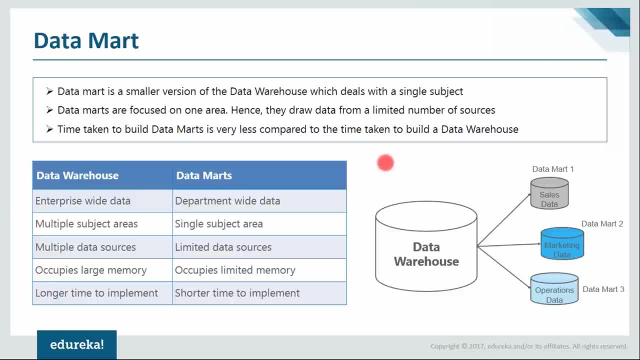 because we have very limited time. all right, So moving on to the next slide. Okay, now, speaking of the different types of data, marts- okay, this is what I was talking about. I was talking about it in the previous slide. 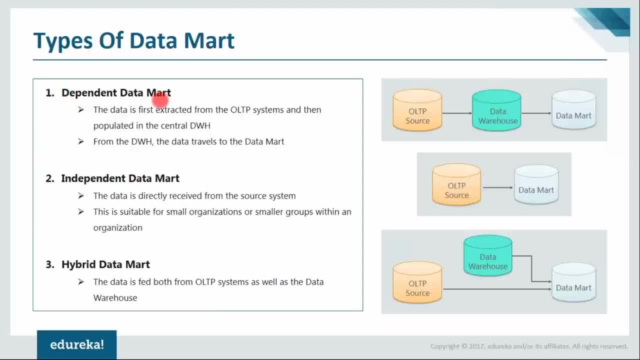 So you have three different types. One is a dependent data mart, The other one is independent data mart. The third one is hybrid data mart. Your dependent data mart is the data is first extracted from the OLTP systems and then populated in the central data warehouse. 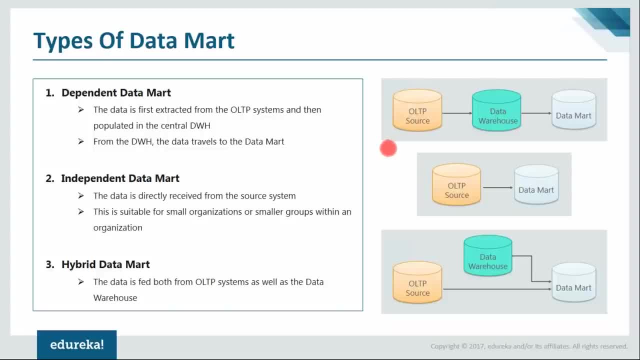 and then from this data warehouse the data travels to the data mart. So look at this example. okay, This is the standard practice or the default approach. where you have an OLTP source, then you get that data into a data warehouse and then from the data warehouse 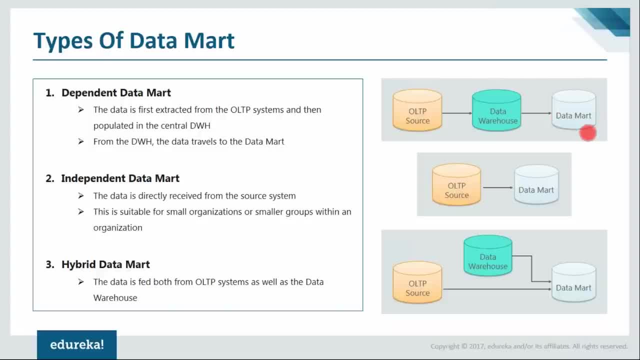 you get a data mart. okay, You'll have multiple data marts where each different mart will have particular data from the entire data warehouse. okay, This is the first regular approach. and then you have the independent data mart, which is a slight variation compared to dependent. 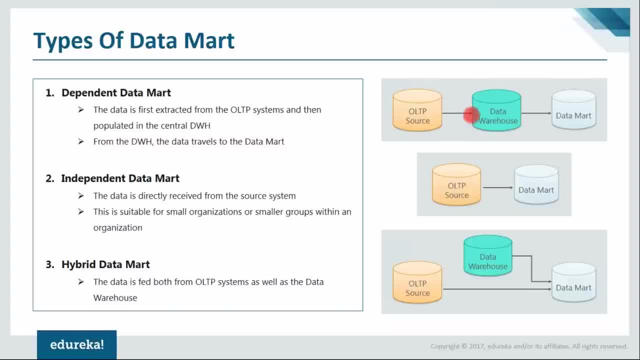 So here the data is directly received from the source system. okay, You don't have a data warehouse in place over here. That is what this line means, and this is suitable for small organizations or smaller groups within an organization, So basically an organization which is very small. 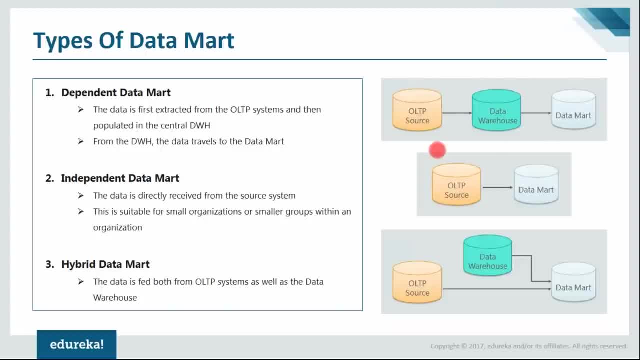 it might not need to go through of creating a data warehouse and stuff, So they can just have an OLTP source and from there they can just get the data onto a data mart and they can use it for various purposes. Okay, 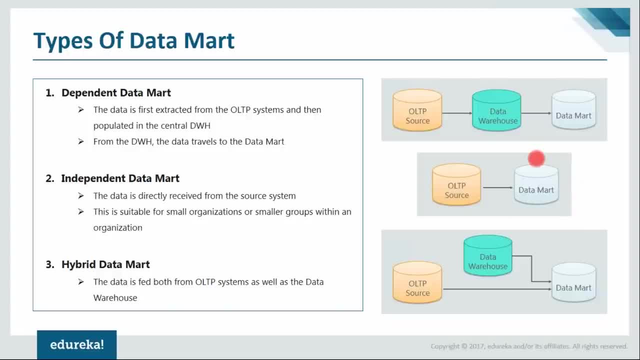 That's what we have an independent data mart for. So that's the difference. It just does not involve a major data warehouse, So directly the data goes to a data mart. In fact, you'll have multiple data marts over here. 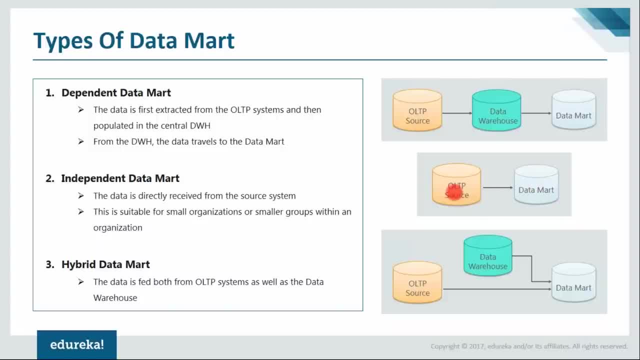 You'll have data mart one, data mart two and stuff okay, Which will be coming directly from the OLTP source, And then you have a third type, which is the hybrid data mart. So, by definition, you might know what this is right. 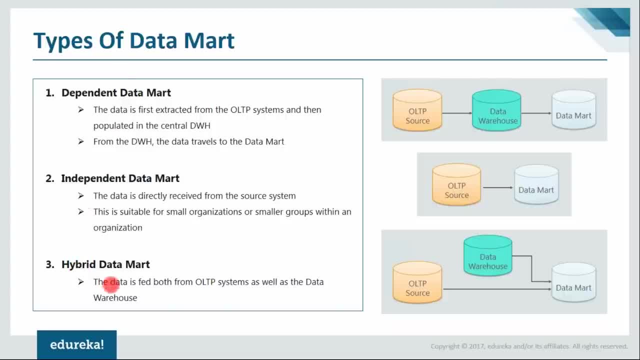 By the name of The name itself is pretty obvious. It's a combination of these two. The data here is fed from both the OLTP systems as well as the data warehouse. Okay, so look at this example for that instance, The data here it's coming from the OLTP source. 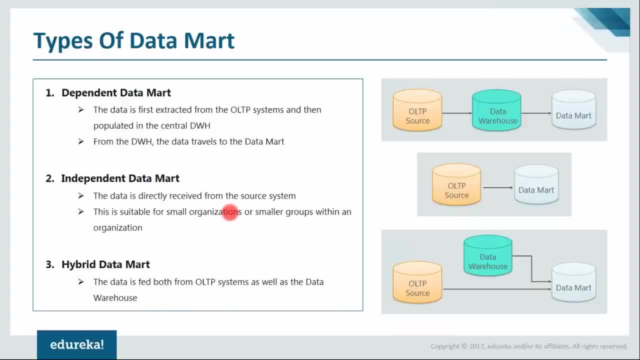 as well as from a data warehouse. So this is what the hybrid data mart is And, depending on your company, depending on the size of your company, the requirements of your company or your organization, you can choose one of these. You can model your entire database and data warehouse. 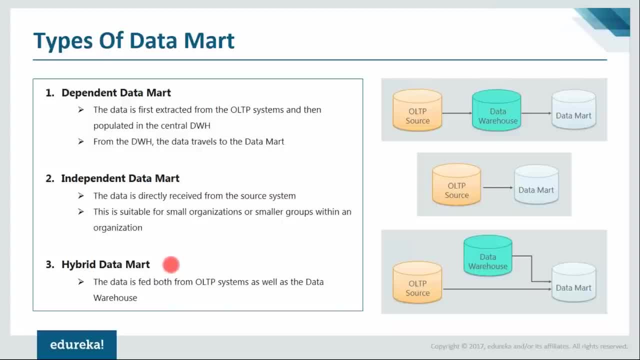 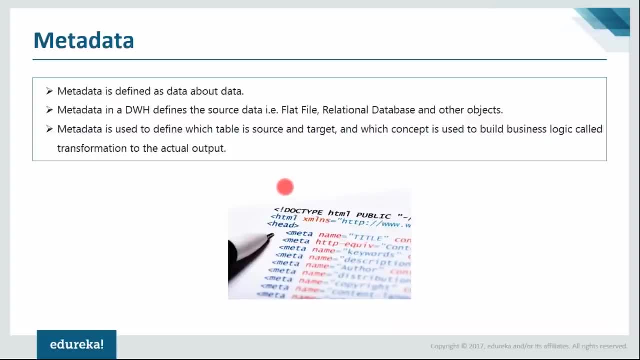 in any one of these models, Either the dependent or the independent data mart or hybrid data mart. all right, So that's about the different types of data mart. So, moving on to the next slide, we have something called as metadata. Now, people here from programming background. 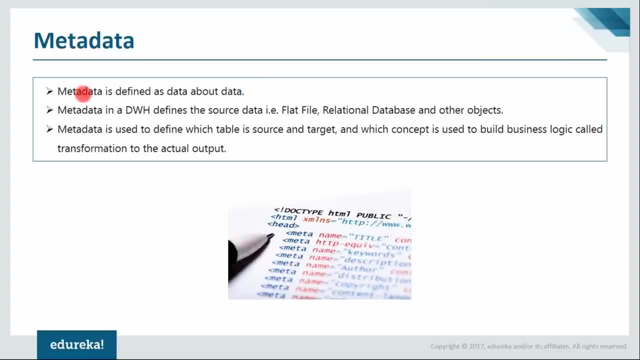 or from the technology background, you might all be aware of what a metadata is. Metadata basically is defined as data about data. okay, It contains data about where your actual data is stored. Supposing you have your raw data right, Where is that data stored? 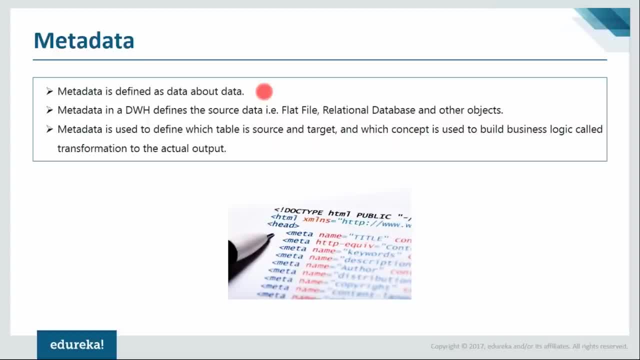 What is the size of that data? So these are the answers to these kind of questions- is what will be present in your metadata? Your metadata will contain the location of your actual data. It will contain the size of your actual data. It will contain details like which was the source? 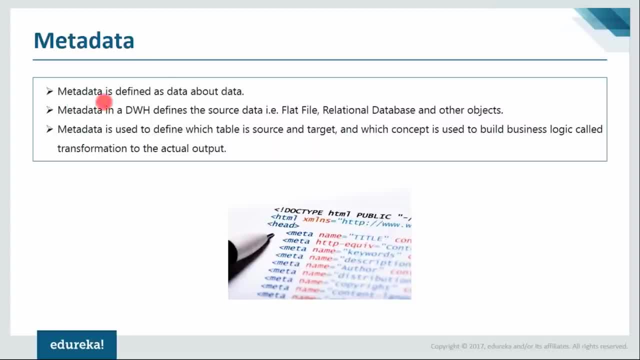 it came from and when was it created. All these details will be stored in your metadata right. So that's what metadata is. So that's how different metadata is from regular data And metadata specifically in a data warehouse. it defines the source data. 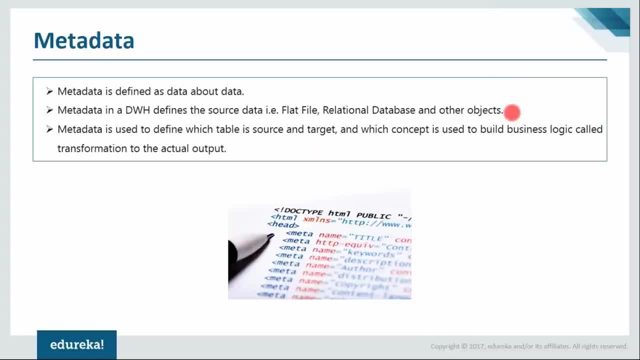 There is a flat file, There is a file, relational database and other objects. So the reason that we give so much importance to metadata in a data warehouse is because- take the example of any company that's having a 24-7 business. okay. 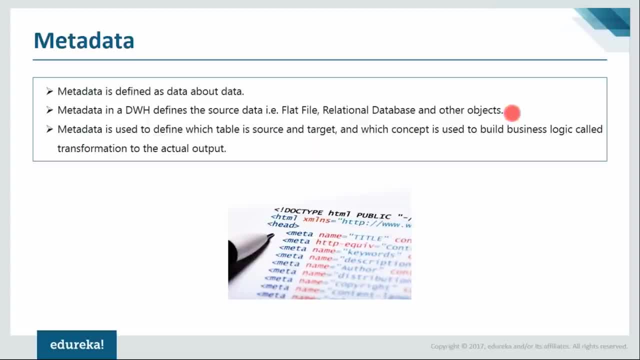 They have a rolling sales team that works throughout the clock, The 24-7,. they have sales coming in. Data will be going into your database. okay, Now, in this case, you cannot always keep adding data into your data warehouse, because you know that data warehouse is not real time. 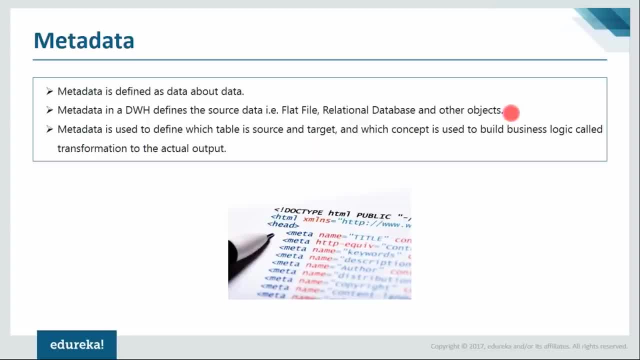 So you'll have to manually update your data into your data warehouse. probably at every day at a particular time, maybe at six o'clock every day in the morning, or maybe once in the night at 10 o'clock, or basically at regular intervals. you've got to store data into your data warehouse. 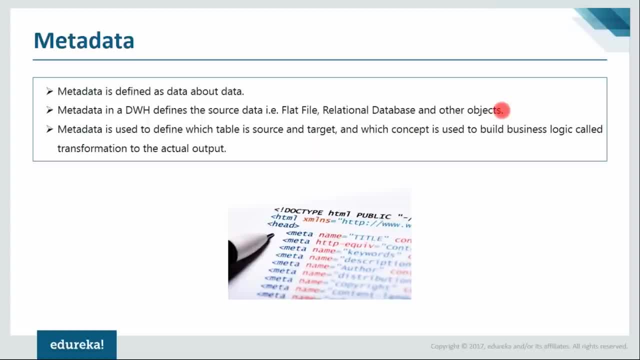 And this whole strategy becomes difficult because you have to do this process every day. So every day when a guy comes in in the morning he has to look at the new data that has come into your database correct, And then from that database, which is data source. 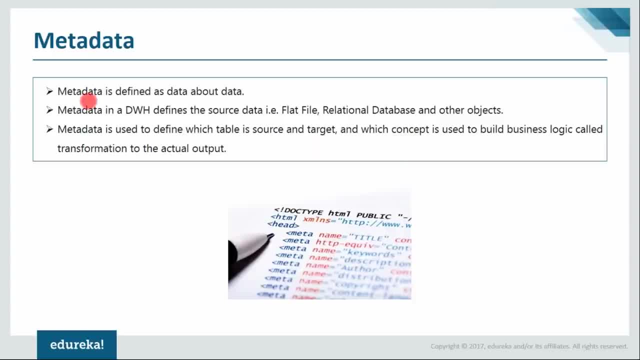 he has to add that data to your data warehouse. This process becomes difficult. So that is where metadata comes in handy. With metadata, you define the address where your data source is okay. You define the address of your flat file from where your data is coming in. 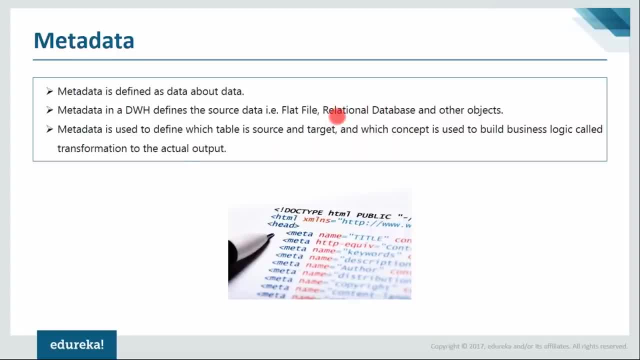 or your relational data, from where your data is coming in, And then you can also, in fact, store the metadata of your data warehouse where you want the data to go. So it basically, you know, saves a lot of your time, okay. 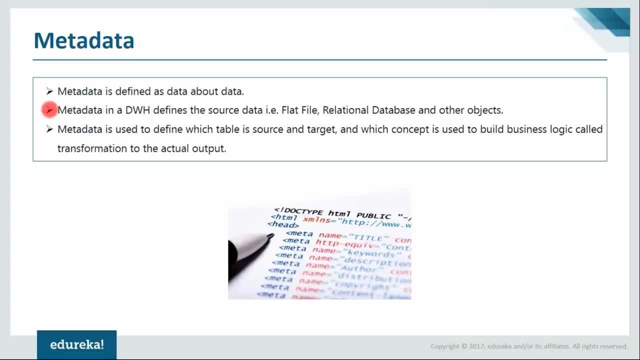 And this is the most common and the most you know unspoken fact about a data warehouse. So any professional that's dealing with data warehouse, you would always be using metadata, because it saves a lot of time, because every time you cannot be importing data. 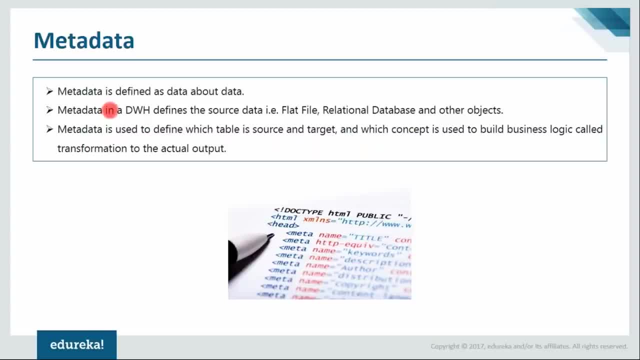 from a database. you always have to get it from your metadata by defining rules and defining your source and your targets correct. So metadata saves a lot of your time, And this is something I'll show you a demonstration on. okay, And when I show a demonstration? 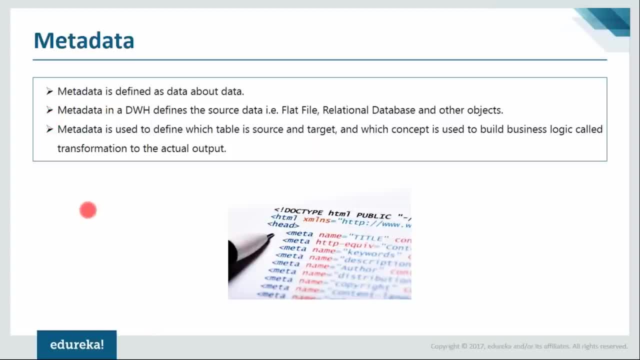 you will understand how easy it is. So you'll just write the rules such that you have your source over here and then you have your destination over here, your target over here, And once you've written this thing, you'll go back here. 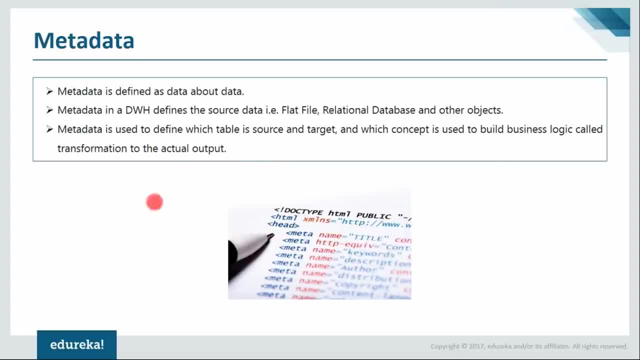 So every day it might pick up the data from here and it might move to your data warehouse and all these things. It will update all the new details which are present in your database and it'll add it into your data warehouse. So that's what a metadata does. 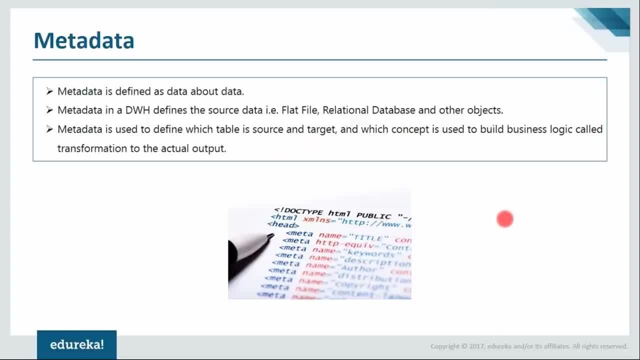 It's a very big advantage and it's one of the best strategies that we can go for. okay, And then the final point here is: metadata is used to define which table is source and target and which concept is used to build business logic called transformation to the actual output. 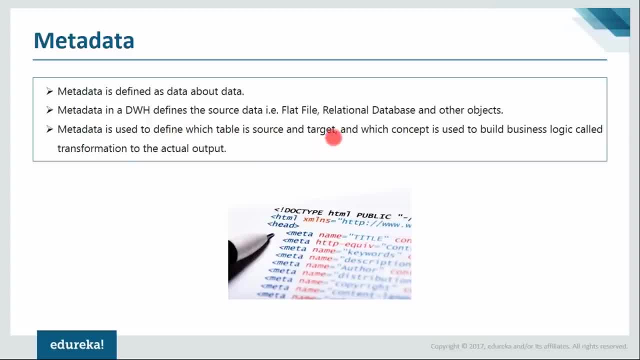 Yeah, this is what I told you right. So it's used to define source and target and how to build your business logic called transformation. So transformation is basically your act of converting your source data into the form that you want to, and what is the logic that you use? correct? 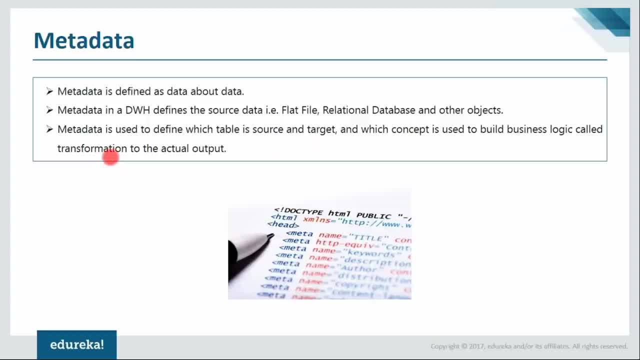 So all the different the filter criterias, all the transformation criterias, all these things can be also done using the metadata correct. So even the process of forgetting data from your source, your destination, it can involve extra additional steps which can save your time. 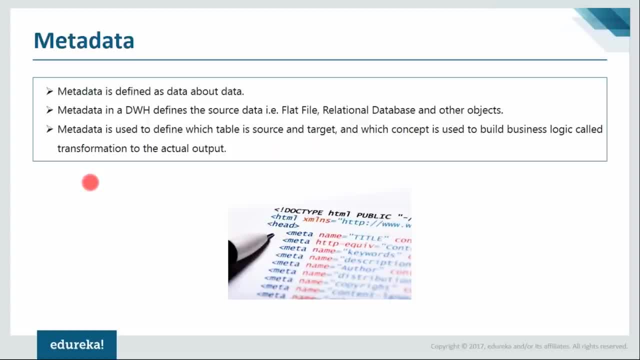 and default process, basically. So every time you have data in a particular format, you might want to store it in a different format, and for all that purpose you can use a metadata, right? So, since things will all already be defined here, 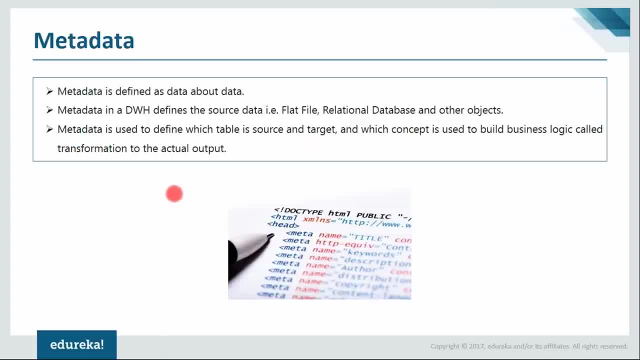 the work of metadata is just to get the data from the source defined and do the set of activities that is required and which is already defined. It will perform all those activities and it will store it in the place where you want it to. So that is the role of a metadata, correct? 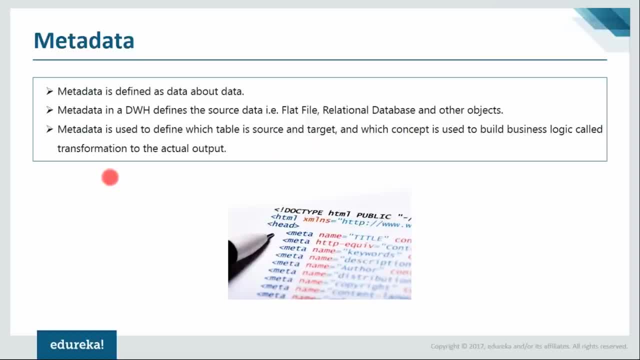 So metadata is very, very important and it's very, very highly used, And it's actually the most important, or let's say it's the epitome of data warehousing. okay, This is probably the best thing that can happen to data warehousing, right. 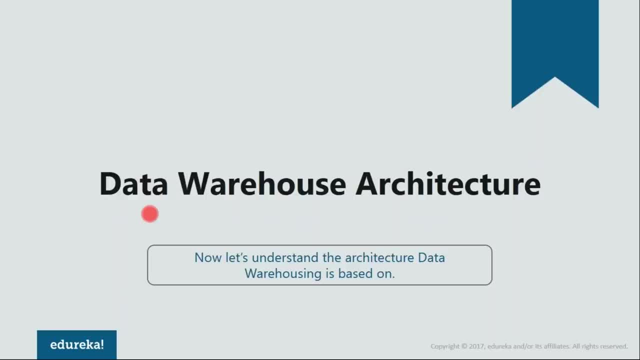 So that's the thing about metadata, guys. Now, going to the next slide, we have the architecture. So now that you know everything, okay, these four terminologies are more than enough for you to understand the architecture. okay, So let's understand what the architecture is. 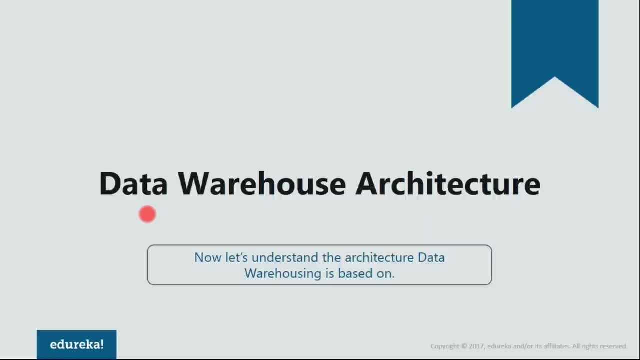 So this is the entire architecture diagram. okay, So this is what you know. data comes in from various sources. It can come from either a database or it can come from a flat file, and then that data, an action of ETL, will be performed. 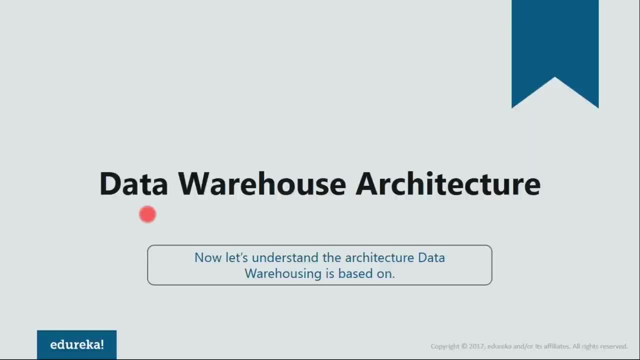 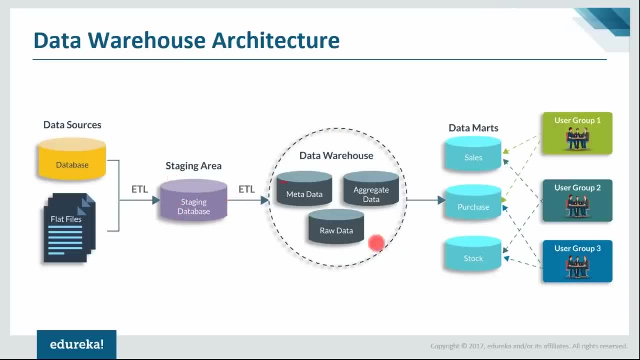 on that data and it will go to the staging area. okay, This is called the staging area and this is the staging database And the data that is stored over here. it is temporary data Before the data completely moves to the data warehouse. 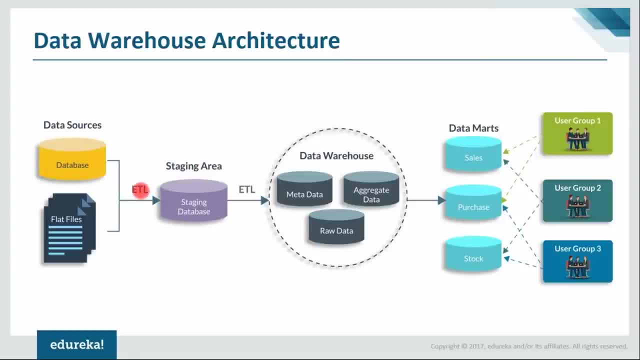 it'll be present in this area, okay, And that is done by using the act of ETL And also between moving to the data warehouse, the process of ETL continues. So ETL process starts over here and it ends over here, okay. 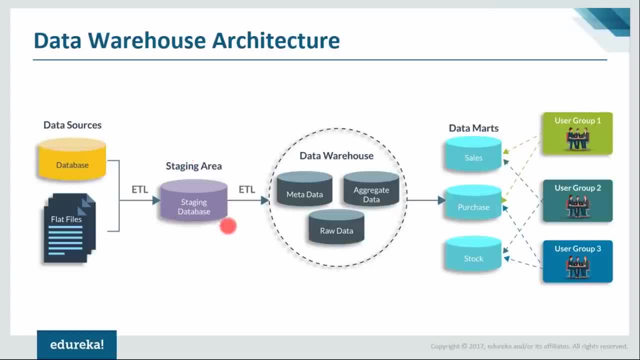 Between the conversion, it is temporarily stored in a staging area, And this is most often present inside the ETL tool itself. okay, like your talent or Informatica and all these things, And then this data will be stored in your data warehouse. 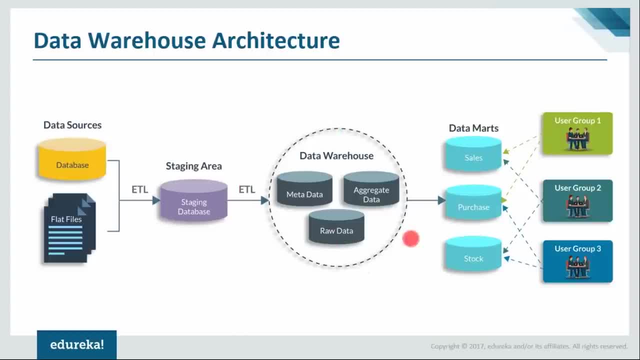 So whatever is extracted, transformed and loaded, it'll be loaded into your data warehouse And in your data warehouse you'll have metadata, okay, And of course, you'll have your raw data and then you'll have your aggregate data, okay. 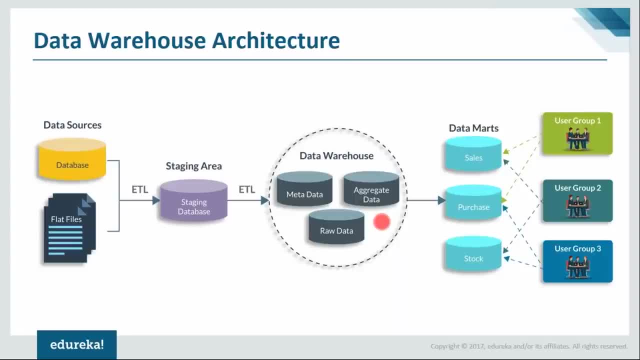 And this is the reason why a data warehouse is generally. you know it's larger in size, Okay, And this is the reason why a data warehouse is generally. you know it's larger in size, Okay, And this is the reason why a data warehouse is generally. 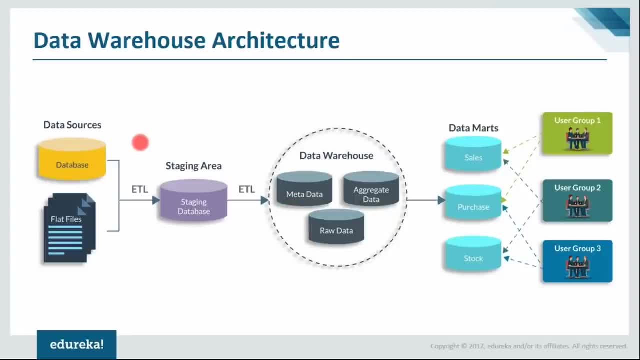 because it has not just raw data. Your database, which from where the data's coming in, it'll only have your raw data, okay, But your data warehouse will have additional stuff here It'll have also your metadata and your aggregate data. 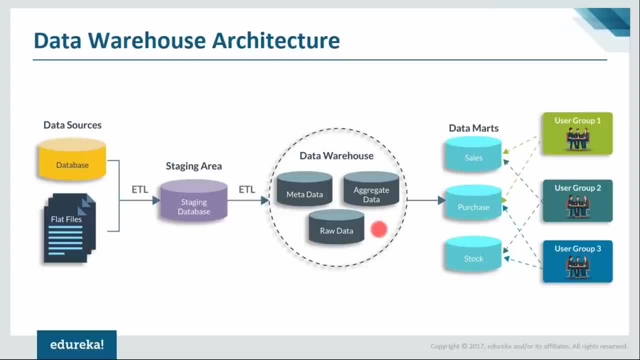 And together all these three things together is what helping you, being you doing your analysis sooner- okay. This is what powers your ability to do OLAP online analytical processing- okay. So that's what a data warehouse is and that's what it stores. 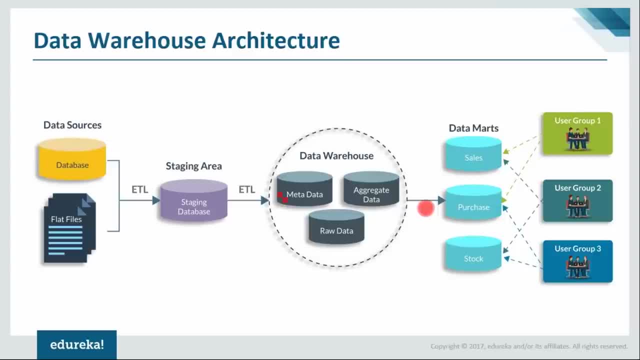 And then this data warehouse. you can- either your entire company can- use a data warehouse, or, if you want more of a security-based access, then you can divide it into different data marts where your sales team and your different teams- like here, we have a purchase table. 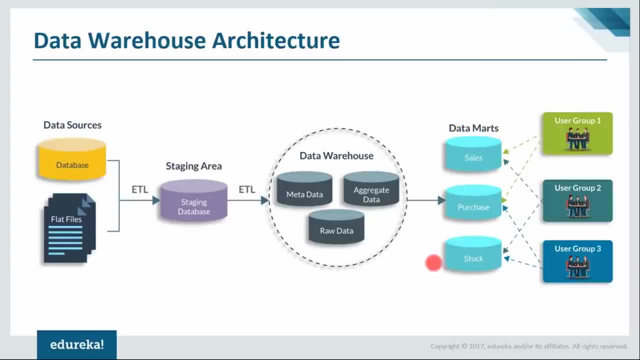 and then you have your stock table. So these are like three different marts data, marts for three tables, like sales, purchase and stock. So you'll have different tables here and different teams can access different set of tables. okay, 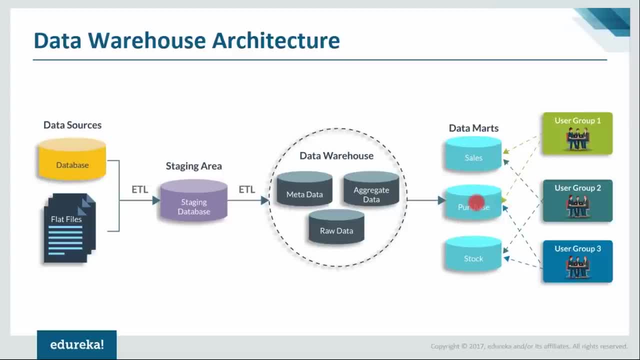 Your purchase can be something that's used by your operations- people, right- And then this may be something that's used by your sales people, And your stock may be again used by your operations or your sales group. So that's what each of these here defines. 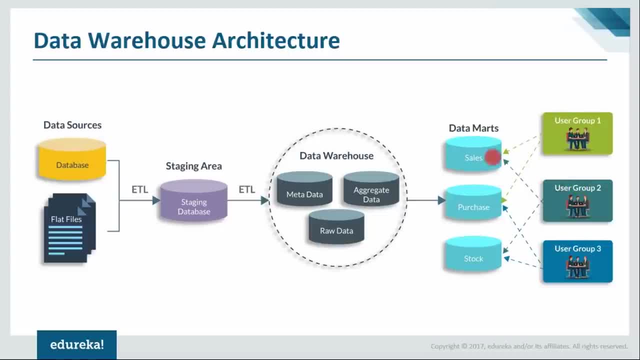 You have your user group one, user group two and user group three, And each group will be getting access to different parts of your data warehouse because your data warehouse will be divided into different data marts and your data, your different groups. 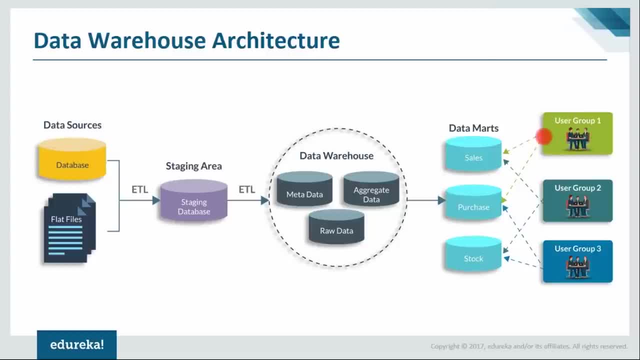 we get access to only that data which they want to or which they can get access to correct. So this way, no group can get access to every data that is present in a data warehouse and you can get access to all of that data, okay. 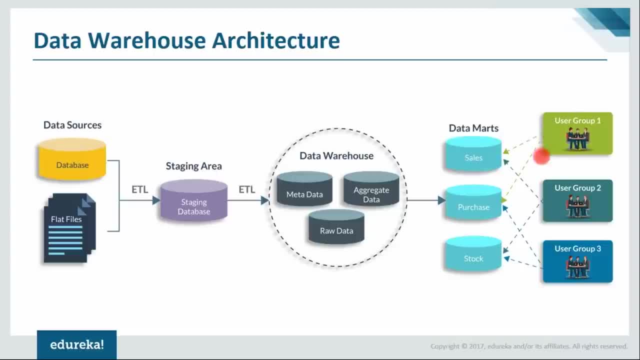 And there's advanced, there's a little more data security in this case. okay, Same thing over here. So this group gets access only to this data and this data and this table or this mart, right? And then this user group gets access. 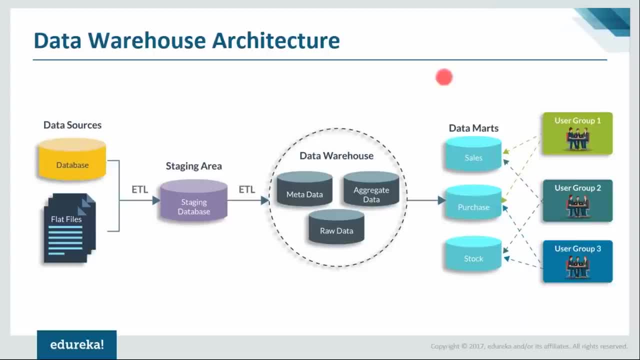 to only the data that is present in this mart and in this mart. So that's what the entire architecture looks like and this is how the data flow is right. So if you guys have understood this much, then you're ready to get a demonstration, correct, guys? 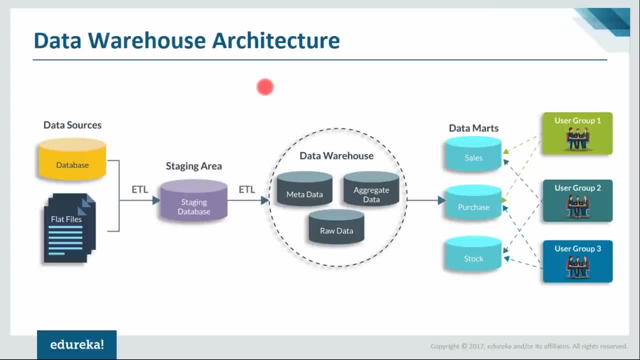 And this is also my last topic in this presentation. so right now I can go to my demonstration and what I'll be doing in my demonstration is I'll be using talent. okay, So I'll be importing data from my database. I'll be using, I'll be getting it from my Oracle database. 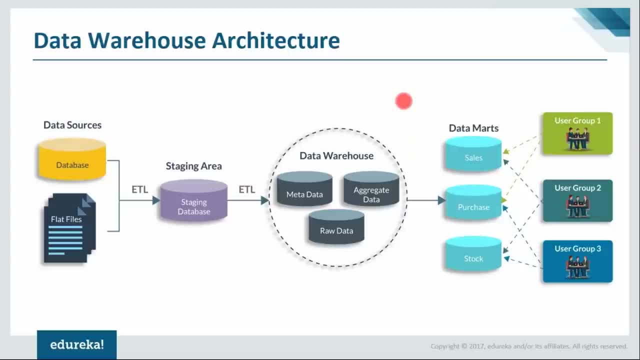 and I'll be storing that into a data warehouse which can be ready for any kind of analysis or visualization on any other visualization tool. okay, So this act over here which I'm gonna show you, this is what powers your business intelligence, right? 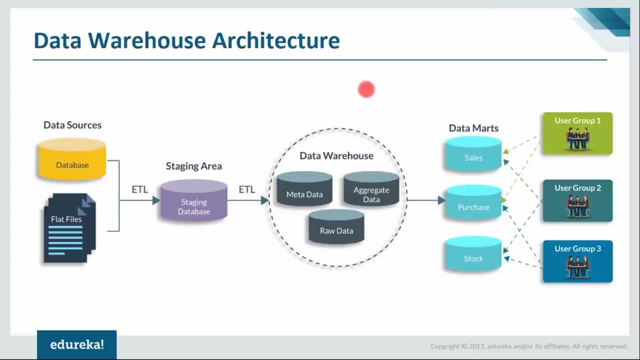 So are you guys ready for the demonstration? Any doubts here, guys? Okay, great Rodney says he's all ready. he's all pumped up. All right, Rodney, that's very good. So Jacob's also ready, and so is Rajesh. 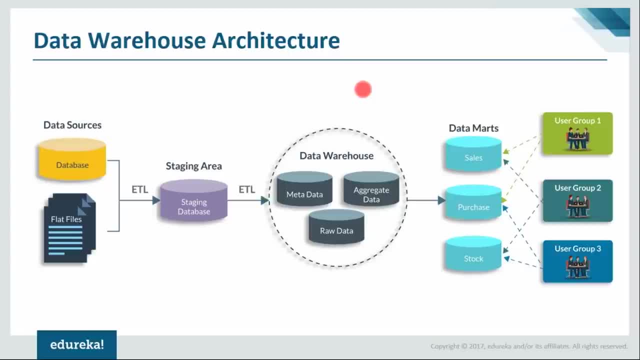 Are you Rajesh? Can I get a yes from you? Yes, very good, very good, attaboy Rajesh. So let's go. So let's go to the next part of my session, and this is gonna be demonstration. 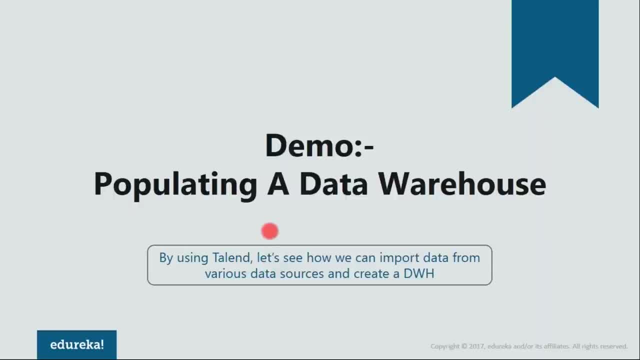 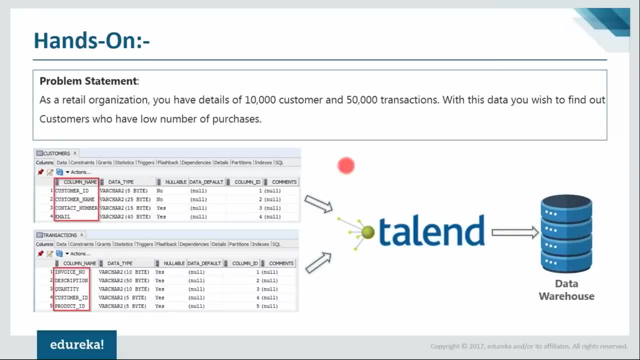 where I'll populate a data warehouse. okay, I'll be using talent for the data warehouse activities and let's see how we can import data from various data sources and create a data warehouse. So for our hands-on session, I'll be importing. 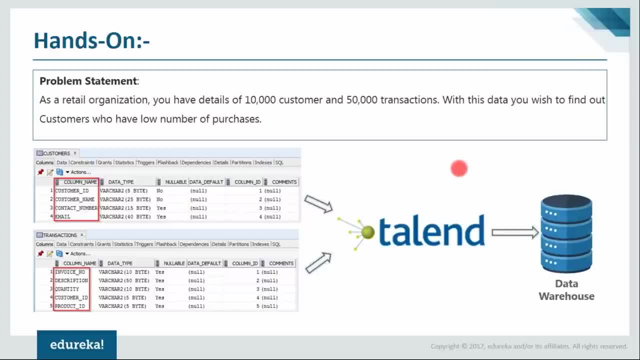 data into my talent BI. okay, Like I said earlier, I'll be using my talent BI for my data warehousing and ETL processes and I'll create a data warehouse using talent BI. okay, Now the data set that I'll be using. 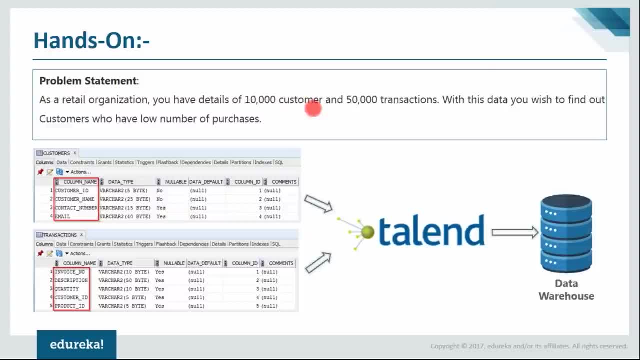 is that of a 10,000-row table and a 3,000-row table, okay. So there'll be one table having 10,000 customer details, okay, and then there'll be another table having 50,000 rows of transactions. 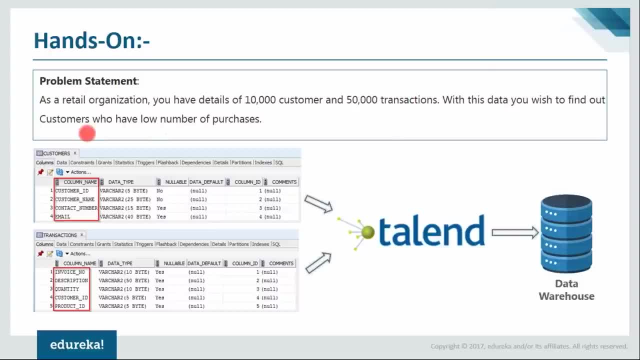 which either of those customers make. Okay, now, based on this data, we have to find those customers who have the lowest number of purchases. okay, So right now my data set is present in my Oracle database. okay, so I have two tables and both my tables. 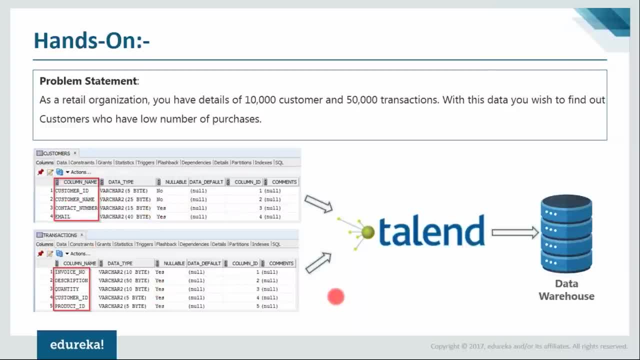 customer's table and my transaction's table is present in my Oracle database. I also have them in my Excel, so first let me show you how they are present in my Excel file. okay, Okay. so this is my customer table. 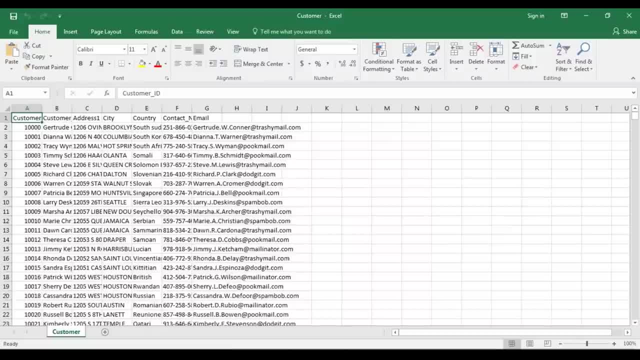 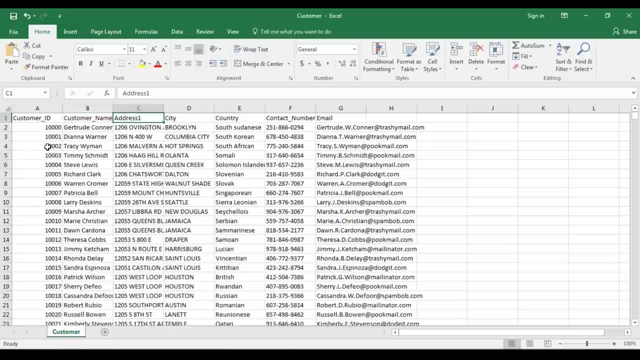 As you can see, we have all these details right. We have all these fields here. So we have our customer ID, we have customer name, we have the address of that customer city, the country he's from. the contact number: 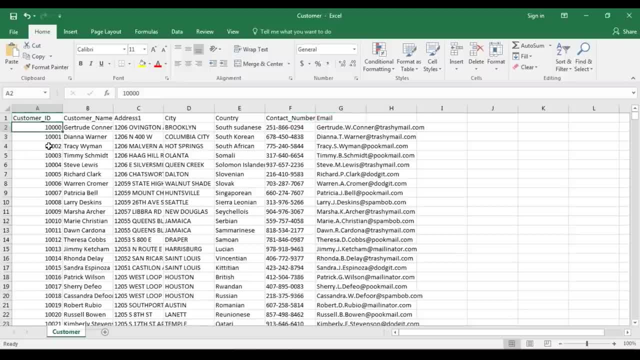 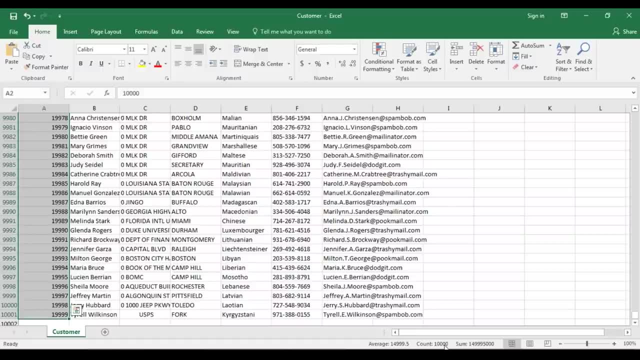 and his email address right, And if I do this, then you can see that there are almost 10,000 fields here, so 10,000 rows are there here, So this means that I have it's a pretty big data set. 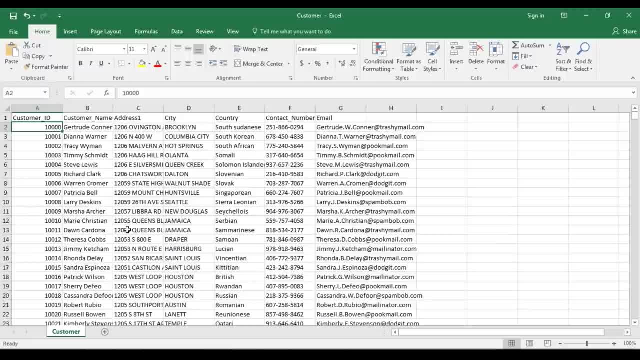 and I can use this in combination with my other table. okay, So here we have customer ID as the primary key, okay, And if I go back to my other data set, that's my transaction's table- you can see that I have further more fields here. 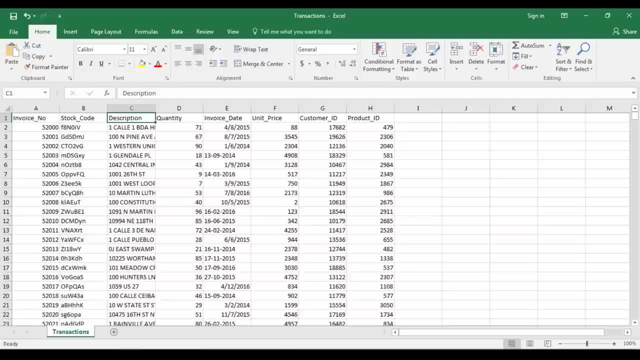 I have those of invoice number, I have stock code, I have description, I have quantity, I have invoice date, unit, price, customer ID and product ID. okay, So there's a customer ID over here also. So the customer ID is the primary key over there. 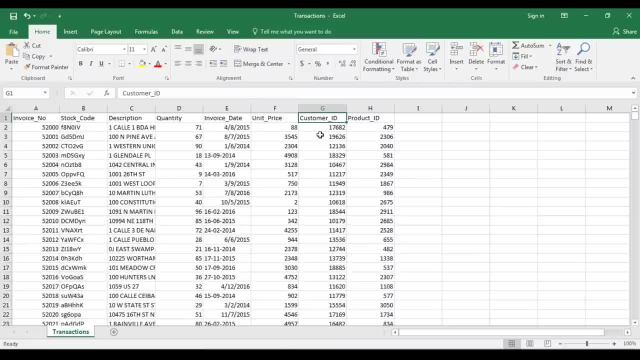 and this is the foreign key over here. So basically, the customer ID is the same and I will have to do a lookup to that table with the help of my customer ID. okay, Since these are two different tables, I can create my data warehouse with the help of. 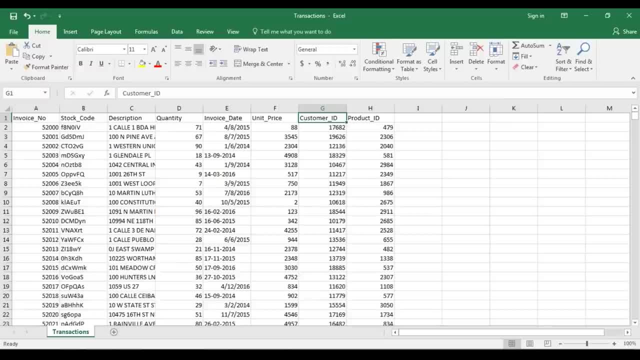 this particular primary and foreign key concept. I can create a link and I can create, I can probably just link these two tables with the primary key, foreign key concept. okay, So any doubts, guys, I'm sure that you all know what a primary key. 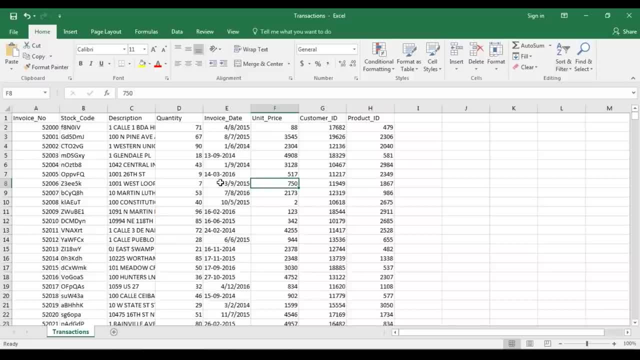 and a foreign key is, and if at all anybody has a problem, please let me know, okay. So Rodney says I don't know what's a foreign key, Okay, so see, Rodney, the thing is we have something called as a primary key. 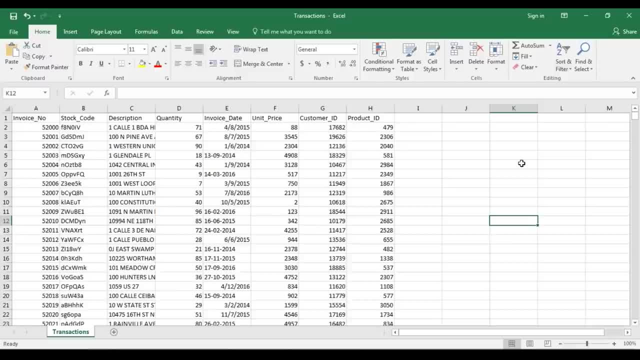 and a foreign key. okay, And we use these two columns when you want to use a combination of two different tables, right? So if you consider the example of this one, then you can see that there are a number of columns here. 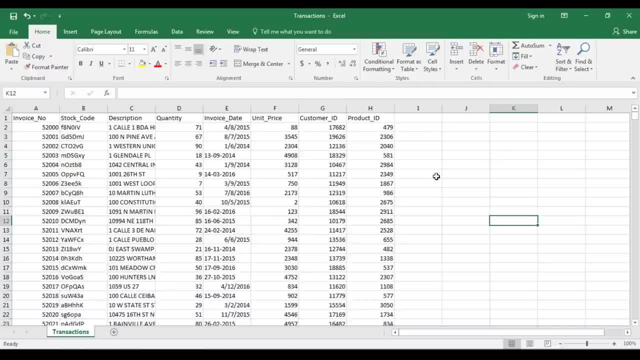 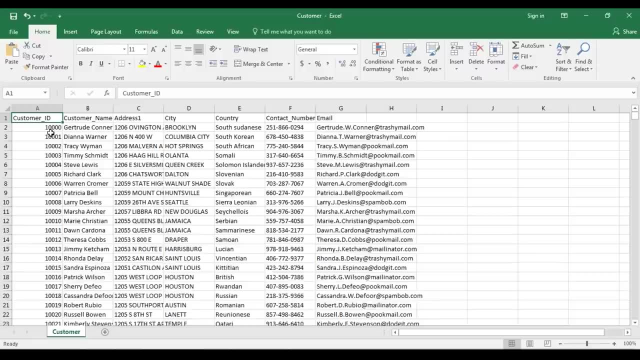 and not everything is matching with the details in that part in the other table. okay, So only customer ID is the only common field. Okay, so there's a customer ID here and even in this table we have a customer ID. Now the thing is, the customer ID is a primary key. 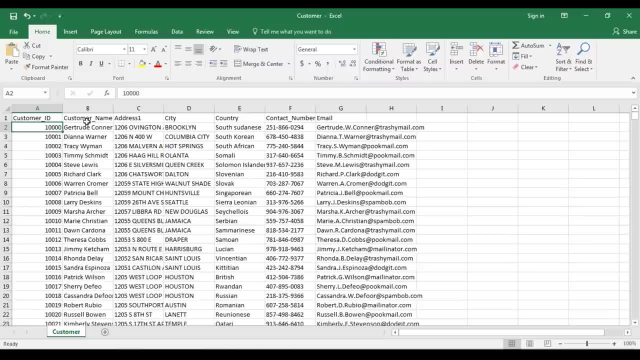 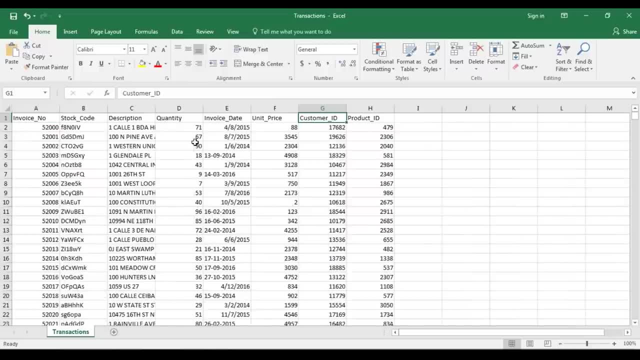 because it's constant and it's unique for each and every single record over here. So each and every customer here will have a separate customer ID, okay, So no two customers will have the same customer ID, okay, And over here the transactions here. 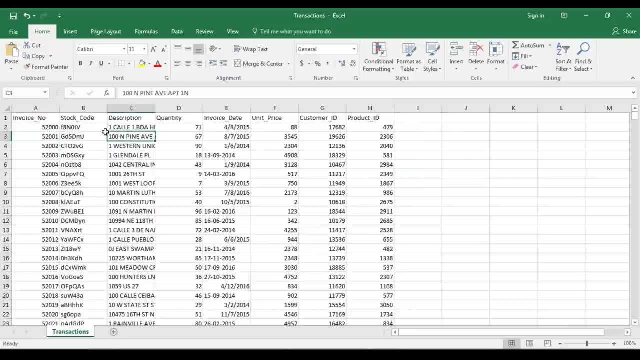 which has the invoice number, the description of the product that was purchased, the stock code, the quantity. all these things are sorted by the customer ID, okay, So if you find a particular customer ID more than once, then well, here you can find the customer ID more than once. 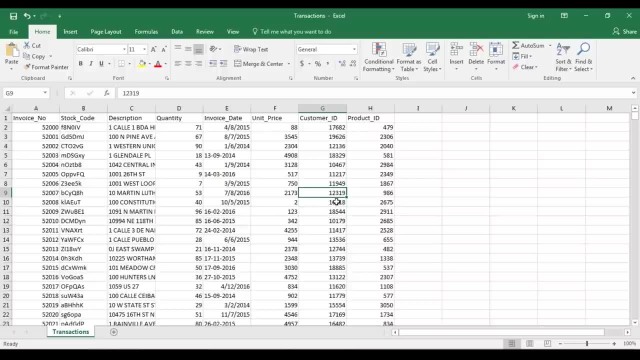 That's because a customer would have made more than one transaction. He might have come onto their, he might have bought from the same the same person more than twice or thrice or four times or something like that. right? So supposing I go back to this person. 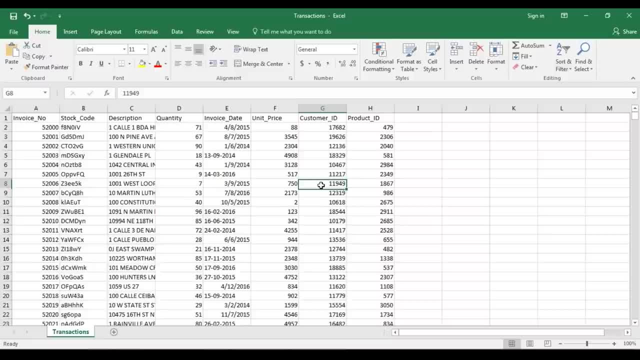 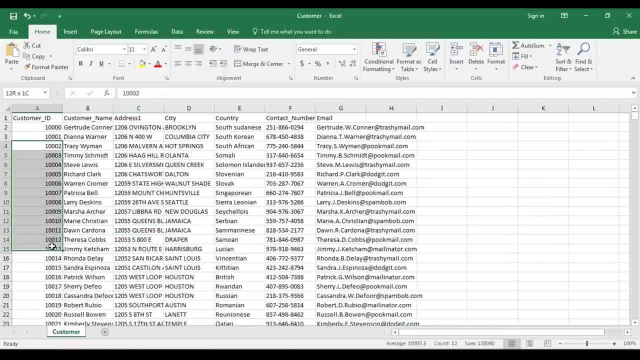 and I buy his products. since it's a retail store, I buy products, say, 50 times, then I'll have 50 different times. my customer ID will appear here, okay, But however, it will not appear again because it's a primary key right here. 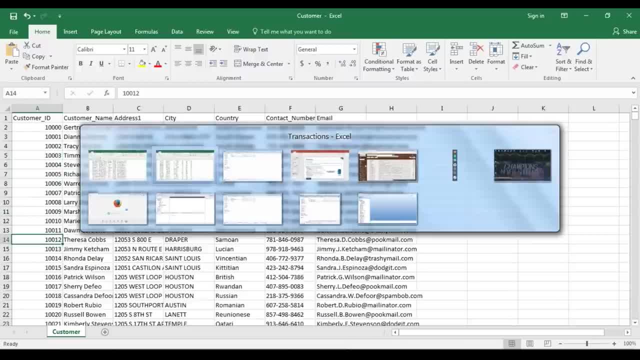 So that's the difference. So here the uniqueness is there. That's why it's called the primary key in this case, And here there's no uniqueness for the customer ID. okay, It can appear more than once and that's why it's a foreign key over here. 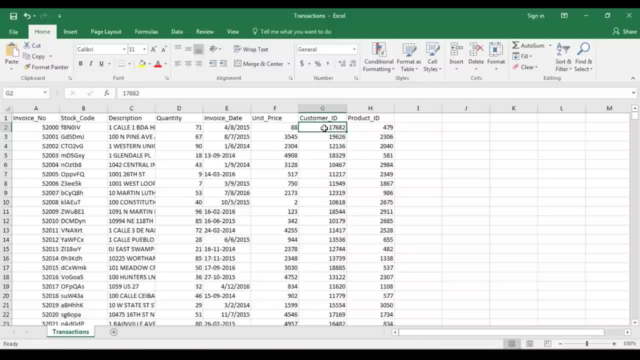 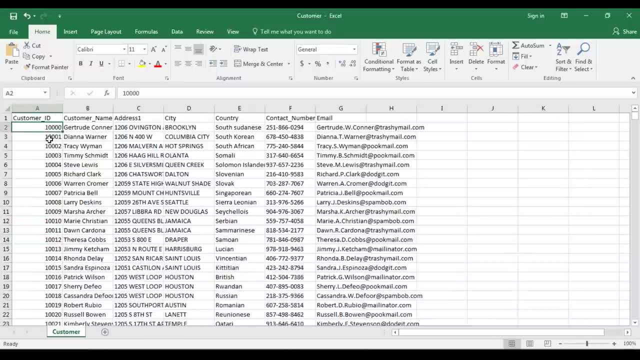 And what we're gonna do is for every customer ID over here, right? So for every customer ID over here, we're gonna link it to this particular table with the help of this customer ID, Since the customer ID is a common field in both the cases. 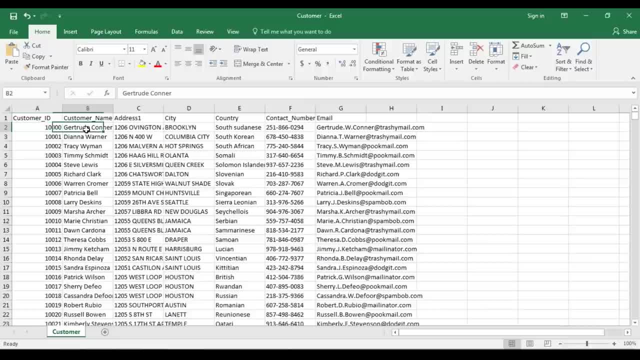 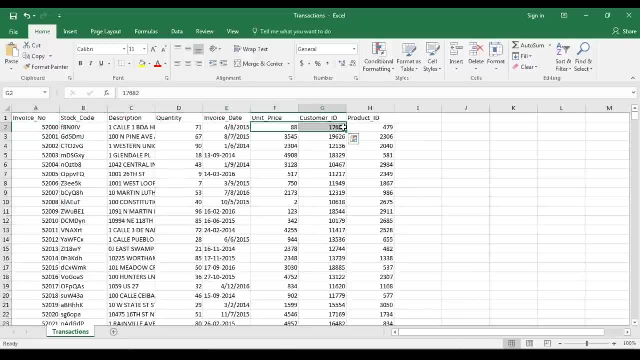 I can make a table which would show which customer, which would probably display all these details along with the other columns. okay, Now, that's because I have customer ID, which is common in both the tables, And using that I can link the fields that are there. okay, 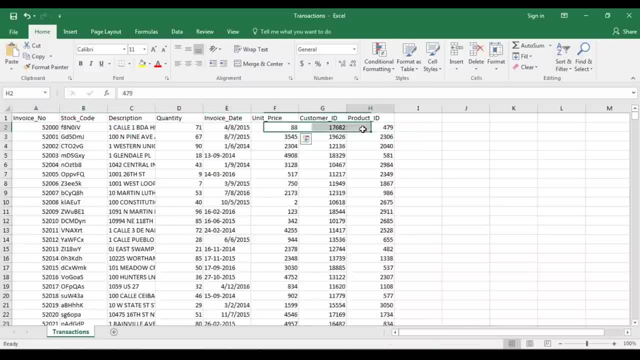 And, using that, I can link the fields that are there, okay, And using that, I can link the fields that are there, okay, Which are there in this table and which are there in the customer's table, right. So that's what I'm gonna do. 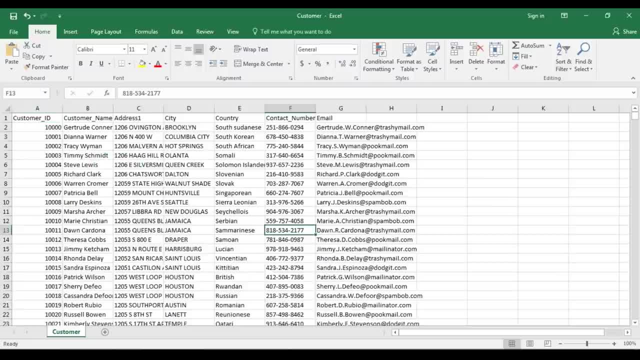 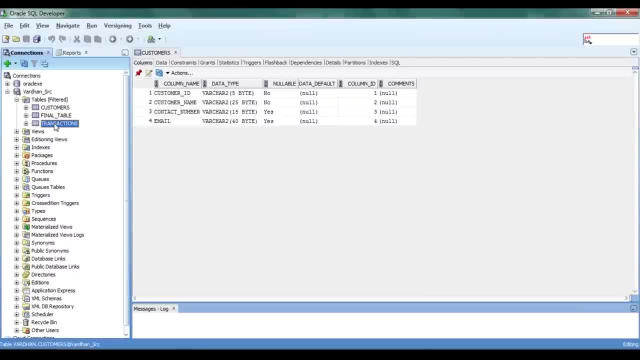 Now the similar thing is also there in my Oracle database, So let me show you that. So this is my SQL developer GUI. okay, So I have two tables here. I have customer's table and I have transaction's table. right, 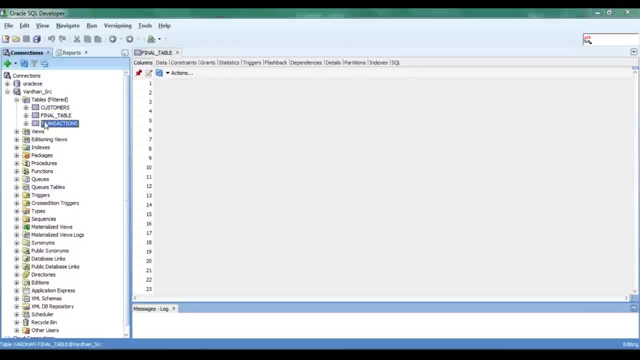 And then I have a final table, but this is not something which is relevant, so this is not something we'll be using, But we have the same two tables: customer's table and transaction's table. as I showed you, We have these two here. 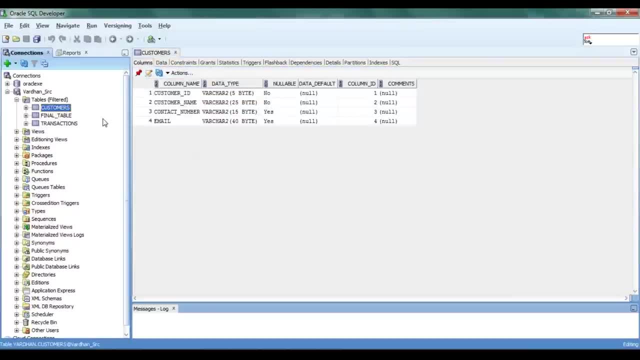 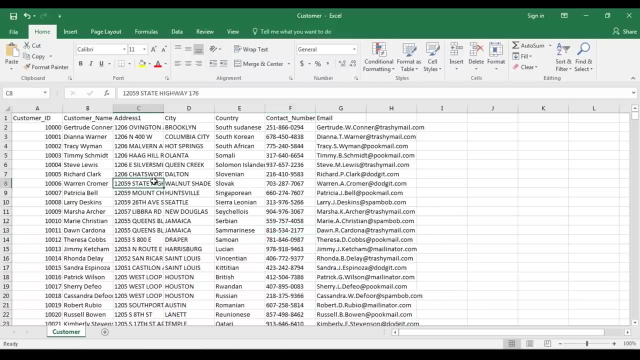 and we have almost the same fields over here, Because if you see the customer's table, we have the customer ID, we have the customer name, we have the customer number and the email address. okay, And here we have additionally. 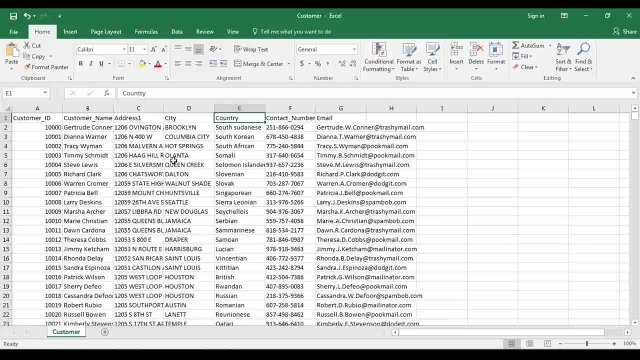 we have the address, city and country. Now what I did is, when I imported this Excel file into my database, I ignored these three columns, right? I didn't want these details because I was not gonna use them in my data warehouse. 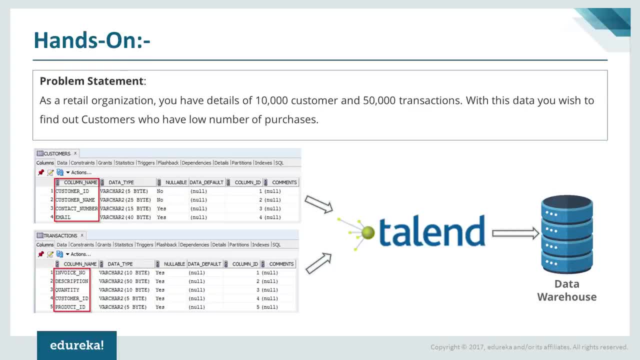 So if you see our problem statement here, it only says you have to find out the customers who have the lower number of purchases. It doesn't mention that you need their country details Or city details or anything for that matter of fact. So for that reason, using the country, city, 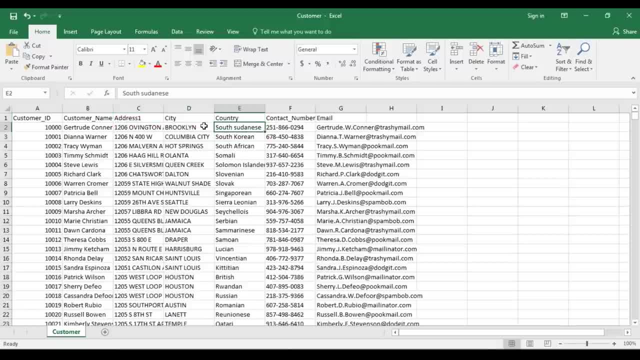 and address fields would be a waste, So that's why I've not imported these into my data warehouse. I have only the customer ID, the customer name, my contact number and my email address fields. okay, This would be sufficient to find out the customer details. 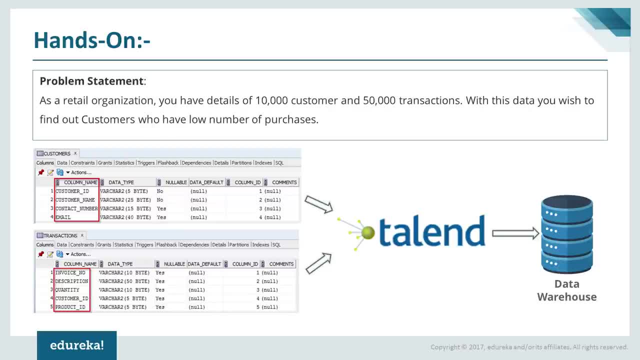 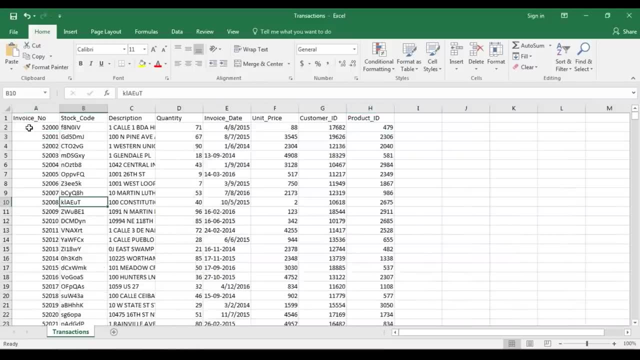 Okay, and to find the purchases right and to see who has all the lowest purchases, we can use the other table. So in the other table, that is the transactions table, we have this quantity field right, We have this column. 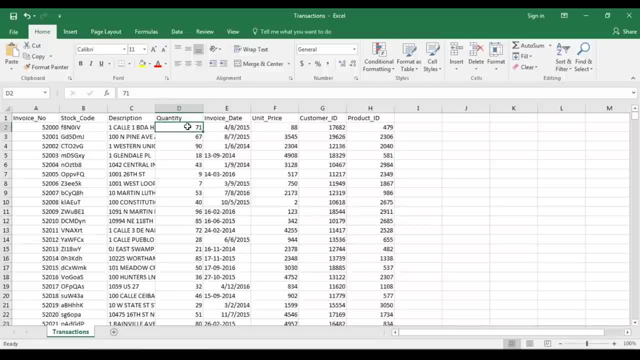 This quantity table basically represents how many products this particular person purchased. So this person with this customer ID purchased 71 products, right? and then you have another person who has purchased 67 products, and so on. So you also have people who purchased only seven or nine. 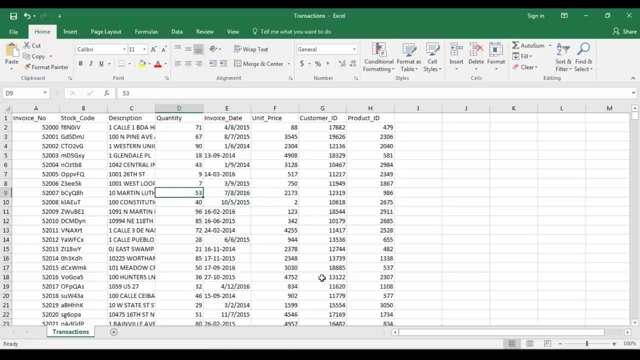 Okay, now our problem statement is such that we have to find those people who have made a very less number of purchases. okay, Now, if we define less to be 10, then we can extract the data such that the data warehouse gets the details of only those people who have made purchases. 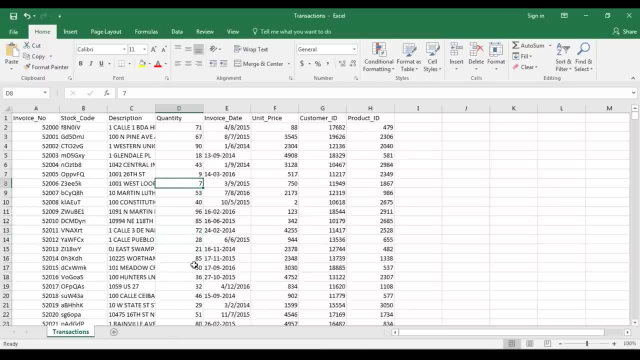 of less than 10 items per order, right. So, per transaction, whoever has made less than 10 purchases. So this person has made seven and this person has made nine- right, So we can get a list of those customers, right. 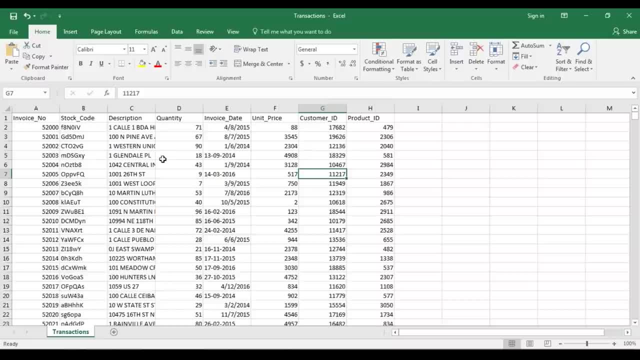 Using the customer ID. we can go to that customer table and get his name, We can get his email address, his phone number and other details, okay, And we can publish all those things and we can probably export them to another CSV file like this: 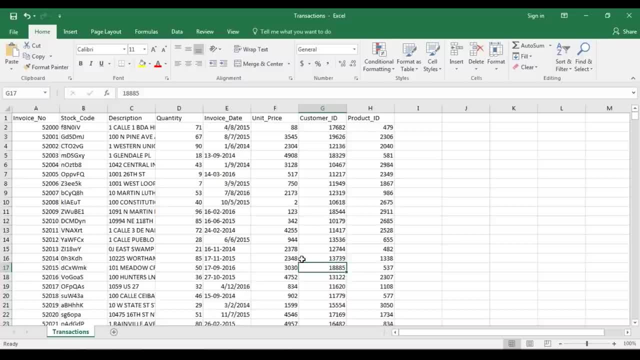 or we can put that into our database, basically into anything which would support data visualization, right? So that's what we want and this function is what our talent is gonna do, okay, and what I'm gonna do for that purpose is: I'm gonna do a lookup. 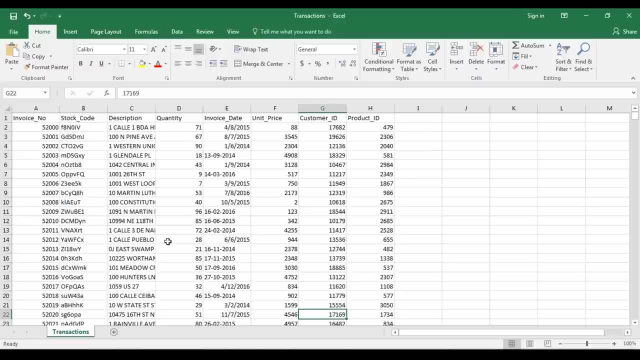 from this table onto my customer's table, right. So this is my transaction table and from here I'm gonna use the customer ID field to look up to my customer's table to obtain their name, email address and phone number and all those things. 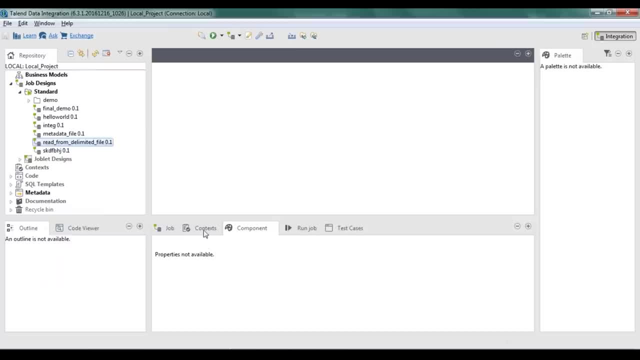 So first of all, let me introduce you to our talent interface. okay, So this was the Oracle SQL database which I showed you earlier, and this one is the talent right. so Talent Open Studio. This is basically the data integration version of the project, okay. 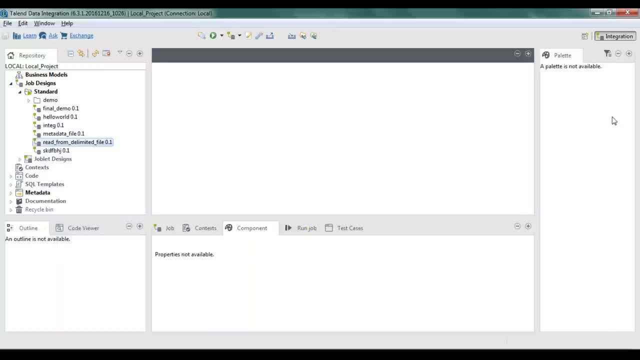 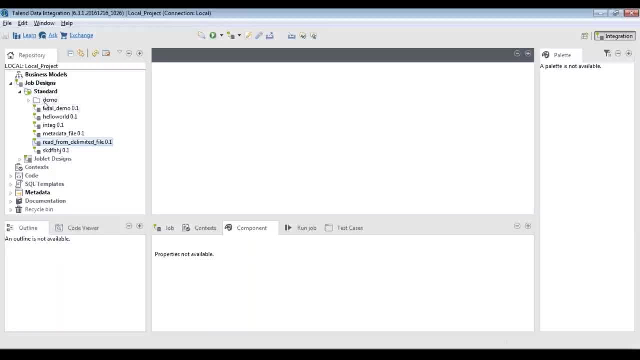 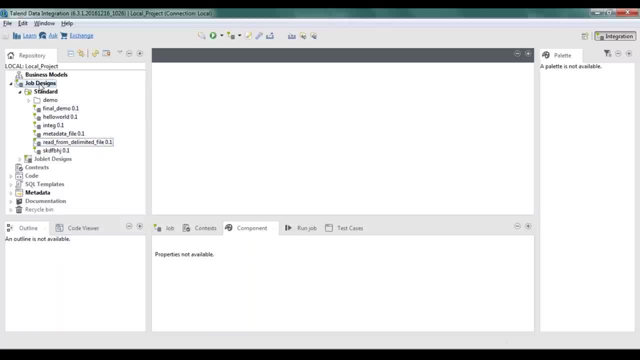 So all these are the different projects that I have created. okay, And when we say job design, so job design is what you use to create your jobs on the UI here. okay, So in our case, in talent, whatever actions are performed, right. 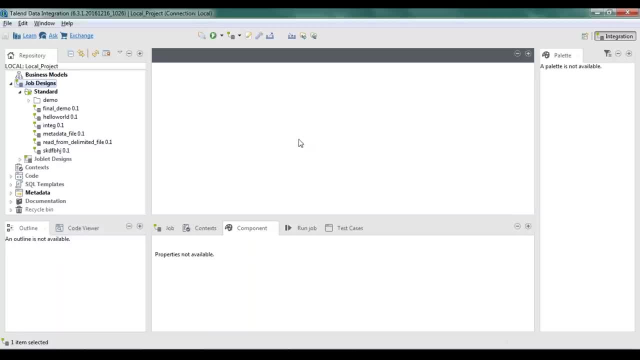 We gotta do it with respect to a UI, So we don't have a. this is not a coding interface, okay? So of course this talent runs on Java, but we don't. but talent is known for its GUI, okay. 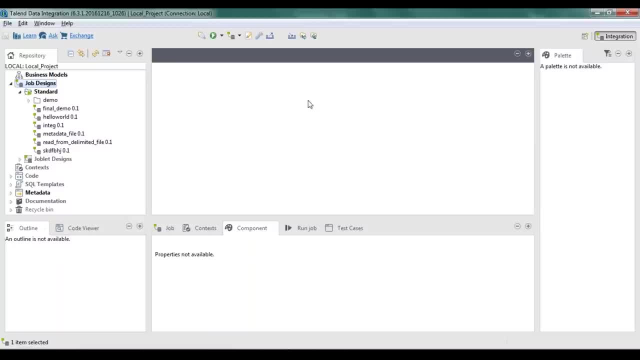 So we can drag and drop the items on the job task. So this is the job design taskbar and we can first of all create a new task, Supposing I want to create a new database by importing radials from another database. Then we can start by creating a new job design. 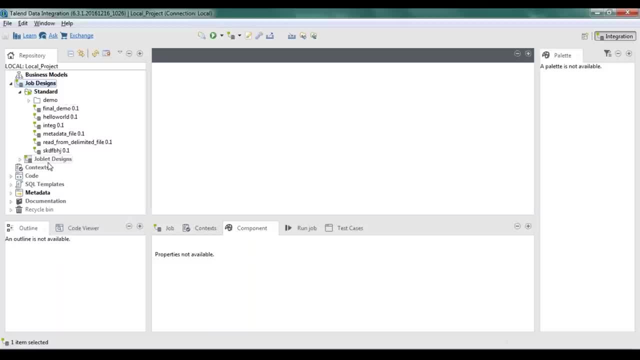 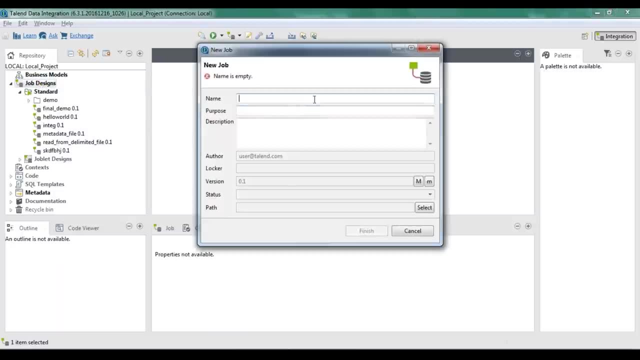 Okay, and then create a new project in that job design. So right now we are in my local project, So I'm gonna create a new job design. I want to say create standard job. Let's give a name to this particular job. So let's say data warehousing, BI session. 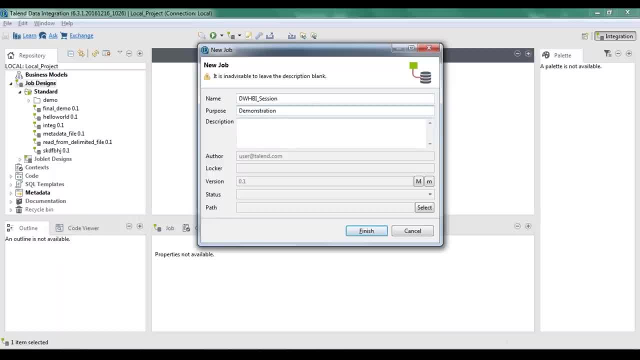 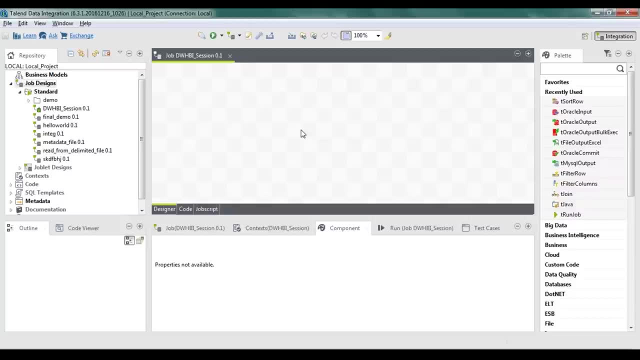 Okay, and demonstration is the purpose. So I'm just gonna copy paste the same details into my description field also and I'm gonna say: finish. Okay, now what you can see here. this is the job designer, So this is where I can get all the data. 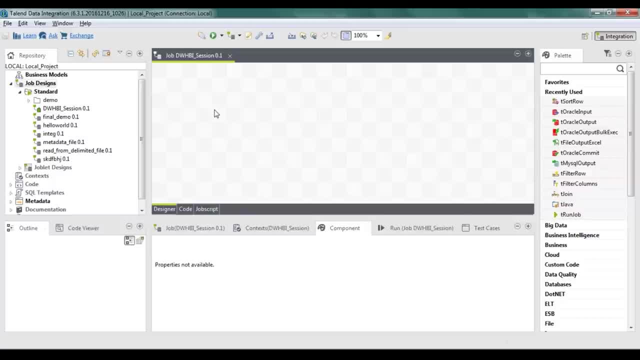 from my different databases or fields or files and get them to my data warehouse So I can write my projects over here, And then on the right hand side you have your pallet. okay, So from your pallet you can choose the files or your database from where you want to import your data. 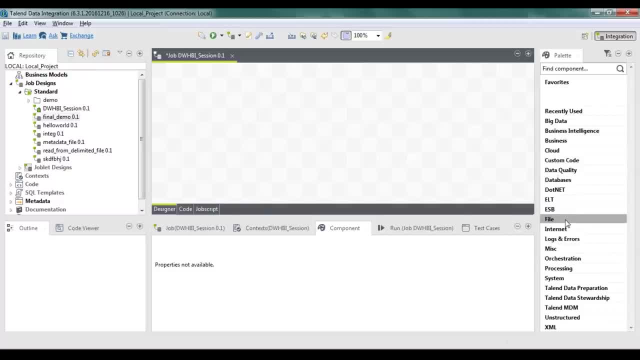 Okay, supposing you want to import from a flat file, Then you can just go to this heading file here. So under file you have input, right. So under input you have all these options. So if you choose any of these options here and if you just drag and drop them over here, 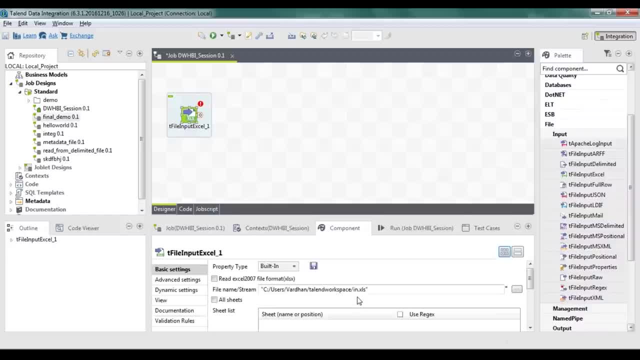 then you can use them as a means to import data. You just need to set the path where the excel file is stored. Okay, and you can choose that, and when you just enter further fields, you can get the data in from these excel files to your data warehouse. okay, to your talent, okay. 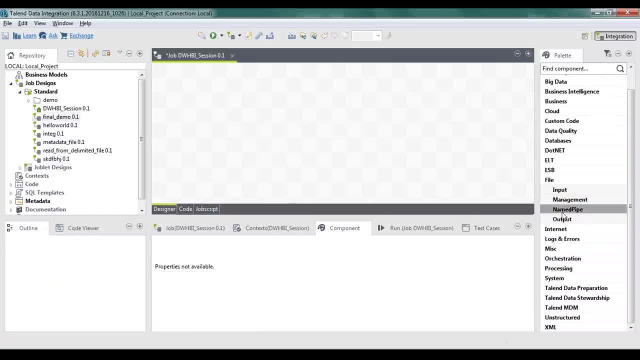 But excel files is a very simple thing and I don't want to show you that. Let me show you how to import this large data from our database, right? So we have also other options here, like big data, big data, business, intelligence- We have business, we have cloud, right. 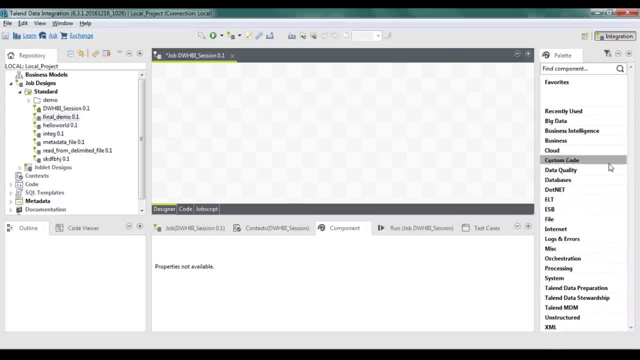 So we have integrations with numerous technologies here, And what we would be concentrating now on is that of databases. right, So I have my Oracle database, so I'm gonna go to, I'm gonna go to Oracle under databases and under Oracle, I'm gonna say the Oracle input. 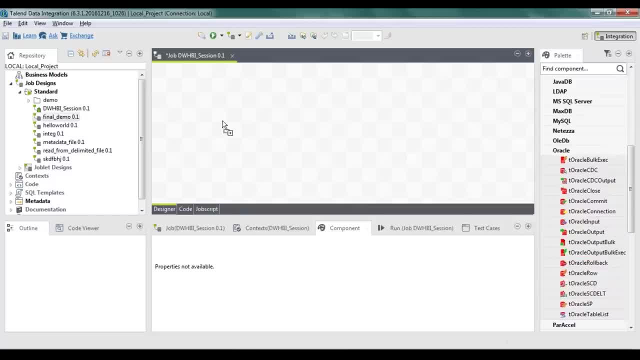 Okay, let's see where is it. The Oracle input is right here, So I'm gonna just click on the Oracle input and paste it here. Okay, I'm gonna drag and drop it here, And now that I've done this, I can use this. 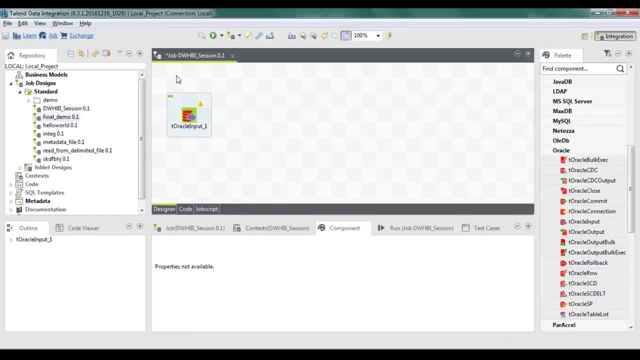 as a means to get my data in from my database. okay, So this is my Oracle database, right? So let me configure my input first. So first of all, I need to configure all these details with respect to my host, the port number on which it's hosted, 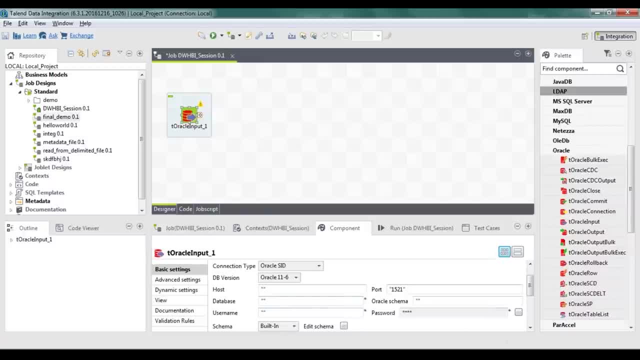 the database name, the username, the password and all these things. okay, So let me first start off from the host. It's hosted on local host, right? It's not on any server, It's not on any remote server, so I'm just gonna say local host. 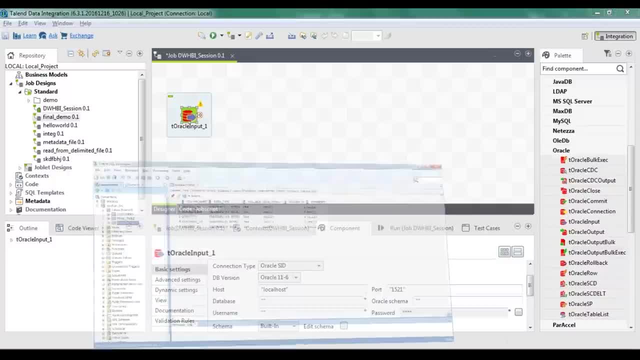 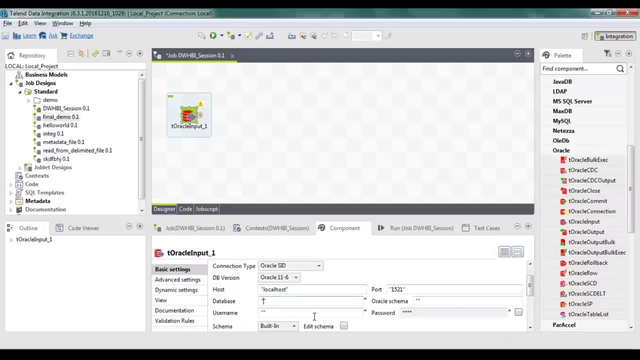 and the port number is 1521.. So these are details that I got when I was when I installed this Oracle SQL server, right, So you'll have to probably enter the same details when you create one, And 1521 is actually the default port. 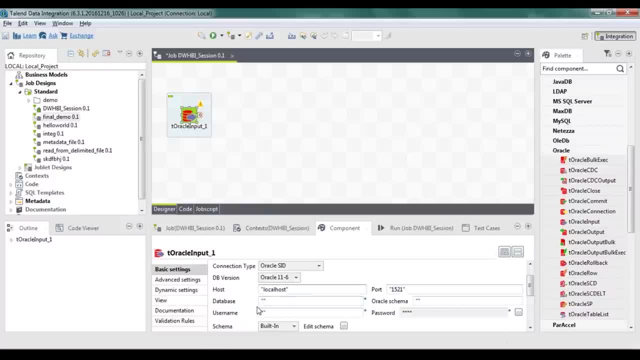 on which Oracle servers usually host it, So you shouldn't have any problem there. So database: here is XE in my case. so Okay, and then my username is Vardhan and the password is something we have to set over here. Okay, all right, and then I've done this. 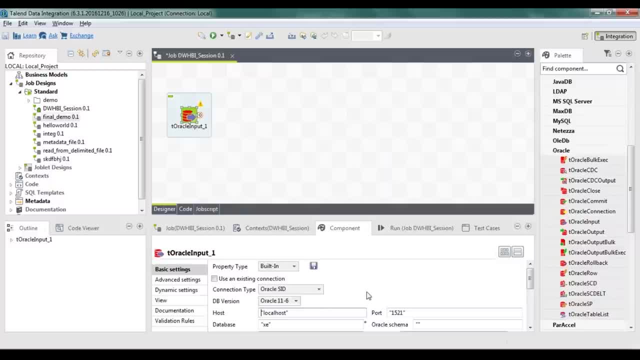 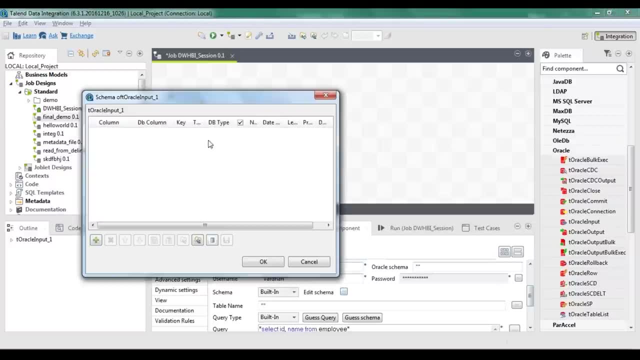 My connection type is Oracle SSID. My database version is 11.6. all right, So all these details here are correct. Now let's check my schema. The schemas, basically, is what is going to. you know, map your fields from your database to your talent, right? 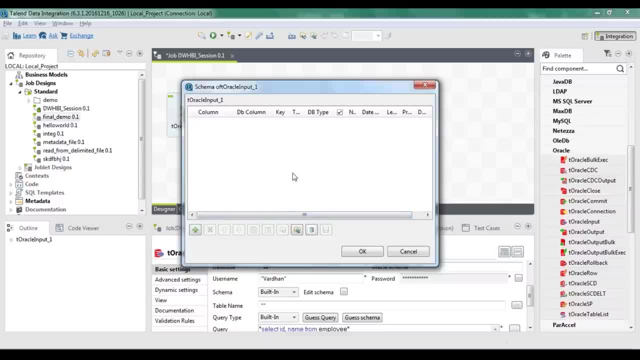 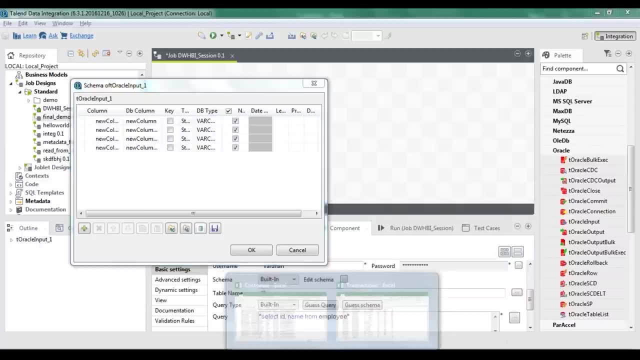 So this is your data warehouse, So we have to define a schema here to add details here. Okay, so now that we have all these fields here, Now let me go back to my database, right? So we are in my customers table and in my customers table. 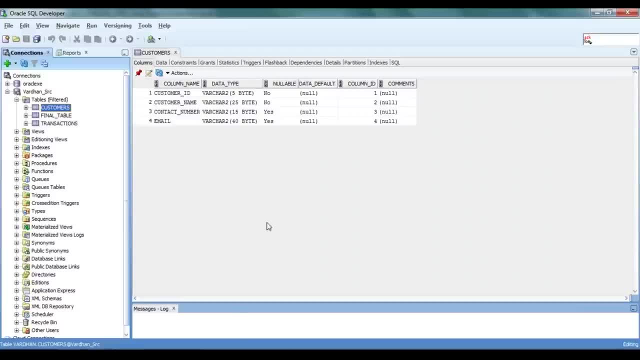 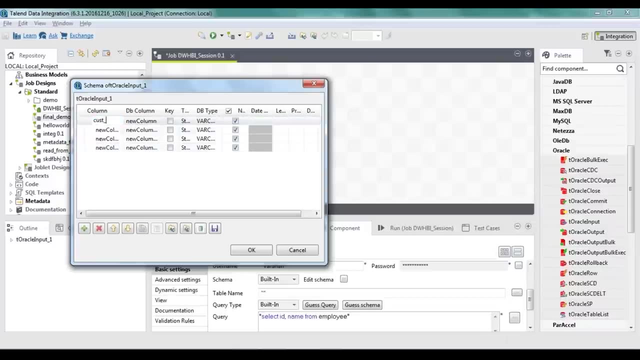 I have four fields: Customer ID, customer name, customer number and email address. So let me add these four fields in my talent. Okay, first column is going to be customer ID. This is going to be customer name. This is going to be customer phone number. 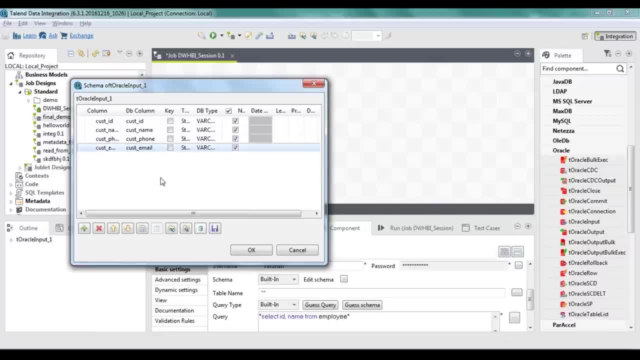 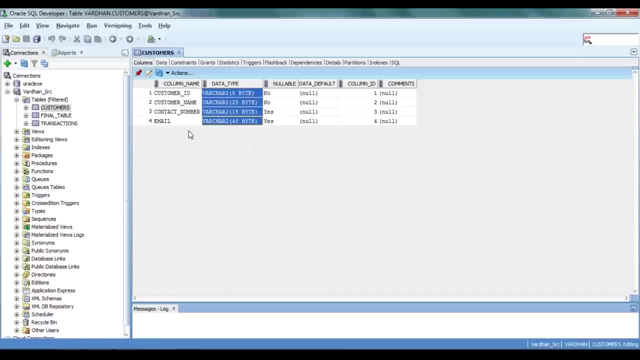 This will be customer email address, all right, So that's all fine. Basically, the data type that it's coming from is all VARCHAR, okay. So if you see here, the data type that is it currently is in is VARCHAR, okay. They have different sizes though, but email address. 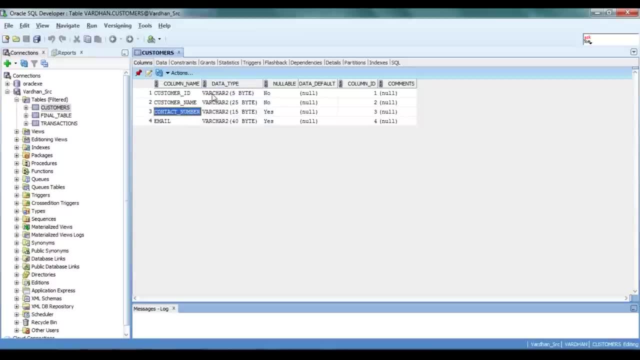 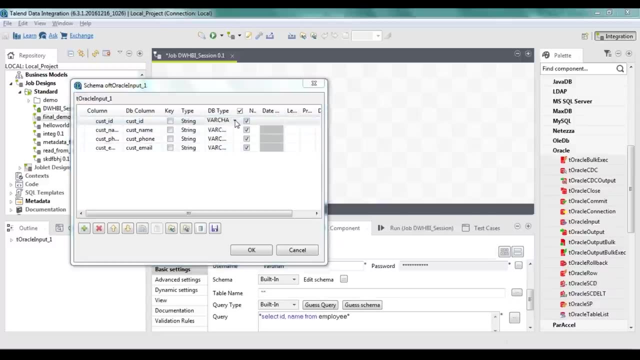 be it email address or contact number or name or ID, all are in VARCHAR2 type. So I'm gonna just say the input also to be as VARCHAR, right? So it's all VARCHAR2.. Everything is technically VARCHAR2.. It's picking up the same data type by default, all right. 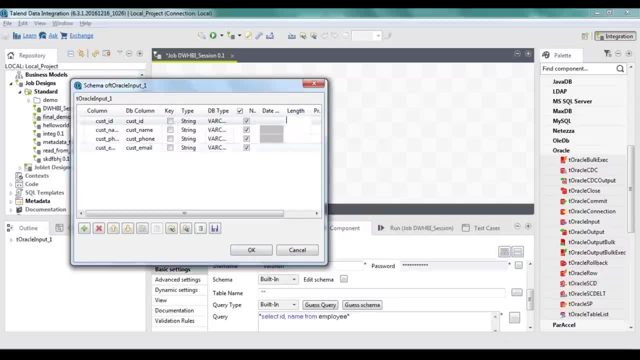 So let's define the length over here though. Let's say the customer ID Is gonna be five characters in length. I'm gonna say the length for the name is gonna be around 30.. The phone number to be around- technically it's 10.. 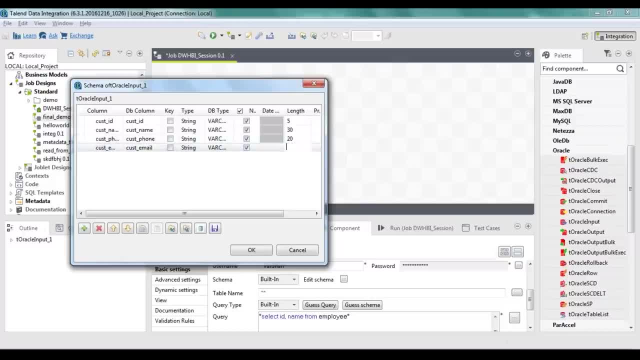 So let's do a buffer of another 10 and say 20.. Email address is gonna be another 20 characters, okay. The customer ID: let me just increase the length to 10.. So these are the length of the fields which are gonna be stored, okay. 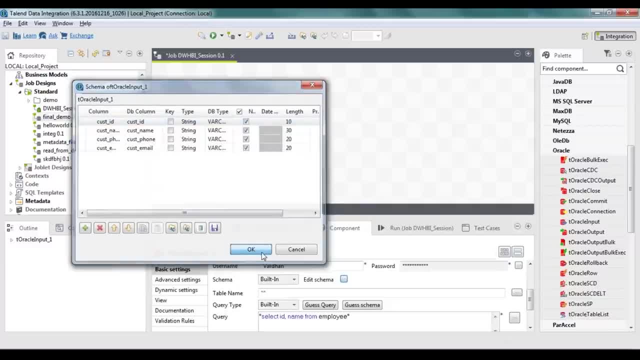 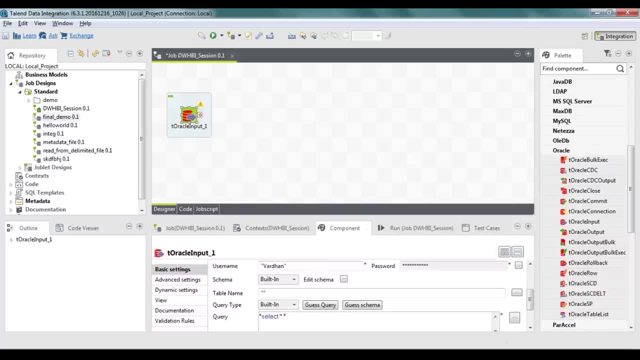 So I'm gonna set the length over here, Okay. Now what I'm gonna do is I need to set the default query, Okay. so I'm gonna say: select star from customers. Select star from customers. Okay, because customers is the name of the table. 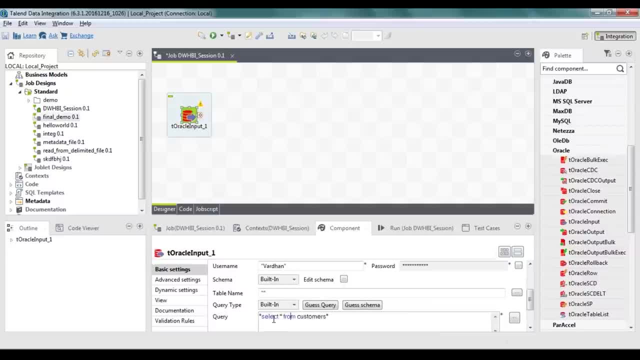 in my oracle database, right? So I'm gonna choose the table name here. I'm gonna say the table name here also. Okay, there's something I forgot earlier: You gotta mention the table name that you want to import from and you gotta specify the query you want to import. 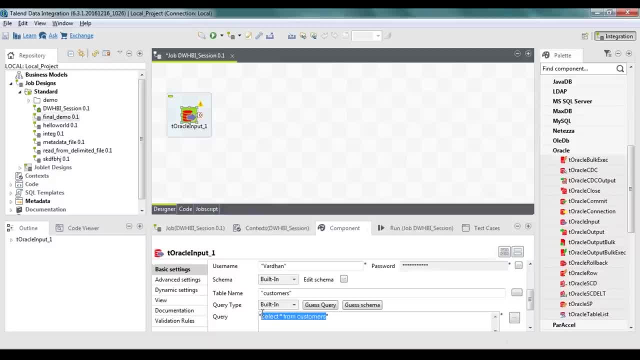 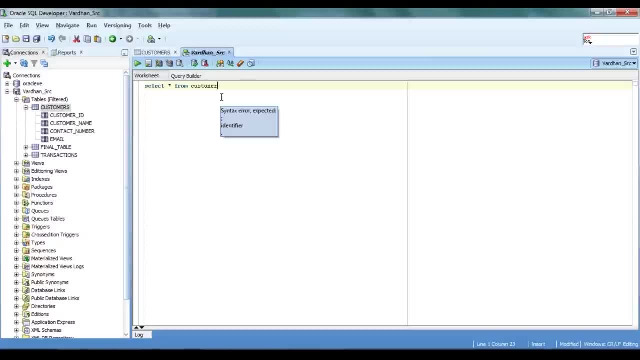 Okay, now let me run the same query in my oracle and let's see what details I get. So I'm gonna feed the same query here, okay? So it's gonna be select star from customers. So when I say this, I have this table option here, okay. 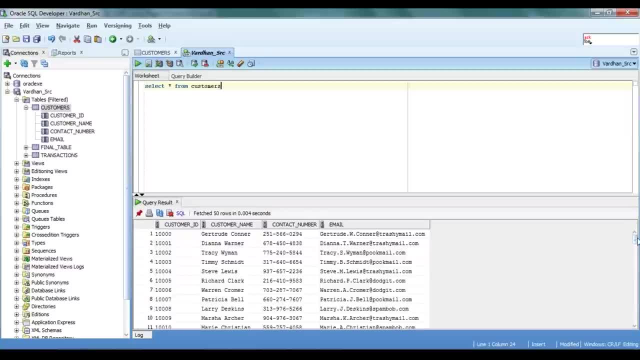 Now let me just run this query, okay? So I've got the same details in here also, right? So my table name is customers, So let me go to my talent and set that. It's set as customers, Customers already, and there's the same query. 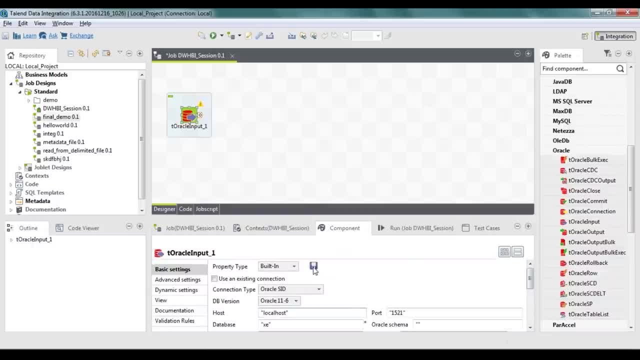 I'll be running here by default. Alright, I'm gonna save this. So I have set my first data in right, So I've got my customers data in here. So let me say another t oracle input and I'm gonna configure another input for my transactions table right. 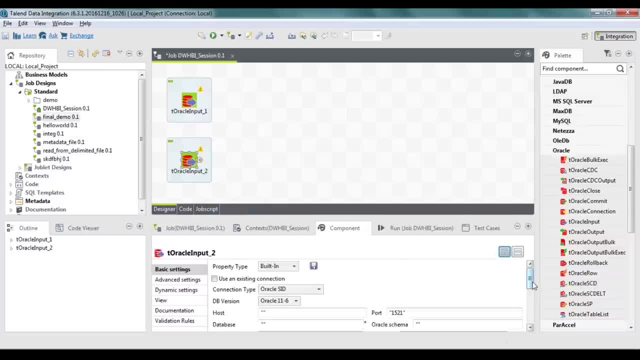 So I have another table for transactions, So let me set that also. And, as you can notice, every time you add a new input or configure a new output, then you'll have to add these details, right, You'll have to add the host name, database name. 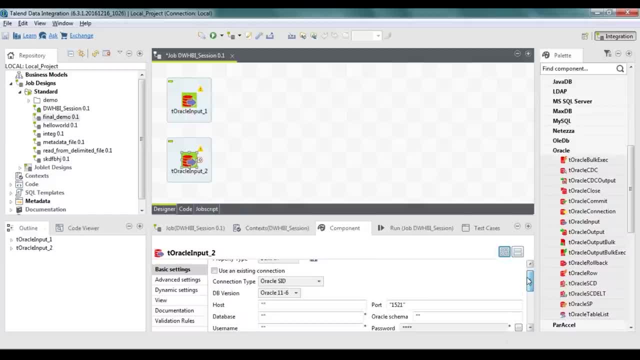 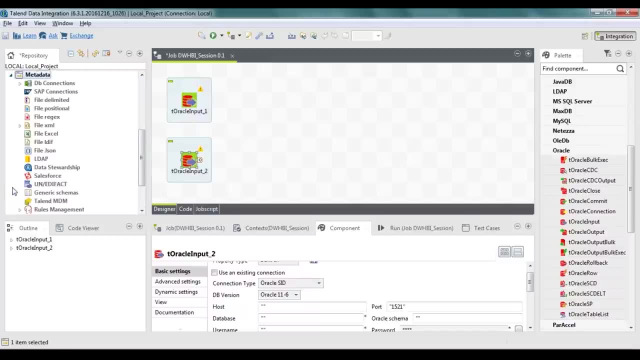 username, password and all these things. So instead of this, you have a shortcut here. So you have a shortcut with respect to metadata. So metadata is something that I explained earlier, right? So it basically contains data about your data. So under metadata tab, if you see, you have DB connections. 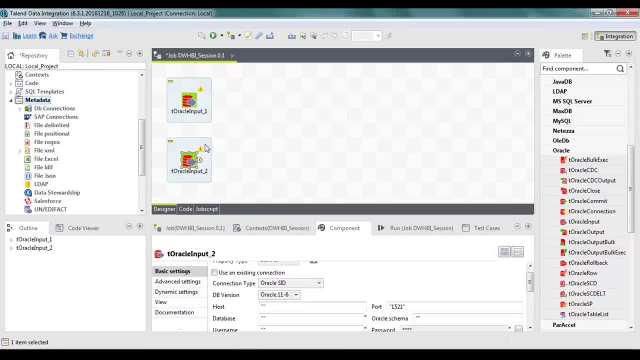 you have file all these things right. So if you want to create a standard input for data coming in from a particular database, then you can just set it once over here, okay? So under DB connections you can set one connection And it can be used in any number of jobs. 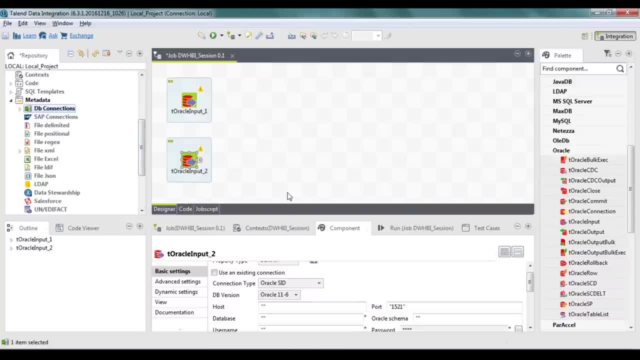 in this particular project. So instead of so this time, probably I'll have to anyways enter the details of this particular table. okay, But if I set the same thing through my metadata here, then I can use the same metadata every time I want to import data to my talent warehouse. 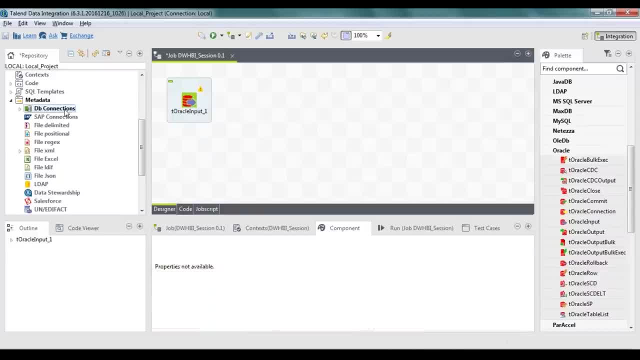 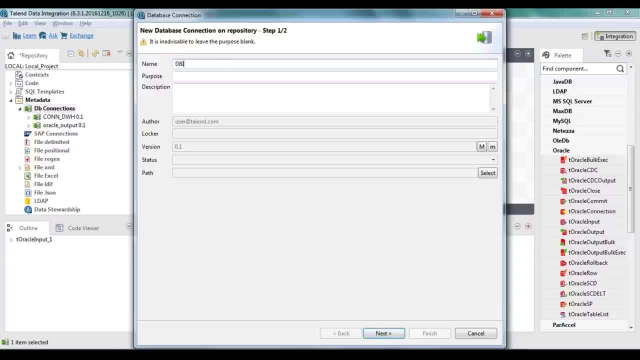 So what I'm gonna do is this time let me show you how to do it through metadata. I'm gonna say create connection. You wanna say the name of the connection is DB input. all right, Let's say database input. purpose: to get data from oracle. 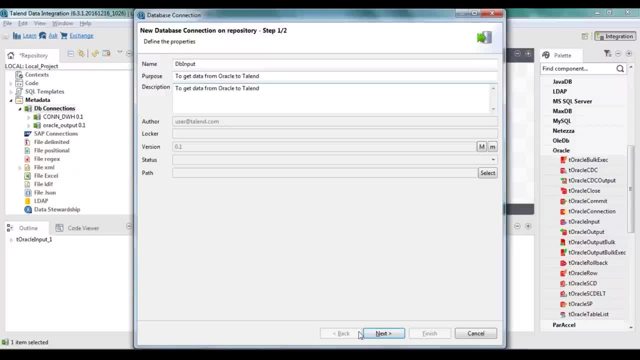 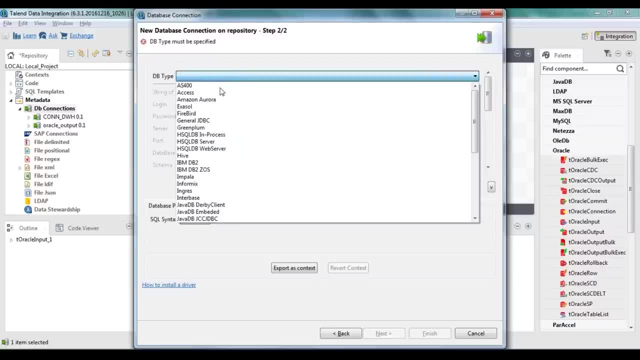 to talent. let's have the description also and say: finish. Okay, we gotta choose a database type over here. okay, Now the database type that I want to import is that of oracle, right, And I'm gonna do it with the help of oracle, with the service name. 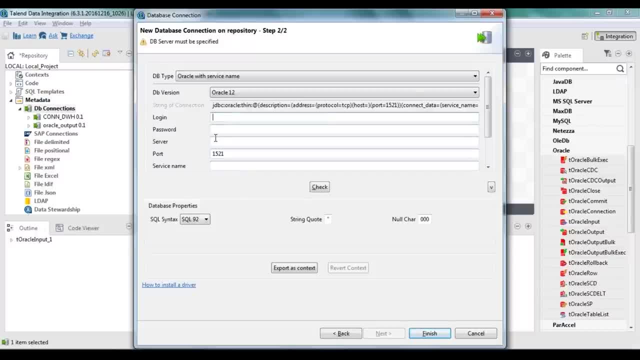 So when you choose that you have your login, you have your password and all these details. So, in place of your login, give you a username here. So in my case it's vardhan. okay, Password is this one. The server is localhost and the port is 1521.. 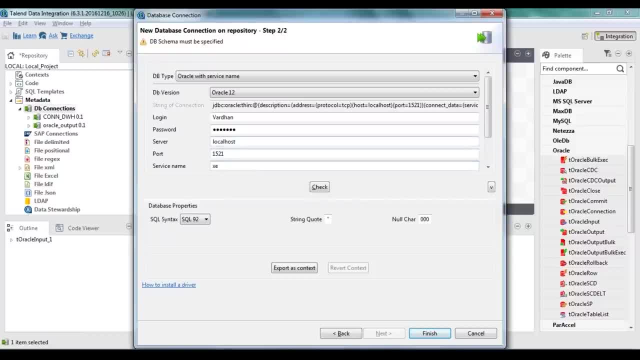 Server's name is xe. okay, Now to verify if the connection is correct, you can click on check over here. So, as you can see, the DB input connection successful message has come okay. This means that your talent is able to successfully communicate with your oracle, which is: 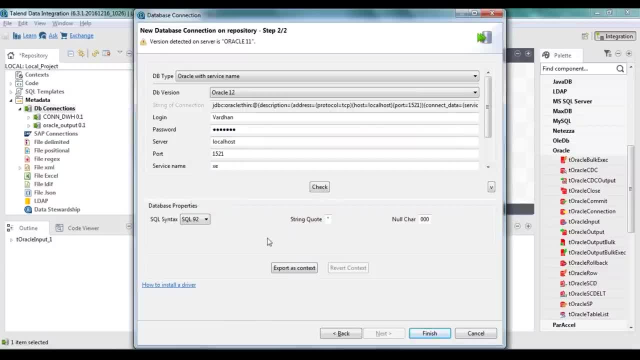 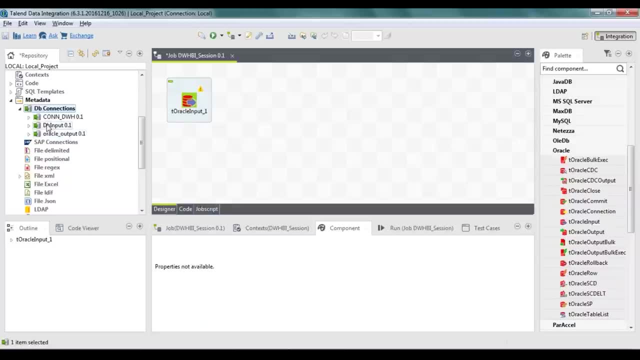 hosted on a port number: one, five, two, one, okay. so now that I have done this, I can now straight away say finish and add this metadata over here. okay, now I'm just gonna click on the drag and drop this DB input over here. when I do that, I 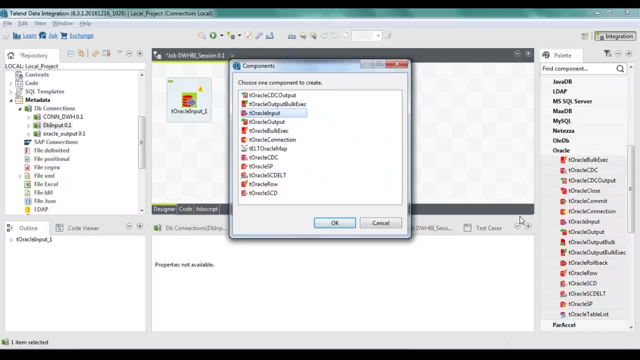 can choose this to be for either input or output or anything here, because under Oracle you have all these options right. so I have chosen this metadata for any of these options here. so if I want to use as input, I can do that also, if I want to use that output, I can do it even at that time. so I'm gonna say to your: 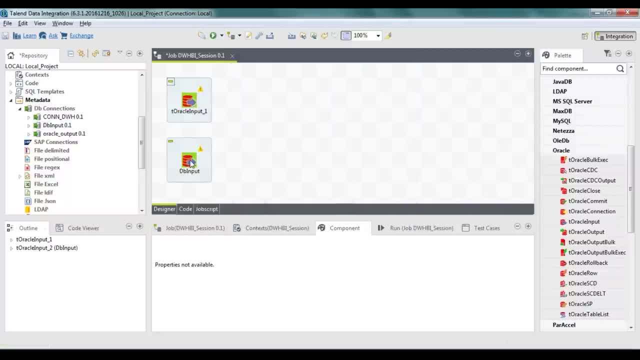 actual input and I'm gonna say, okay now, as you can see my DB input here, this is a metadata which has these properties already inbuilt. okay, so in case of this one, I had to give it manually. but here my metadata: I specified it once and it's. 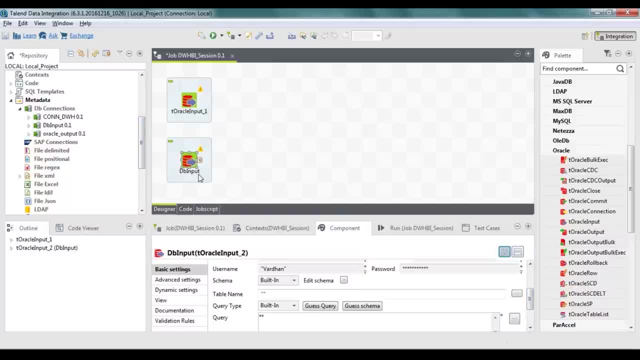 already replicated. so the advantage here is that even if there are 10 different tables from which you want to get data in, then you don't need to add 10 different database connections in your talent right when you're creating your metadata. if you create the database connection once and then, using that one time, you can establish 10. 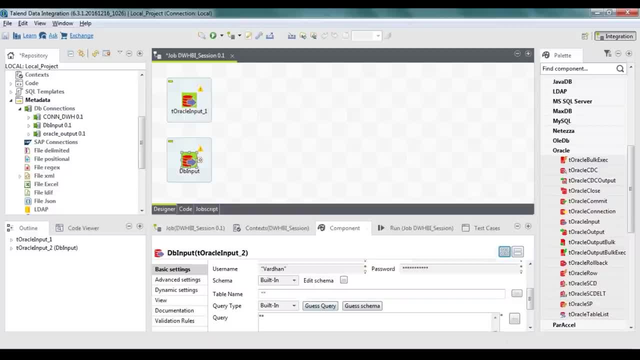 different connections. you can get it on from 10 different tables or replicate the same thing again and again. so that is the advantage here, right? so that's a thing. so next, let's give the table name here, okay? so the table is transactions table, right? so that's what I'm going to enter here. 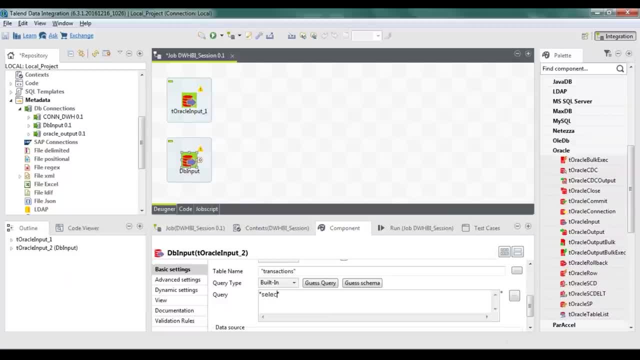 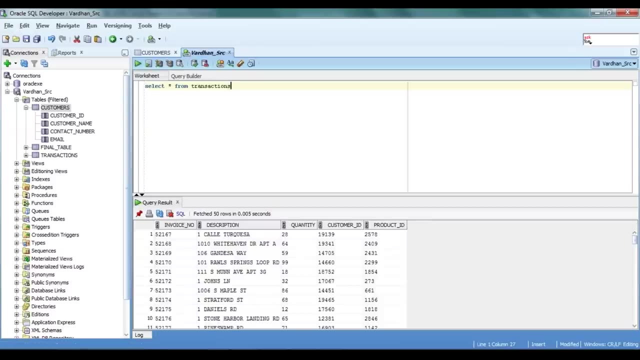 and the query that we have to run is: you select start from transactions. I will end this. transactions. okay, now let me also verify if this query is running in my my sequel developer. okay, and let me run this query. and yes, it's able to fetch data from my transactions table also. now going back to my talent, 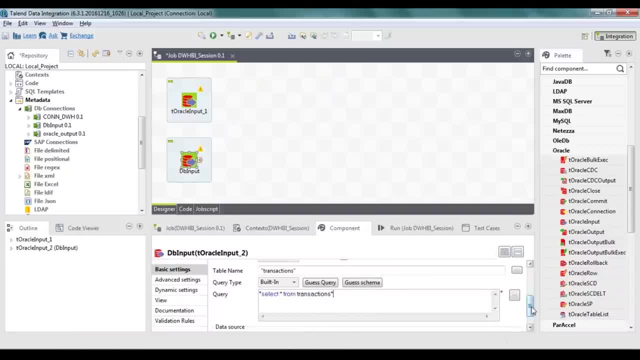 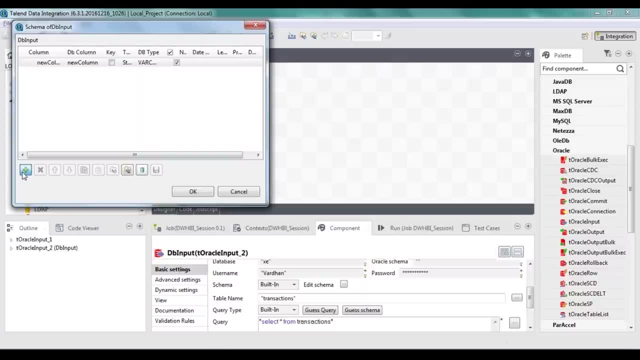 now that I've said this, let me go and edit my schema now. okay, so where do I have my schema option? okay, it's right here. so I'm gonna say edit schema and I'm gonna configure all the different columns and fields over here, if I'm not. 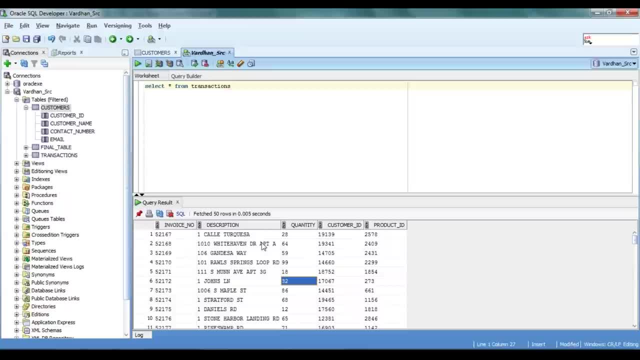 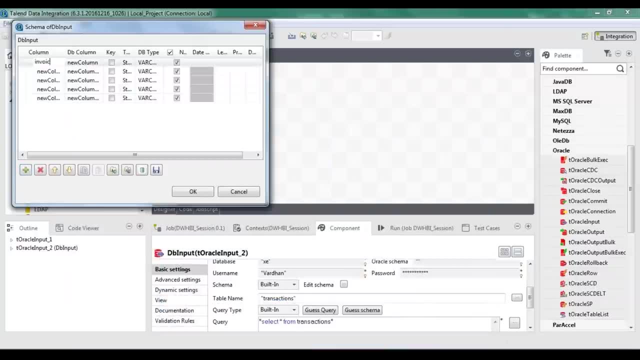 wrong. there are five different columns here: invoice number, description, quantity, customer ID and product- right. so I'm gonna rename everything here. I'm gonna say invoice number, description, quantity. what else do we have? we have customer ID and product ID, right, all right. so even the details here have been set to where care. okay, now this basically. 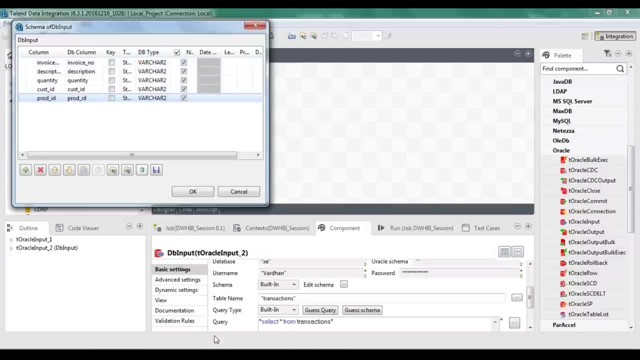 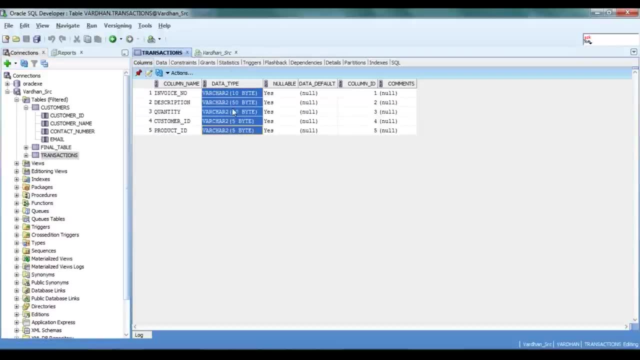 means that I'm getting the data from my database and the data type of that is where get right. so, as you can see from here, when I click on this, all my data, all the fields, have a varchar to read it type. so that's why I'm setting them. 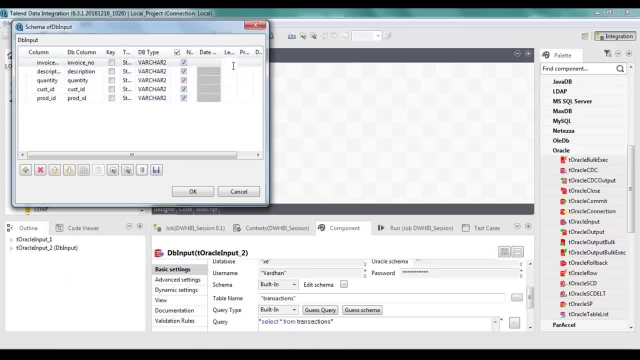 as varchar to over here, and I'm gonna set the default length for everything to be as well, not for everything. so for invoice number, let me give a length of 10. for description, I'm going to give a length of 100. for quantity, let's say 5. for customer ID, it's gonna be 10, and for 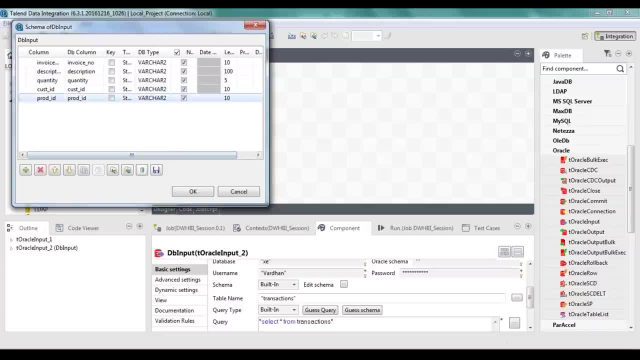 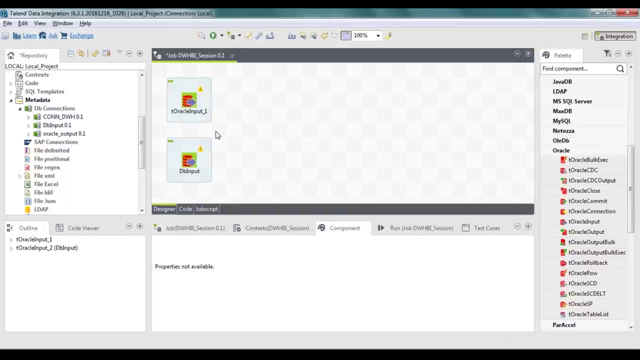 product ID. again, let me give a length of 10, so I want to say: okay, so my schema is basically set for both of these files. now what I've got to do is: now I have a configure, two inputs. now I have to get these inputs into my talent now to check. 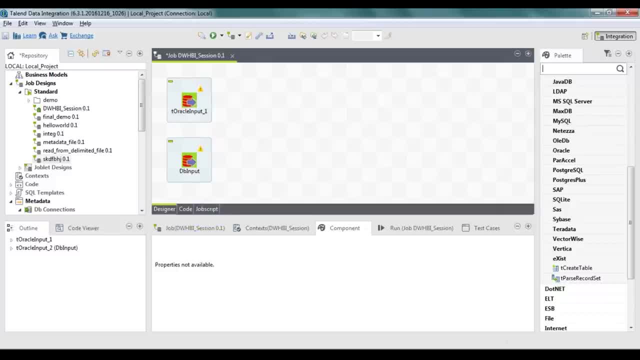 if my data is coming in from my data sources appropriately. let me just check the T log row, right? so the competent name is the T log row, but since I can't find it or I can also search for it here, so T log row, then I just put enter. I. 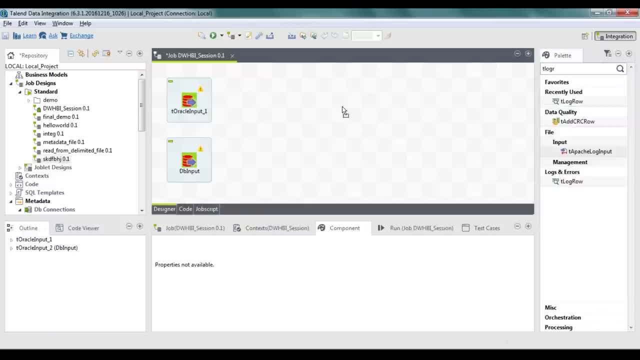 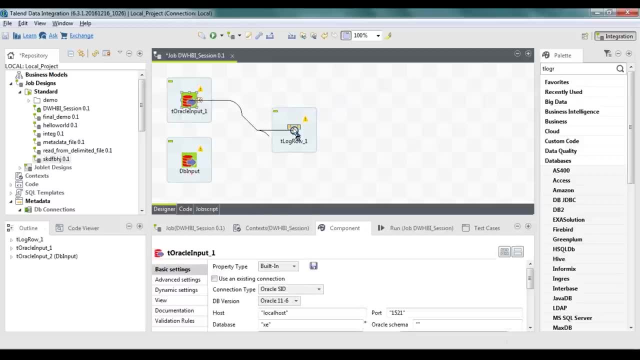 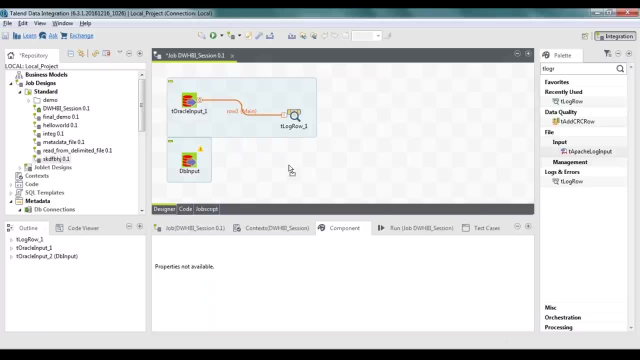 have these options, right. so just capture this T log row and drop it here. now you can create connections from here. you can say main and you can establish a connection over here. okay, and similarly I can use another T log row here. okay, drag it, I can paste it here and check. actually, no, I won't do that. so I can check if my 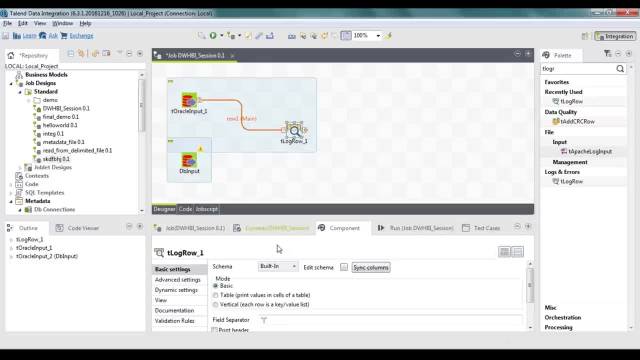 data is coming to my T log row from here, right, so my component is added over here. so let's say so. let's just check the schema ones. so, as you can see, these are the details that I'd entered in my source and it's already been mapped. 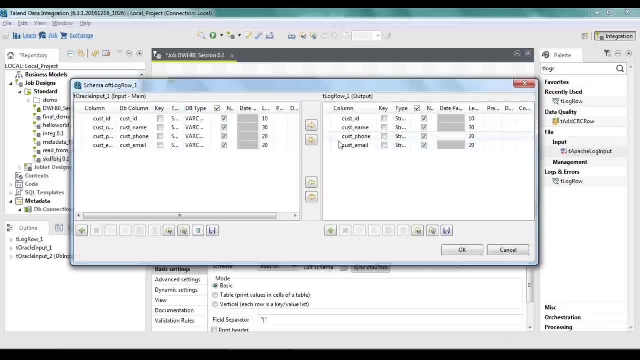 since I gave a connection between to bring my T log row and my input one. these fields are" have been mapped here also, so I'll be getting my customer ID, customer name, phone and my email details here. okay, now let me just stop. click on OK, go down and. 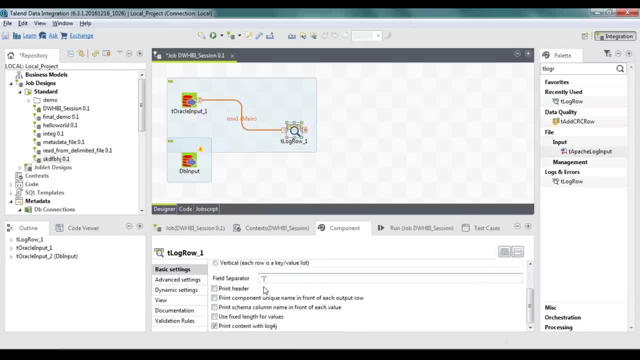 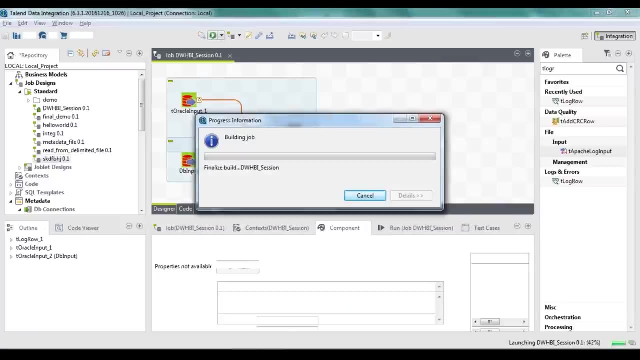 yeah, the free separator would be this pipeline. I'm gonna say: print header, print content with log4j. all right, so now let me just save this and let me run this. now you can see the button here right when I say run. it would build my job, basically, and it should be able to import my data from there, as you can see. 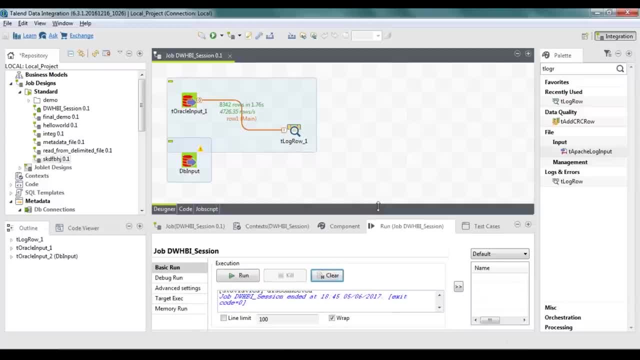 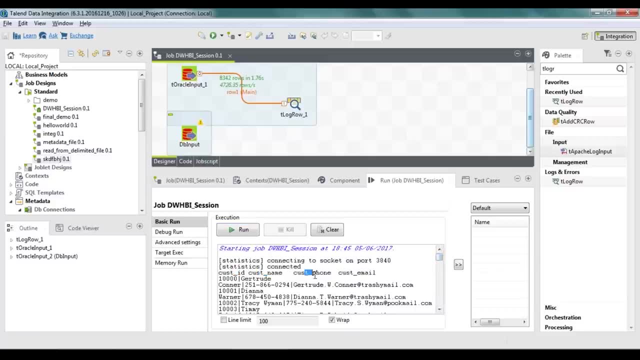 all my data is being imported to this. let me just minimize my screen so, as you can see, all my details are here, right? so? customer ID, customer name, customer phone and customer email- where the four different fields that I had configured to enter into my T log group from my input- and they have come. they have the 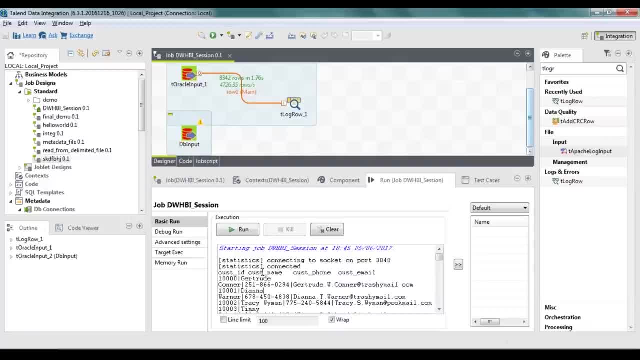 headers are these and the details are here. so for customer ID, it's thousand and the customer name is this one here and the customer name is this one here and the customer name is this one here, and then his phone number is right here, right? so this is his name here, this. 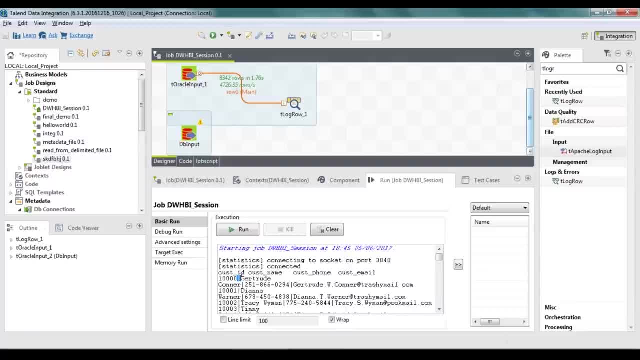 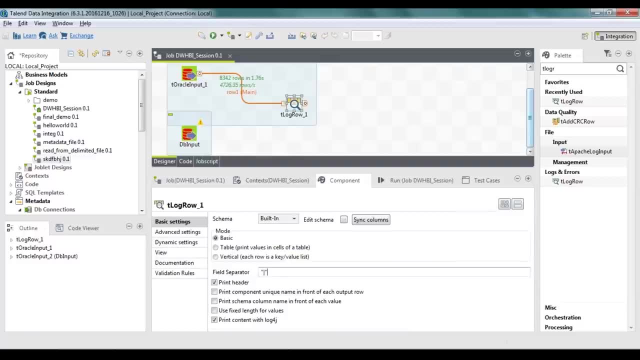 entire row and things like that. so each and every field is separated by a pipeline. so that's because I had in the component editor over here, because in the component editor over here I had set the field separator to be pipeline. okay, so that is the thing. so, since my component editor has a pipeline, so every 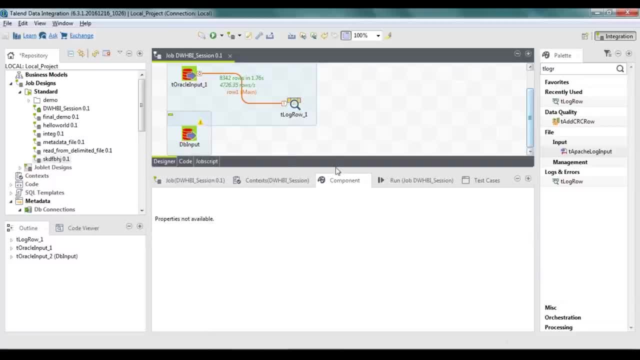 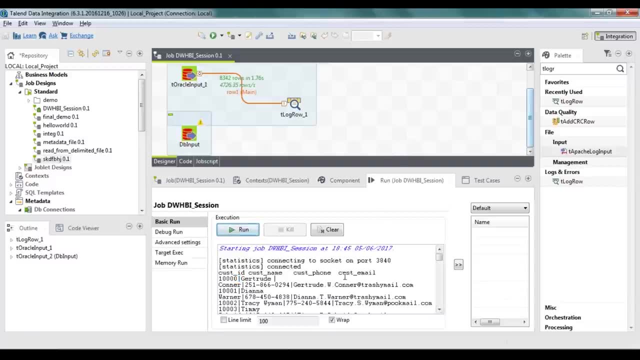 field in my data that is coming through my T log row. it has been separated by a field separator. that is pipeline. now, if I just go back here and, as you can see, by just clicking on run over here or over here, you can get your output. okay, this is, I've just done. 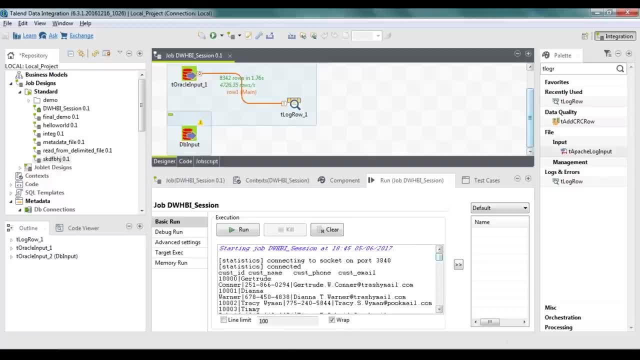 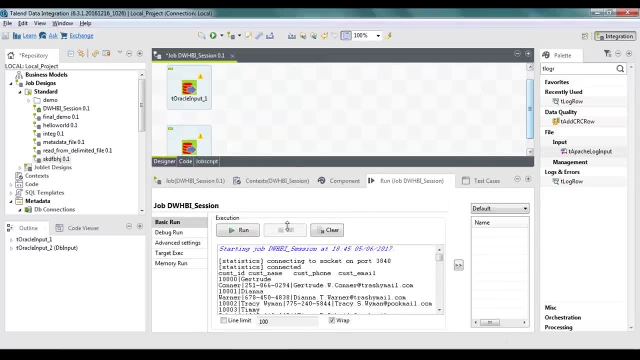 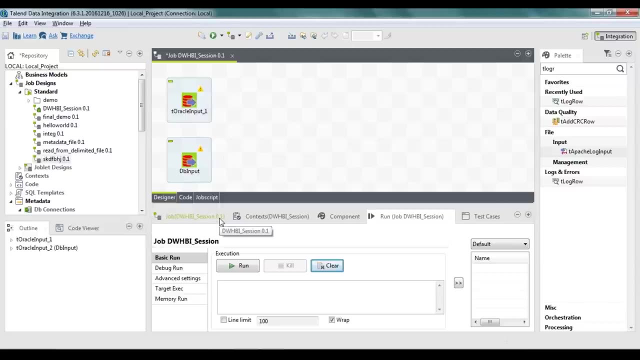 this to show you how data comes in. okay. so now that our data is coming in successfully, I'm just going to delete this T log row. okay, because we don't really need it for our demonstration. so you can just click on this clear here to clear your lock screen. so, now that we've established our connection, what we got? 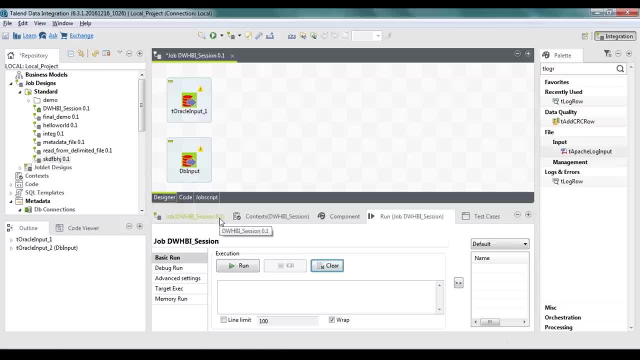 to do is we've got to merge this T log row and then we're going to go ahead and merge these two tables, right? so we've got to create a lookup field and I've got to make sure that my tables are joined, so for that we have another. 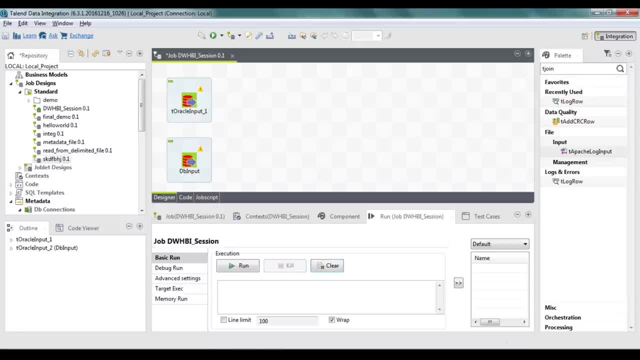 component, here called T join, and when you hit enter you have this right. so under processing you have this option of T join. so you can just drag and drop here, and what this would do is it basically join these two different inputs. so we have the source input of this one and this one right, so it would. 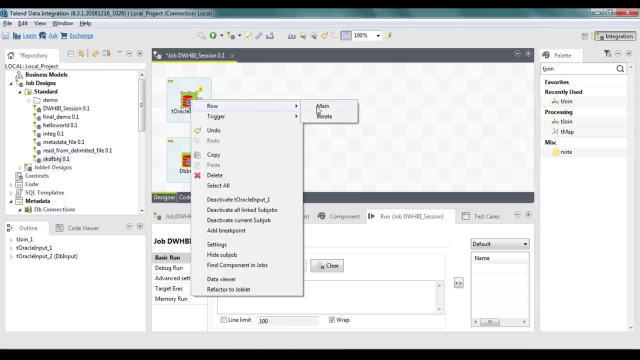 basically merge the two of them. so let's first create one link over here to my T join and similarly, let me create one over here from my input to to my T log. now, if you can see here, since this was the first connection that was established, this took up the name of main, okay, and 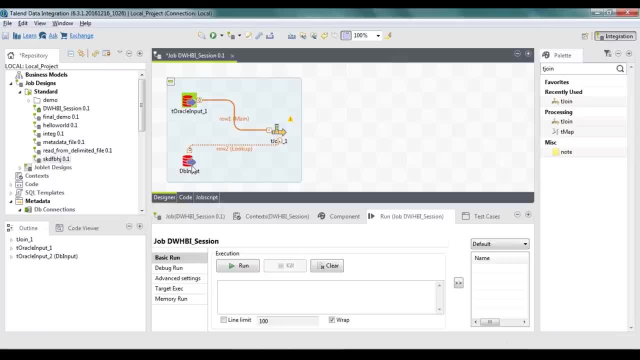 my second connection took up the name of lookup. now, that's because this table here, this will look up to the customer ID field in this table and match the subsequent rows or entities with this particular columns right. so what this lookup would do is it would use the customer ID field in my 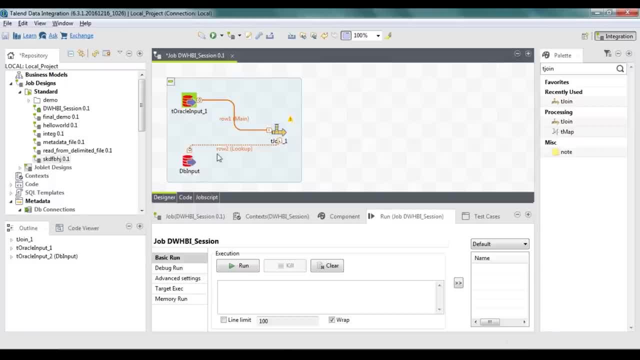 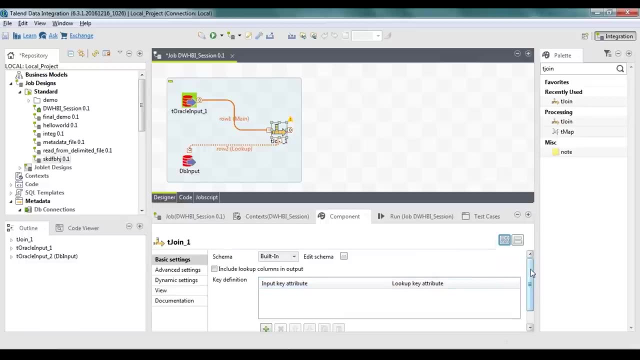 in this table and it would do a look up to this particular table and match the remaining rows and columns right. so let's configure the schema for that. first of all, since we are joining these two, we are using this T joiner. okay, so T join. let's go to the component and edit all the other details here. so we have to. 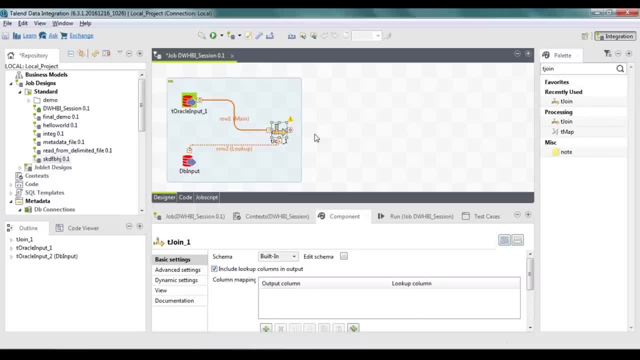 check this include lookup columns and output. this means that the output that comes out of this joint, we want to also include the fields which are present in my lookup field, right? so that's why I've checked this column. so, besides that, here it says column mapping- right? so we have to always map these two. 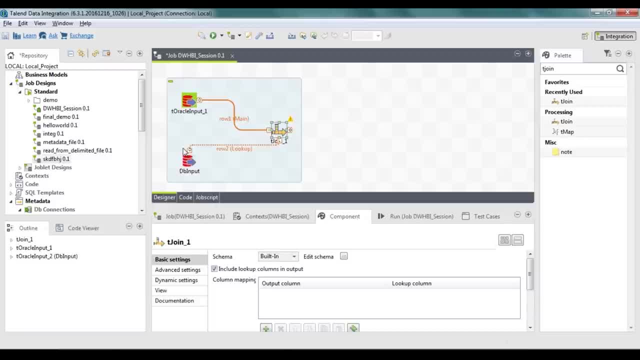 different tables using one lookup field. right, so it's either one lookup field or the primary key, foreign key relationship. so both are the same. so that's what we were to define. here we go to define which is the parameter, which is the foreign key, or which is the lookup or failure. okay, so first of all, let's go to 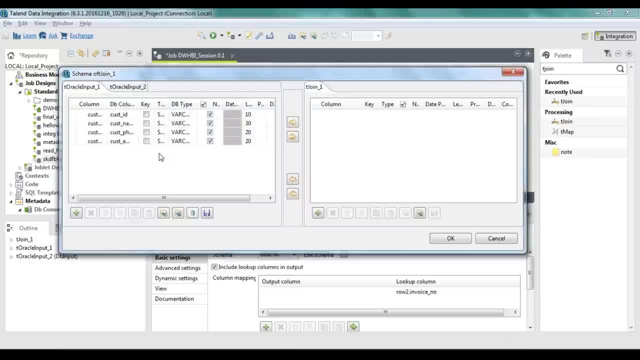 edit the schema here, all right, so we have the two different fields here. we have the input field one and the input field two over here. so let's add all of these. I'm gonna say control a and I'm gonna move it here. all right, so I'm. 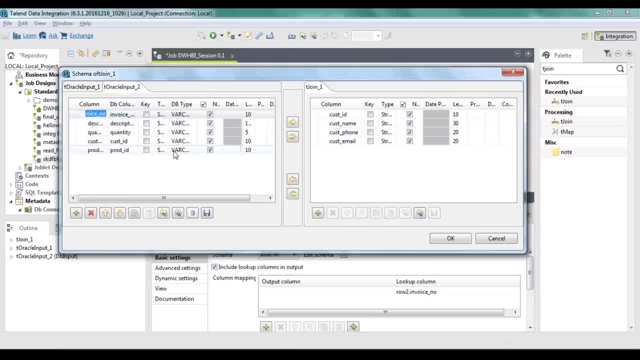 gonna join all these things and from the second table I'm gonna move my invoice number, my description. well, I don't want to move description, so I'm gonna move my quantity. customer ID is already there, so I would then want to move my product ID. okay, now, the reason I'm not moving description is because I don't need a. 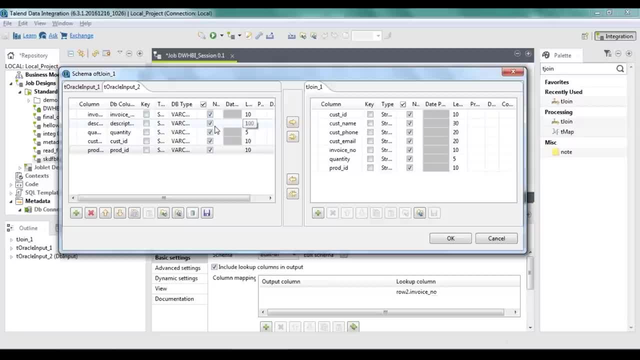 description. as per my problem statement, there's no need for our description. okay. similarly, even product ID is not really needed for me, so I can actually remove this also. right, so I have these. so these will basically be my output fields: my customer ID: customer name, customer phone, customer email address, invoice number: 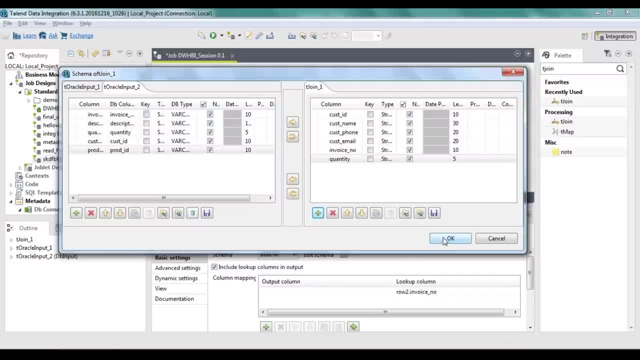 and quantity right. so these will be my output fields and another up set my schema. even the length has been auto picked, right. so this is the nice thing about this is that it's very simple and it's very transparent. things are pretty simple and it's all straightforward so you can just click on, okay. so guys are. 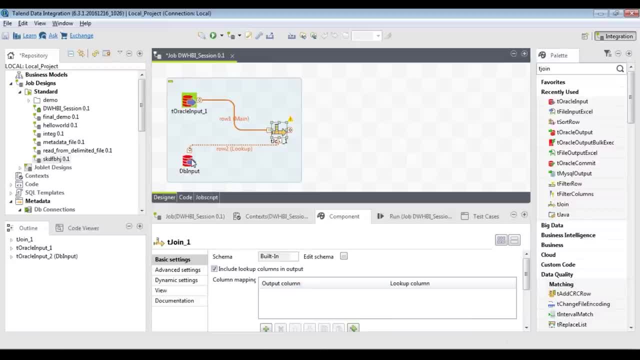 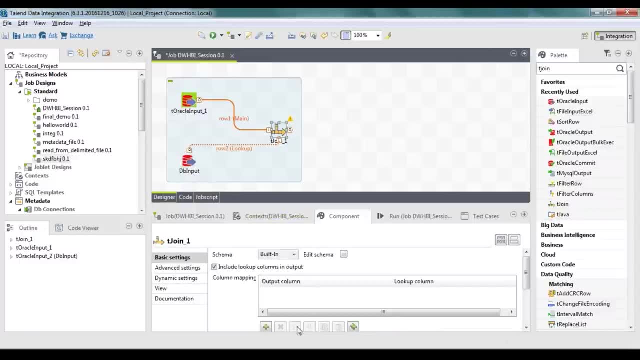 now that we've set a schema here, let's add the columns that we want in our output from our lookup table. okay, so this is a lookup table and from here what all columns would be? what do we want in our output, so that we've got to? 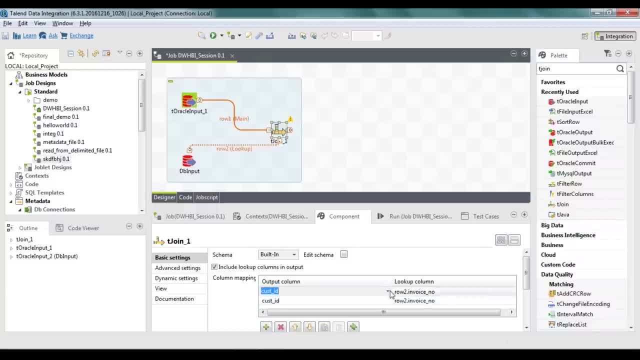 include over here, right so let me add the different entries. so I really want my customer ID to be there, so I'm gonna say: row 2, dot customer ID, row 2 here, right so? and then I want my quantity to come and that I'm gonna set it as row 2. 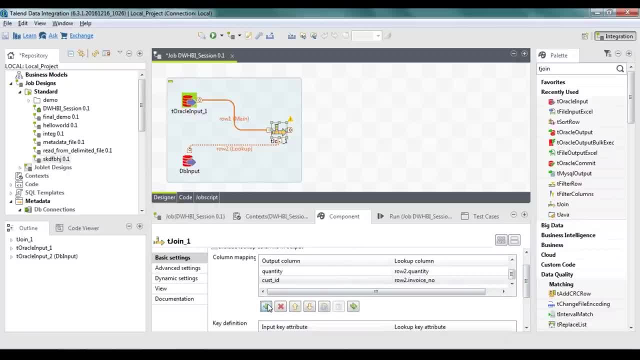 dot quantity. I'm gonna add another entry here and that's gonna be for invoice number. okay, so I'm gonna say this is row 2 dot invoice number. all right, so now that we've done our column mapping here, this is pretty good enough. now let's go. 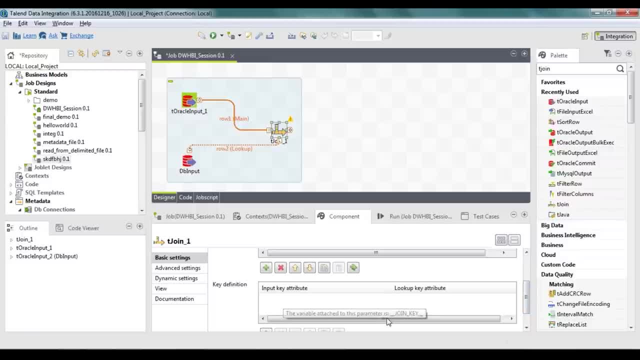 down and set our key definition. so here we set our primary key and secondary key, foreign key definition. okay, so let me add an entry here. so the primary key is going to be customer ID and the lookup table is going to be row 2 dot customer ID. okay, so with the help of these two fields we're going to find 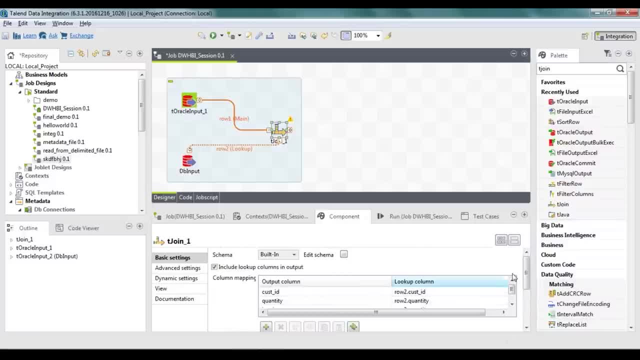 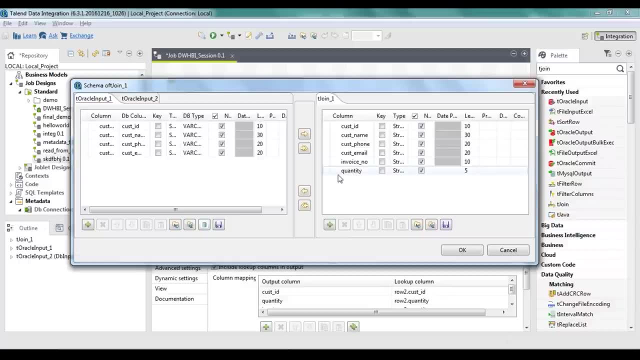 our. we're going to make our do our lookup. and another advantage here is that I can also go back to schema and edit the data type of my quantity. okay, since I'll be using quantity as my differentiator for my problem statement, I can set the data type to. 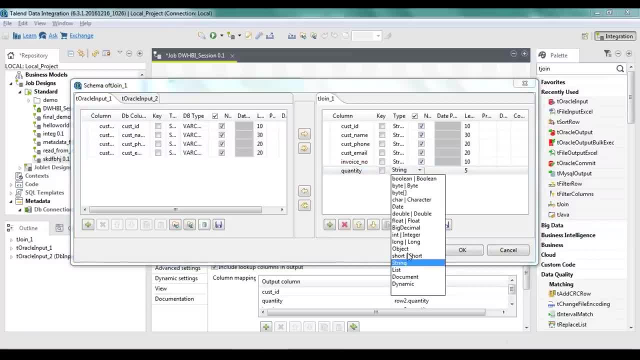 be something else. I can set it to be integer. okay, so I can do this and set the length to be either 5 or 10. right, I can give okay. so now this basically means that, or even though all these are in string format, my quantity can be an. 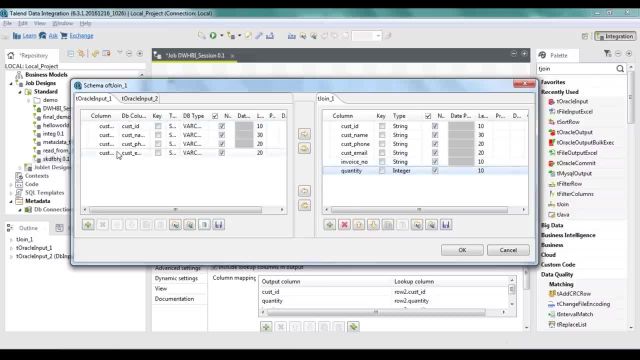 integer and the best part about talent is I don't need to change anything over here. okay, so I can get the data, and from any data type, the data that comes in can be of any data type. okay, but the data that I store, all the data that I finally export, that I can change the data type of that. 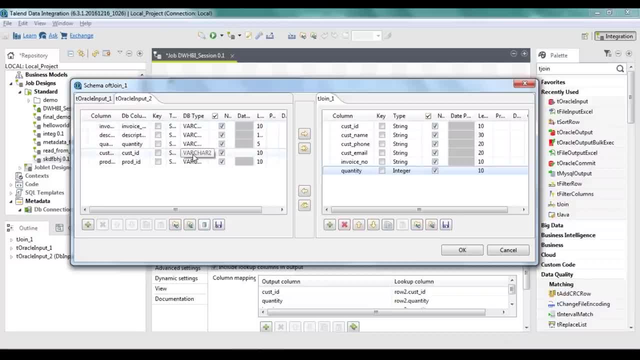 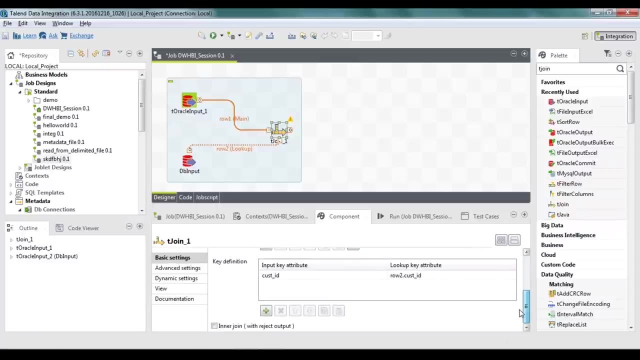 particular data. so that's the advantage. so quantity comes in the form of varchar to data type and I'm converting it into integer from inside talent, right? so that's the thing about advantage with talent. so I'm just going to say, okay, now, alright. so now that I've done this, I think I'm done everything with respect. 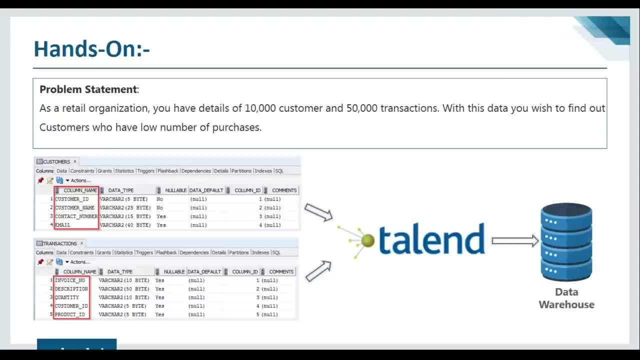 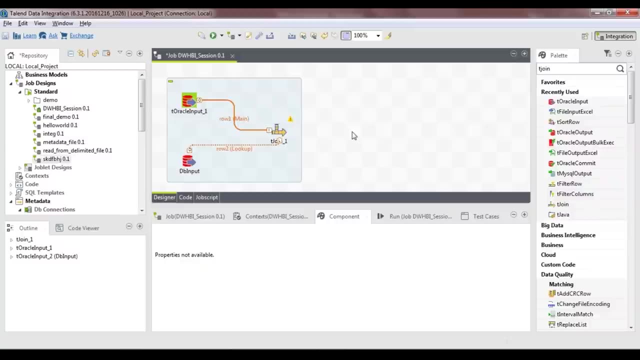 to T join. okay, so now let's go back to my problem statement for a minute now. what they say is: they wish to find out only those customers who have a low number of purchases. okay, so it is quantity which defines how many purchases that they have, right? so I'm gonna go back to my talent here now that 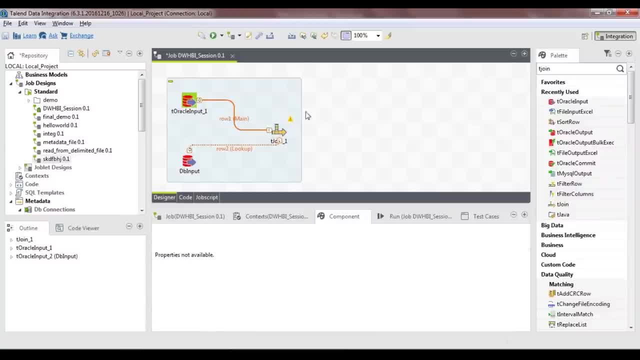 I've added my T login over here. I will be getting all my details and all my data into this component, right? so my input one would be giving me those rows from customers and this would be giving me those rows and fields and records from my transaction table. so I would be getting approximately 50,000 rows from here and 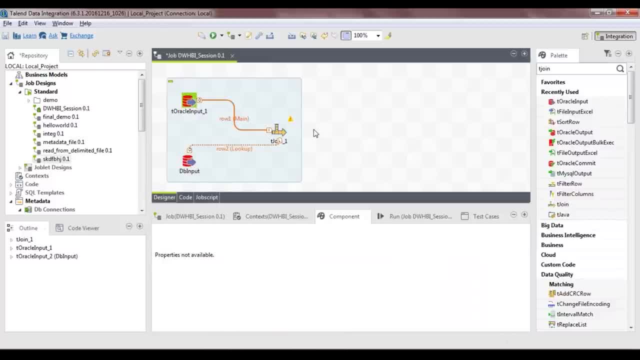 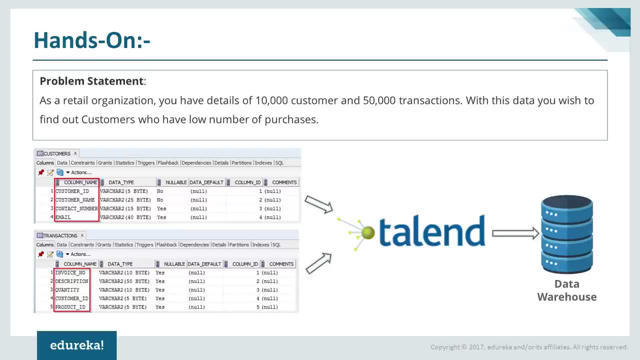 10,000 rows from here. now that I have all these rows over here, what I have to do is I have to filter them based on the quantity, and our problem statement here says that we have to find out those customers who have a low number of. 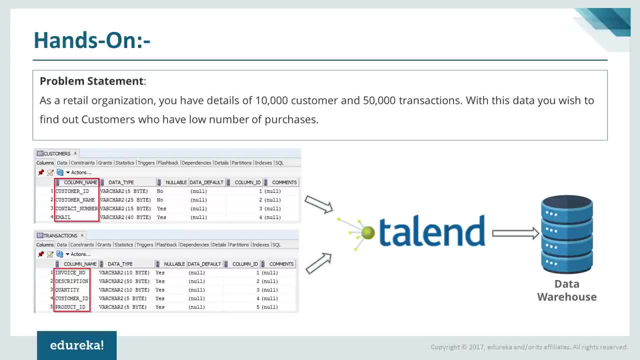 purchases and, if you remember, we defined that when. if you want to find the low number of purchases, it's not exactly defined. so let's say we want to find those people who have less than 10 transactions, or whose quantity is less than 10, all right, who purchased less than 10. 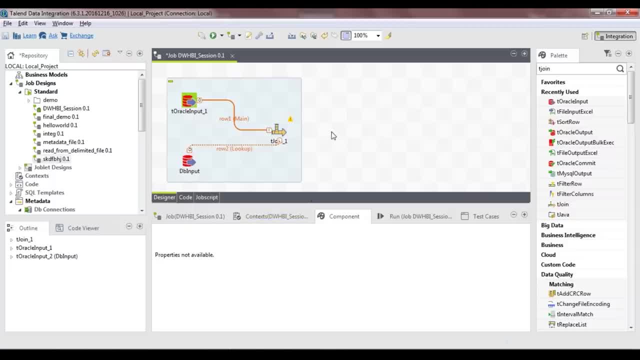 items. so for that, we can just go back to our data warehouse and create another filter or component here which would filter out those people who have less than who have purchased less than 10 items per transaction, right, so for that, let's again go back to my pallet here and search for this component filter. 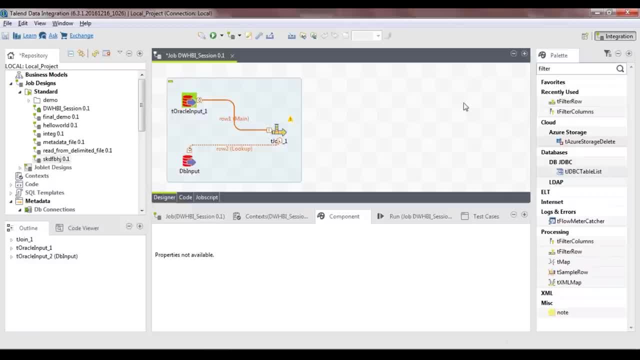 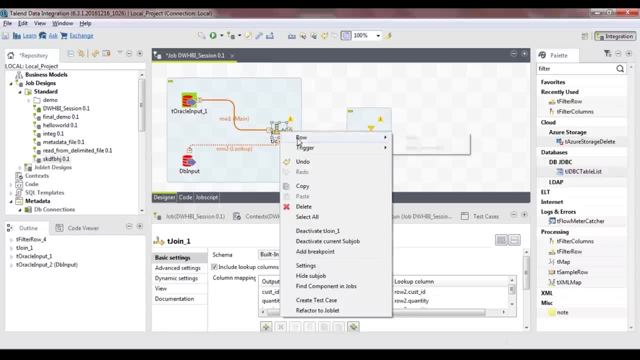 so, as you can see, there is T filter row and T filter columns- okay, but I want to filter rows, so I'm just gonna drag this one, drop it here. so T log filter- okay, and I want to connect these two right. so I'm gonna give a connection here and what I'm. 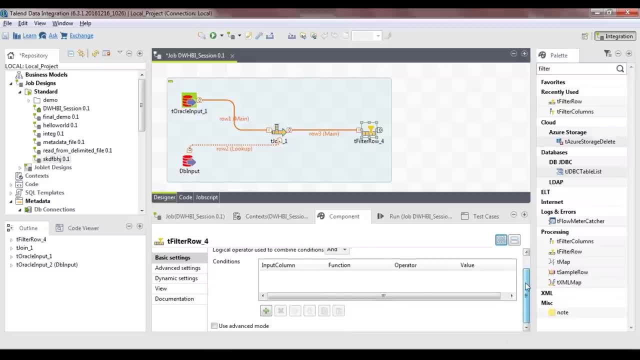 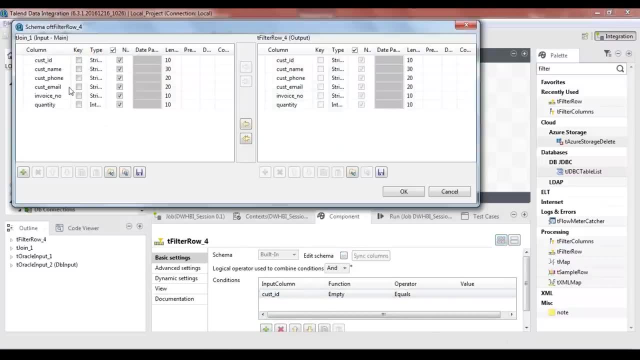 gonna do here is I'm going to define the, the filter criteria. okay, so I'm gonna add an entry here, but before that, let me go to my schema and, as you can see, I have all these entries here and the same fields are here also, right, and even the 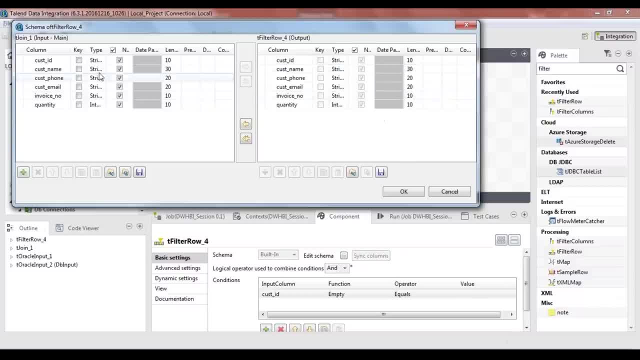 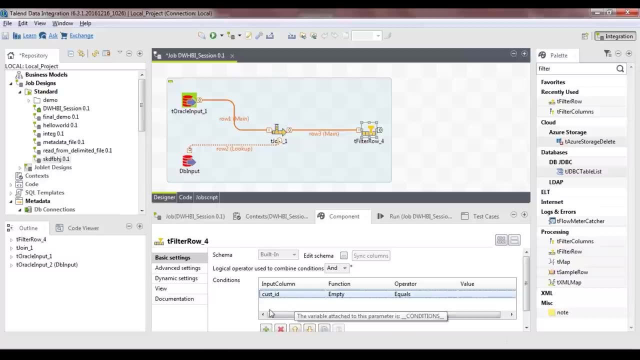 data type hasn't picked up by default, and that's the talents functionality. so this will be the input that will come to my filter and this will be the output. that will go right. so let's just click on OK. and now, coming to my criteria for filtering, I want to filter my quantity, right, so the input column- 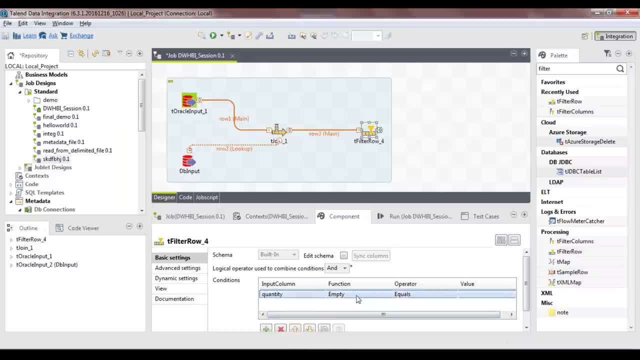 that I want to check is that of quantity. okay, and the function that I would want to do is empty. now for now, let's just leave it empty, and the operator is if it's lower than or equal to right. so if it's lower than or equal to 10, that is. 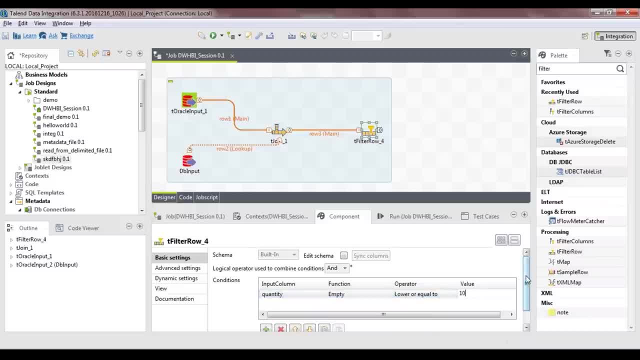 the value that is present in this column. if it's less than or equal to 10, then I want to filter only those rows and I want to send only them. okay, so basically my command is also set over here. alright, so even my schema and my function is set. 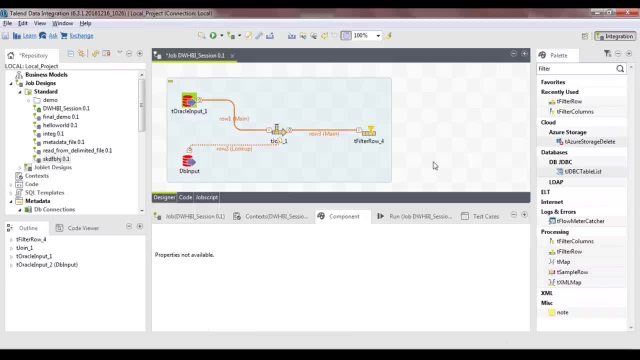 over here and now what I have to do is I have to set the output for my data warehouse. okay, now where do I want to extract these results and store with these this data warehouse? alright, so let's say I want to store it in an external data warehouse and I want to store it in an external data warehouse. 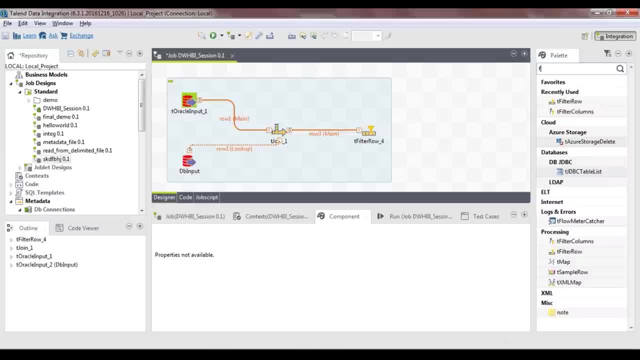 alright, so let's say I want to store it in an external data warehouse and I want to. then I have to just go back to files over here. let me just type file and hit enter, and I have these options right now: T- file input Excel. T- file output Excel. 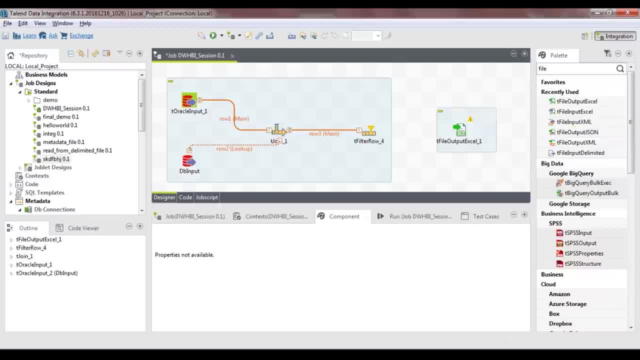 so I'm going to choose the file output, Excel, and drop it here. this would essentially mean that the results that are filtered over here in this component, this would come and get stored in this excel file which I'm going to create now. okay, so let me connect these two. also, I'm going to say 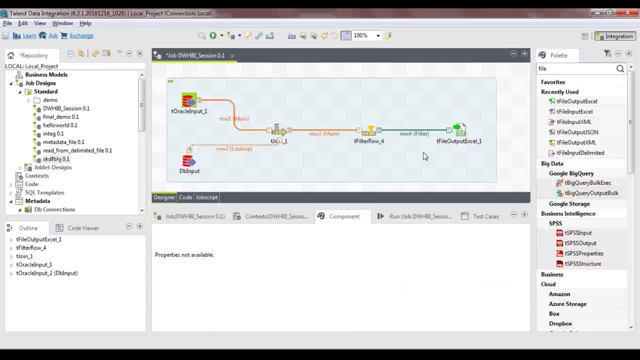 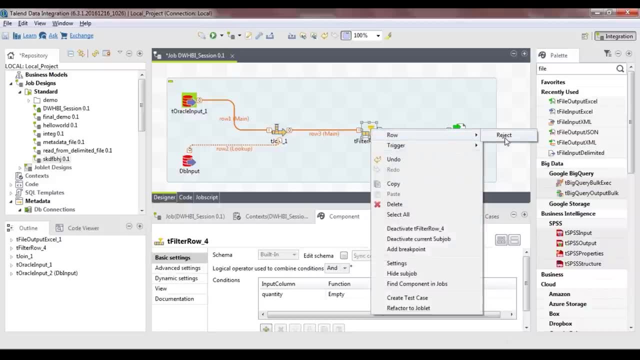 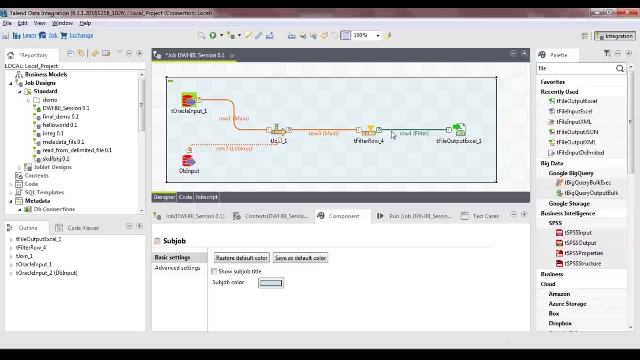 filter and put it here. and, supposing, if I want to also get a list of all those people who have more than 10 transactions, then I can do that also by using this option of reject. so whichever rows get rejected, right. whichever get rejected, from moving to this particular file, those can go to another file, right. 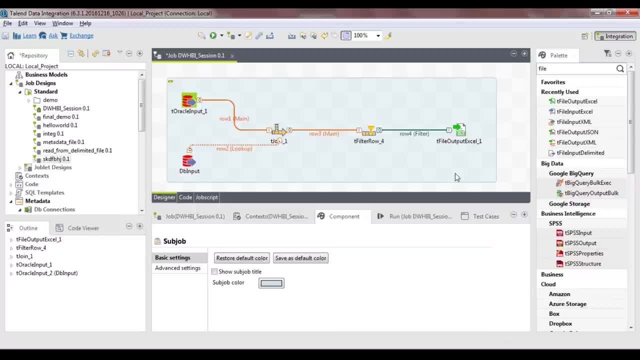 so we have that functionality also, that I'll show you even that, but before that. so let me just show you how this looks like. so I've said row filter T, file output Excel, and let me edit the component over here and let's say the file name is this one. 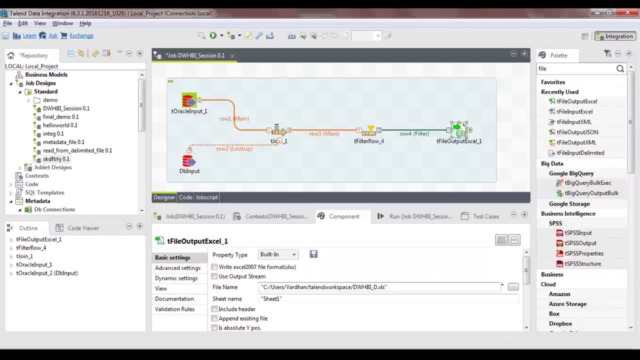 DWH BI demo. all right, I'm gonna say include the header. so header basically is the part which would say customer ID, phone number and all those things. so I'm going to say include header, all right. and I'm gonna say define all columns to auto size, that's just to auto size those columns, right? so 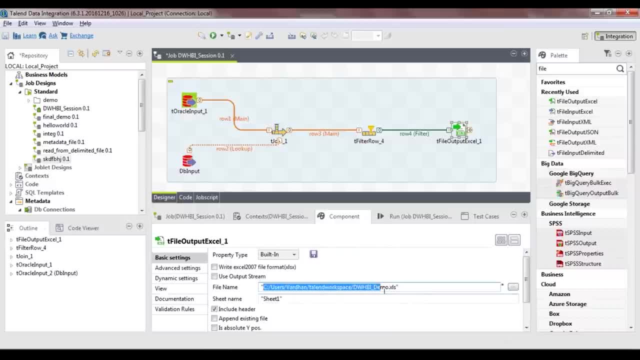 it's all fine. now everything is set and my file would be saved in this particular path. okay, and this would be the name of my file, which would be stored when I run this. so I've copied this path. now what I've got to do is I need to save this job and execute. 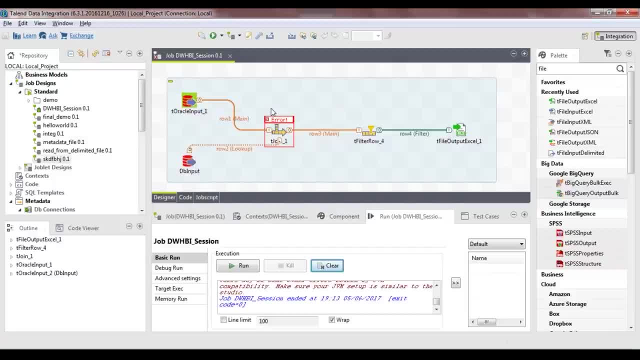 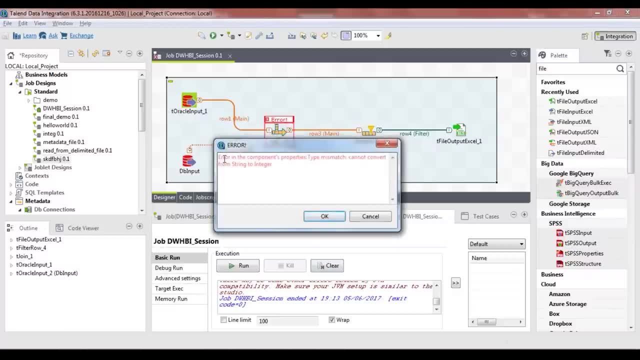 this. okay, when I executed that, it's showing me an error over here. okay, so the error? it shows us that the error in the competence properties type mismatch cannot convert from string to integer, so I need to cut this out. okay, not a big deal, I can fix this error. 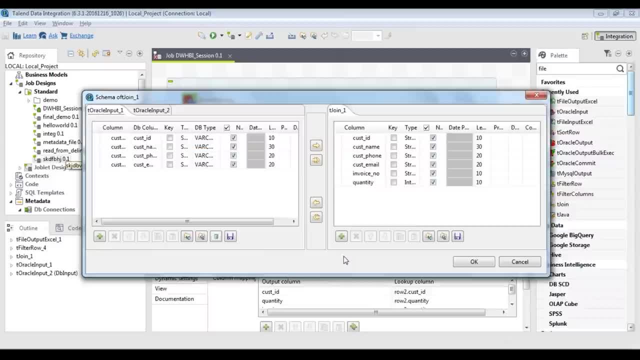 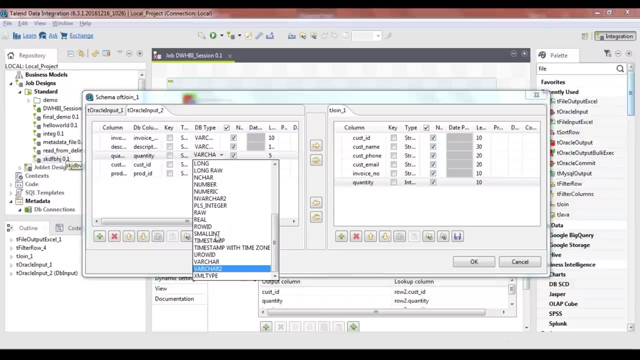 okay, we can fix that by first of all checking our schema right over here. if you see the schema here, it says quantity is type integer. right, but over here quantity is still type spring. so that is what we need to change. we got to change the type over here to integer. so I'm gonna say number and I'm gonna click on. 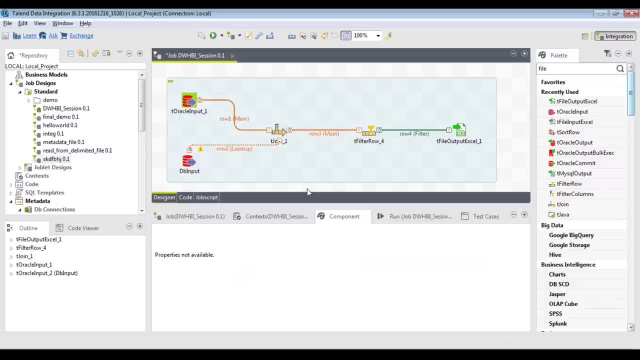 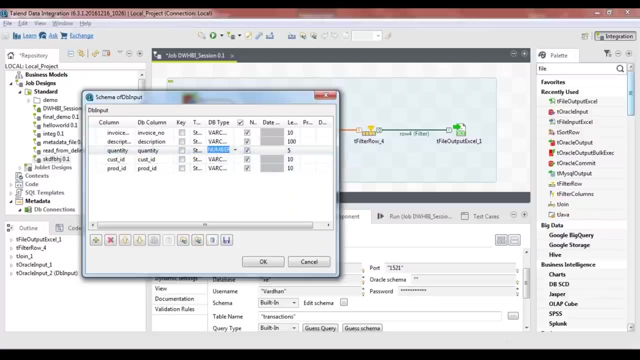 Okay, fine, Okay, so now let's go back to this file, right, And let me edit the schema and set the properties correctly. Okay, so it's not able to convert this right? So the type of string and the DB type is number. 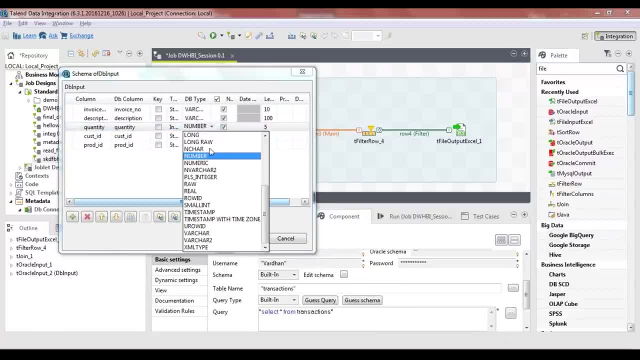 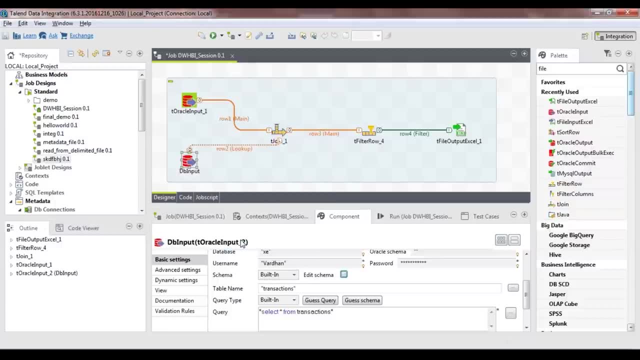 so this is the problem. So I can change this also to integer, right? So integer is right here, so I'm gonna choose this as integer database type. I'm gonna click on, okay, And now let me go back to the t-log: join. 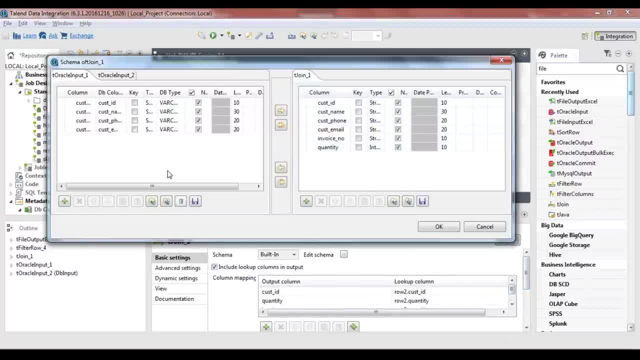 and check the schema over here. Okay, so this is my table and quantity. This is integer. this is also integer. it's coming here and now it'll get converted over here into this, So now it shouldn't idly throw me any error. 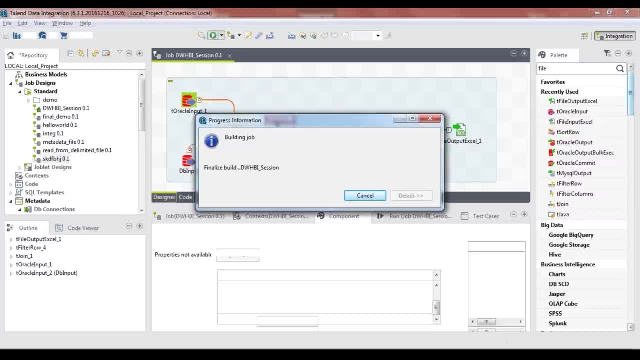 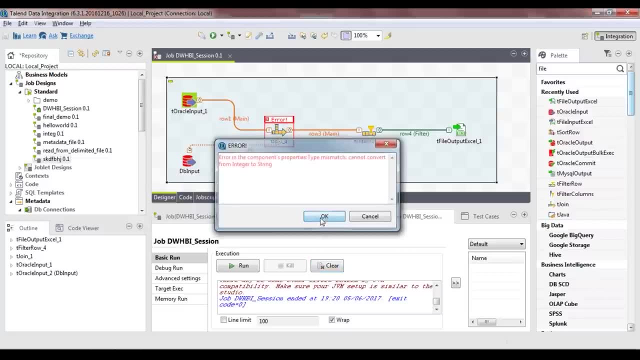 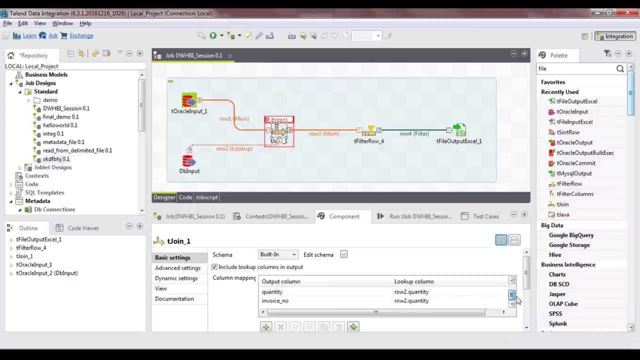 Now let me just save this and run this job. Okay, building job. Okay, it's showing an error again. It cannot convert integer to string. Okay, so let's see what the error is now. Okay, so we have a problem here. 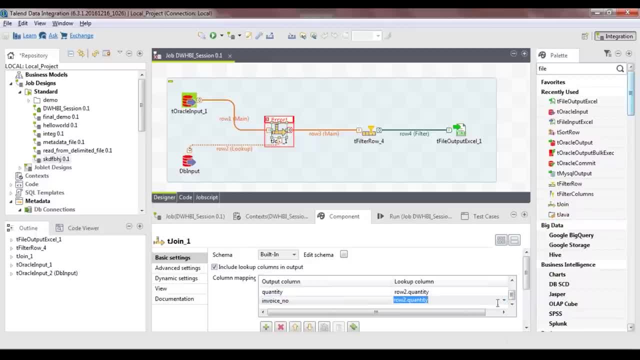 Invoice number: right. So this is the problem. So invoice number: it should be row two, dot invoice number. So this was the type mismatch error that we were getting Right, so no problem. Okay, so again it's changing right. 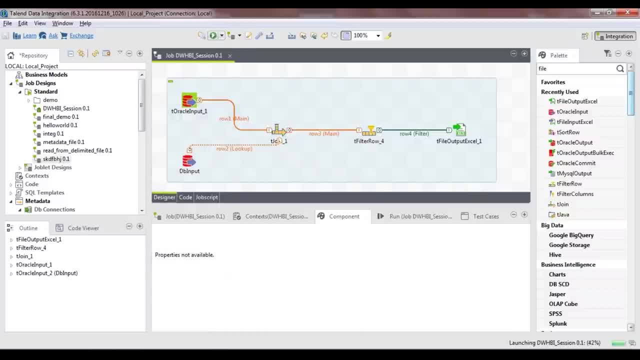 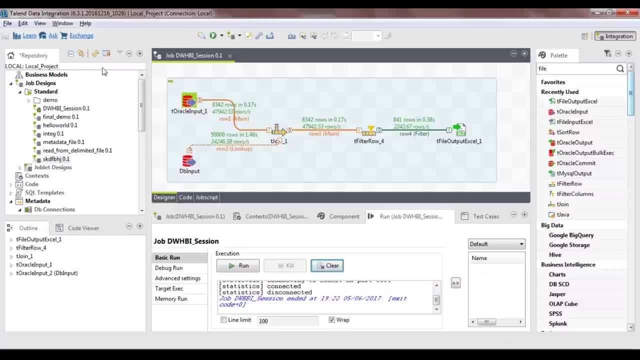 All right, I'm gonna save this now And we wouldn't have the type mismatch error now. Okay, great, So it says connected and disconnected. As you can see the output over here, we've got around these many rows from this table. 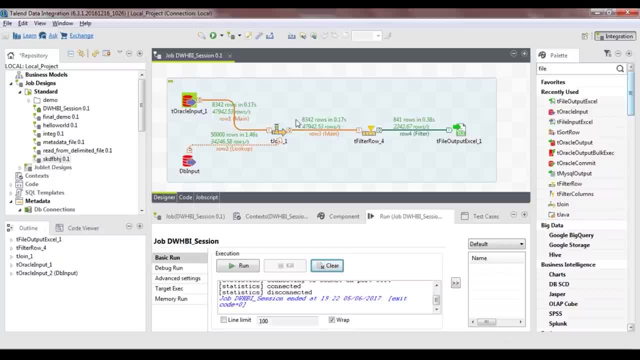 and about 50,000 rows from the table here And we've got it here and then we would have probably joined these two with the help of the customer ID field And then to my t-log row. it would have filtered all the fields. 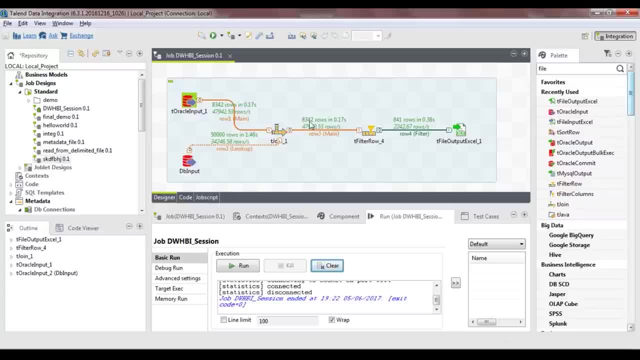 So we've got. the input has basically been 8342. number of rows: 8342 rows, out of which 841 rows got filtered and stored in this Excel file. Awesome, right? So let's just go to this path and check if our field contents are correct. 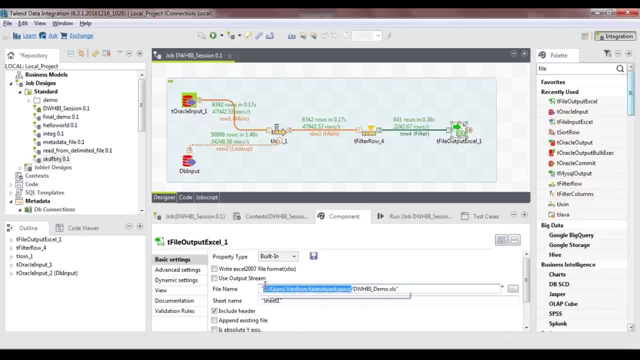 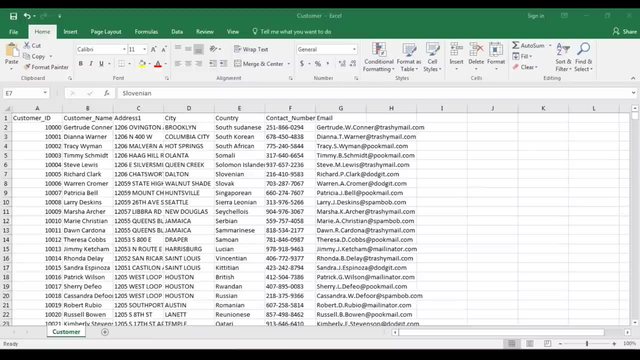 So this is the path where the file is stored, right? So I'm gonna copy this path. I'm gonna go back here and paste this path. So this was the file that we created, right? And yes, As you can see, we've got customer ID, customer name. 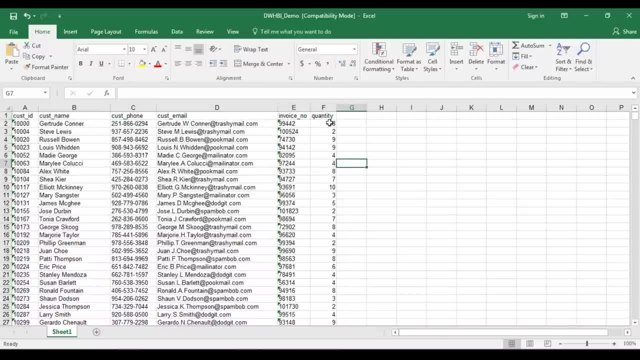 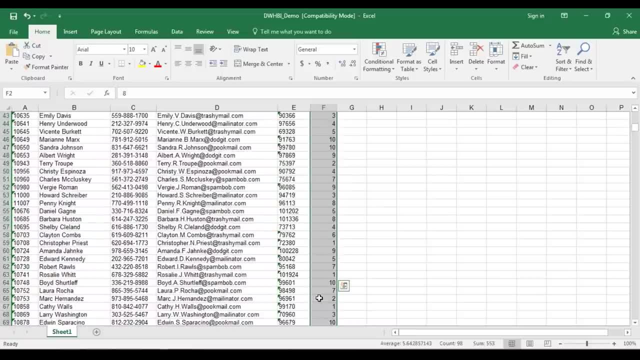 customer phone, the email address, invoice number and the quantity. okay, And the best part is, the quantity here is sorted and it's only that which is less than 10, right, So that was the criteria that we had set. We had filtered for those fields to be only less than 10.. 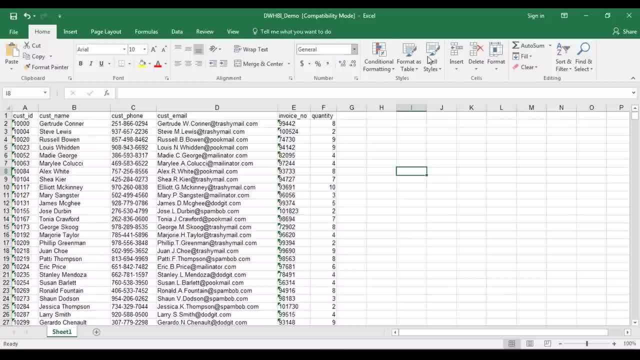 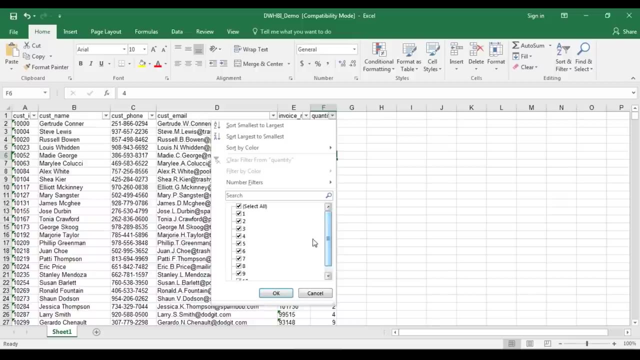 And to show you further proof, what I can do is: I can do this. I'll add a filter, okay, And if you can see here, the only options here are one to 10, okay, That means nobody whose quantity was 90 or 100 plus. 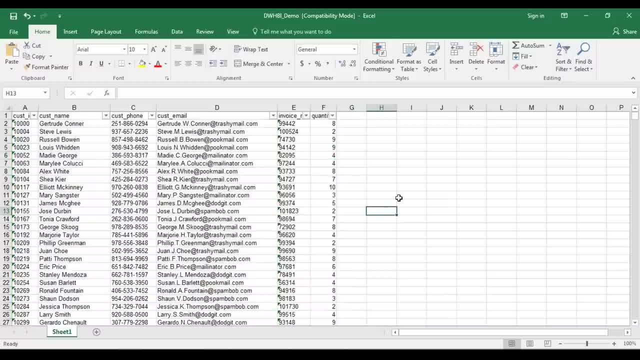 has been added over here, right? So this is how simple Talend is and this is what data warehousing is in basics, right? So this is a very simple example that I've showed you where you can get data into your data warehouse. 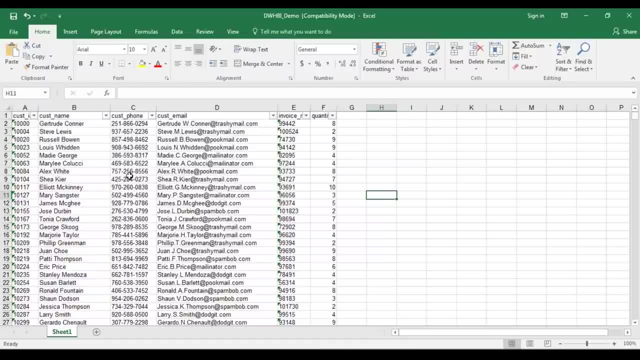 by filtering some data from the database and probably you can use this data to make your analysis or visualization on Tableau or Click-through or any other data visualization, and you can dish 살ks to a very simple tool. but there was another thing that I promised you. 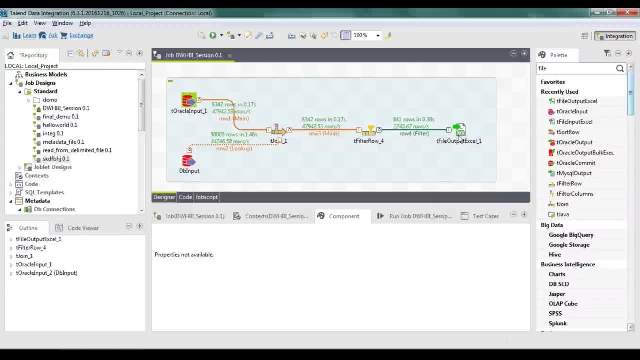 I told you that you will have a filter and you will have another rejected row. so if this was the filter column, I can probably have another Excel here. I can say tfileoutputexcel. so okay, tfileout, internetHands tijd. I'm gonna paste it here and what I'm gonna do is: 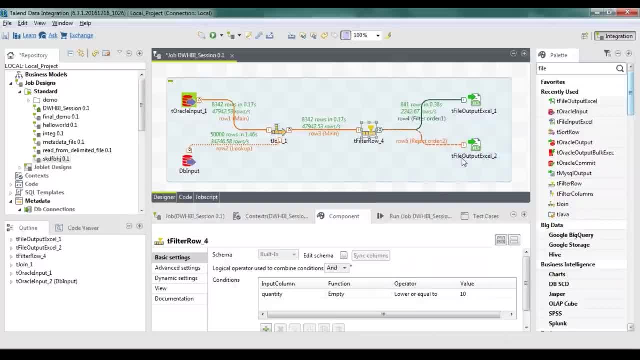 I'm gonna start one when I see a reject and here So the rejected field or row that has been executed here, rows and columns are gonna go into this particular field. okay, so I'm gonna name this also as rejected data, right, so this is also going to be present in the same. 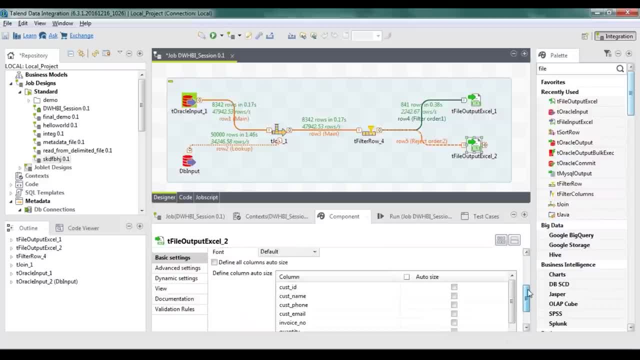 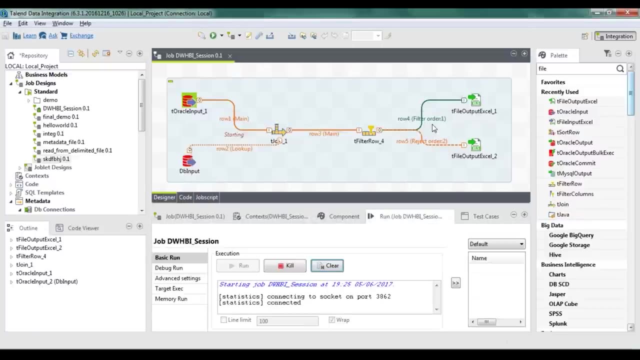 path and let me edit the. I'm gonna say define all the columns size. I'm gonna say include header and yep, I'm gonna save this and run it again. now, run it again. I'll have the same list of fields over here. right, I'll have the same rows. 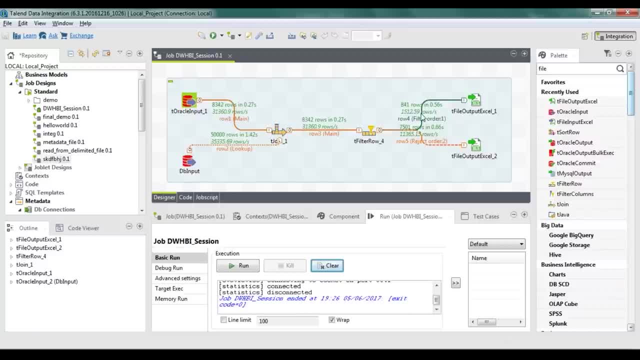 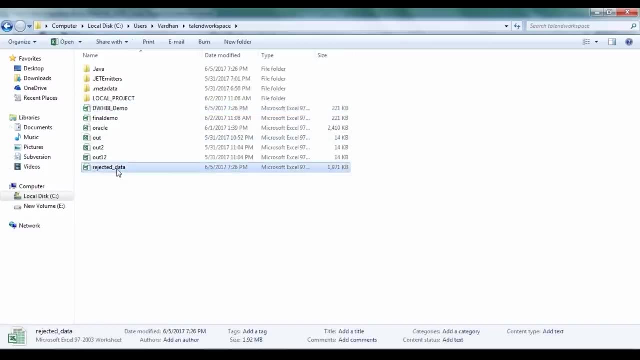 over here, right? so, as you can see, the same 841 rows have been added to this file. okay, the filtered results are here and the remaining ones, which were rejected, they have gone to my new file, and this file is called the rejected one. so if I go back to that same path, this was the original one and the rejected. 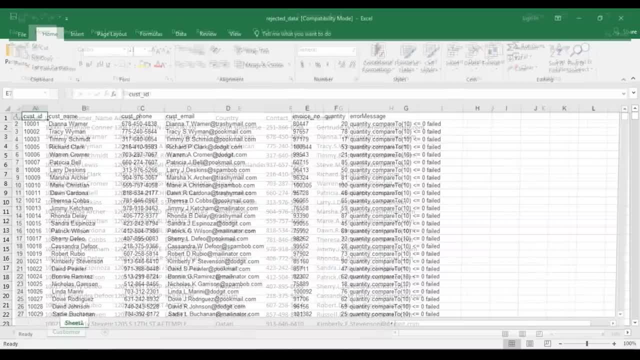 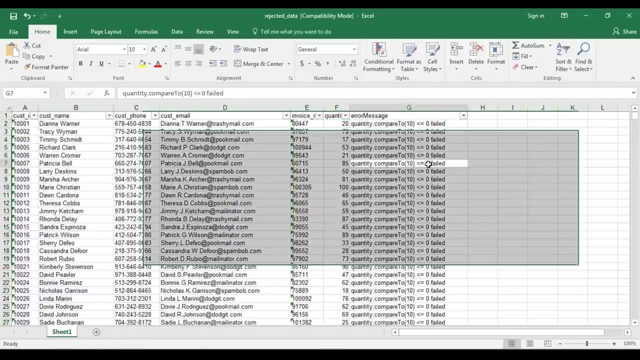 data is here. so when I open here, you can see that the only options here are those of above 10. okay, so if I just show you with a filter column, right, you can see that the only options here are those of above 10. okay, so if I just show you with a filter column, right, 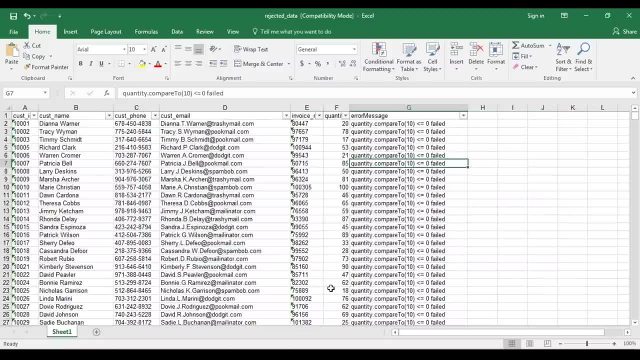 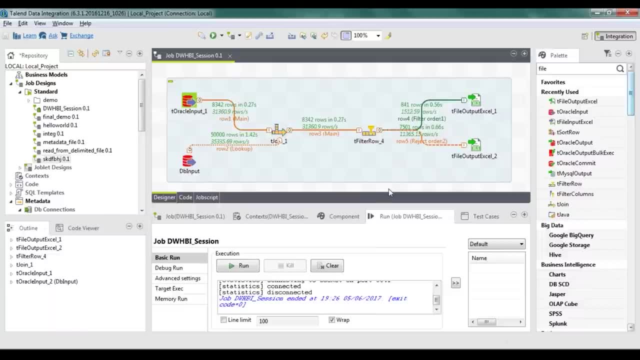 so you can see that there is nothing less than 10. so that's the thing. so that's how you filter data, that's how you get data in and all these things. so that's how you work with talent guys, right, so you get data, and so the same. 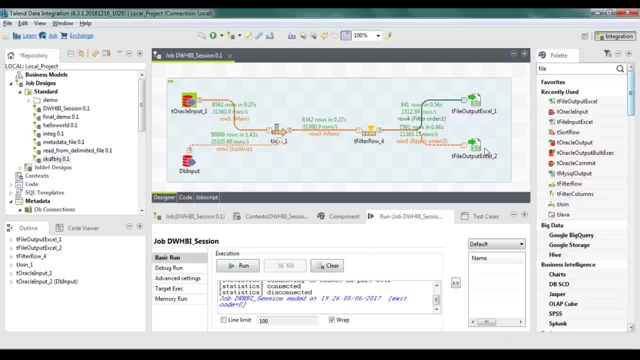 thing here. you can also store it to some database, right? so instead of having a file to excel for this, I can just delete this, and I can just delete this and let me go to databases first of all. all right, so here I'm gonna say Oracle and the Oracle output. okay, I'm gonna paste it here and 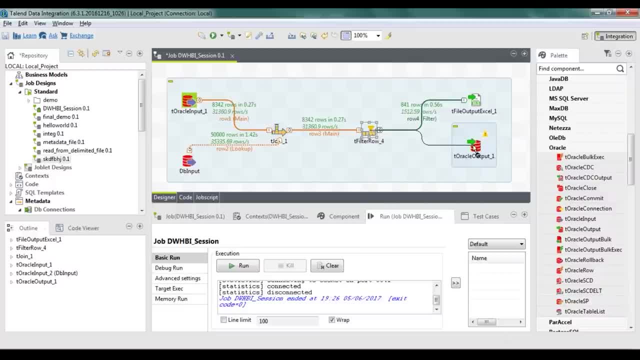 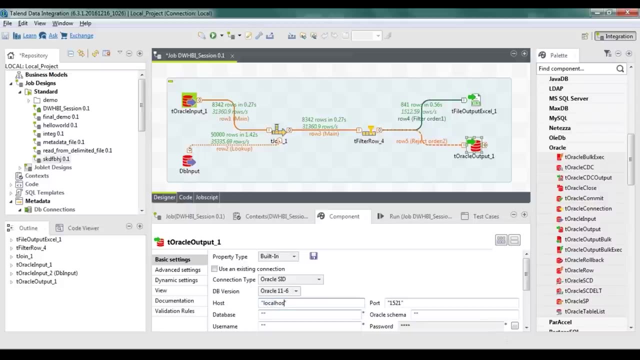 now, if I am gonna say reject or yeah, reject, right, so it's: all these rejected entries would go into this particular file of mine. so let me add the components and edit the components. here the host details: here it's localhost: okay. port is 1521. database is: 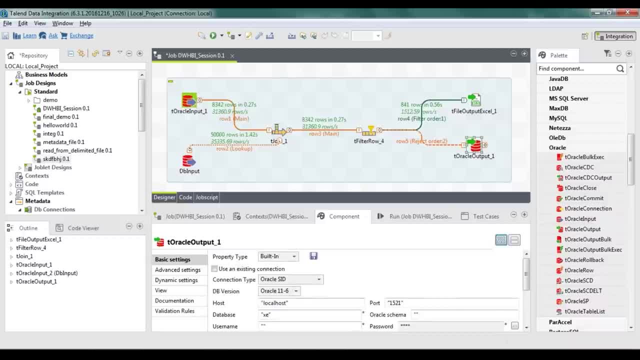 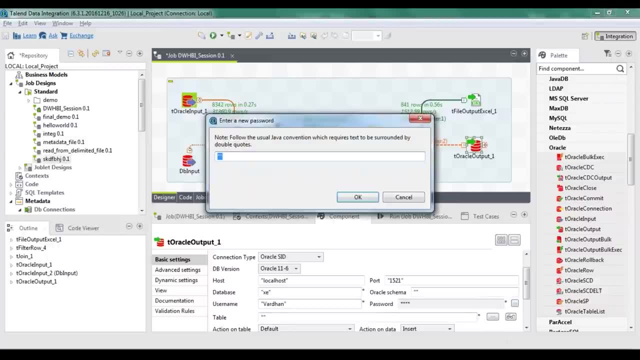 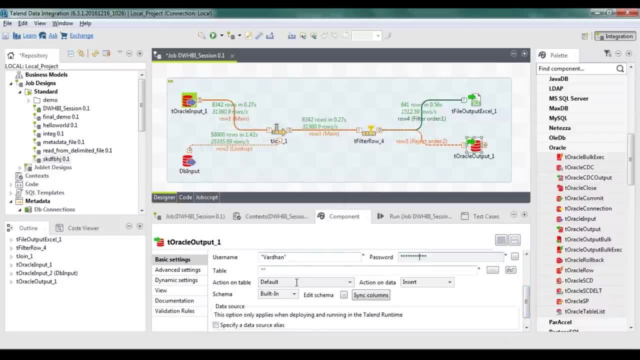 XE. right, yes, it is XE, and my username is- pardon, my password is edureka. all right, so, and then you have the action on table. right, so the action is going to be create table. okay, so when we say create table, we've got to give the table name also, and the table name, let's say reject. 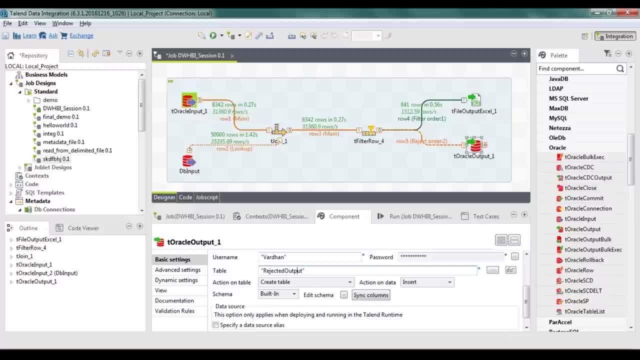 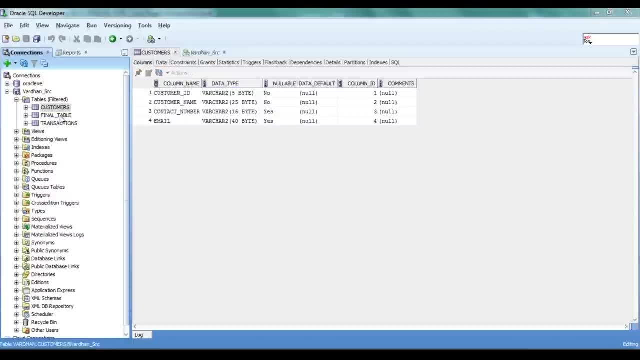 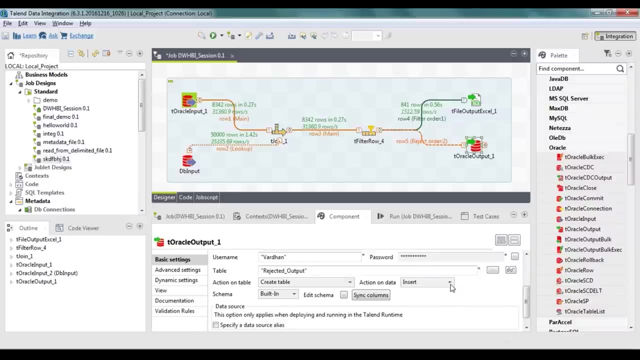 it output: okay, well, I'm getting. there is nothing by that name. yep, there is nothing here by that name. so we have customers, final table and transactions, right. so we will have a new table that will be formed over there. so it's: the action is going to be insert, supposing. 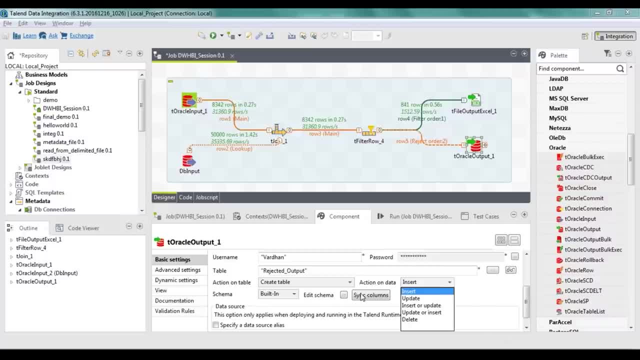 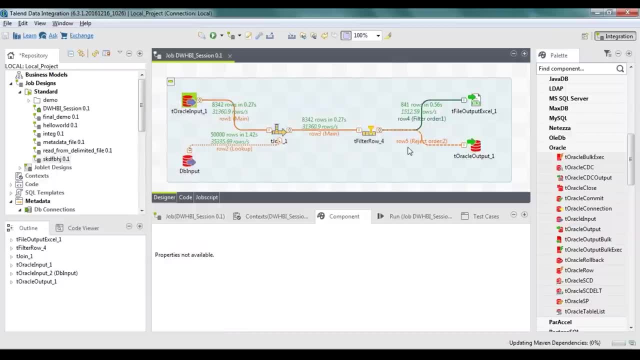 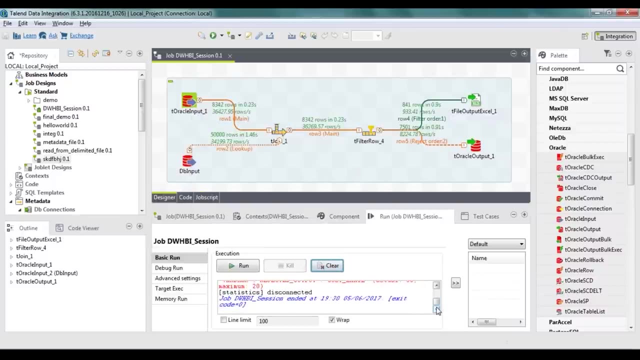 you want to insert or update an existing file, then you can choose the various options, but in our case it would be create a new table and the action would be insert, okay, so let me just save this okay and run this now. so it seems like my new table has been created here. let me just go back to my 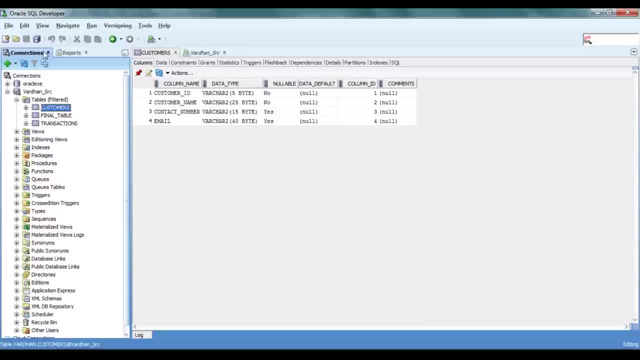 sequel here or actual table, and we need to refresh this. yes, so as you can see, there's a new table that's been created, and when you see here, these are the different fields- error message was another field that gets auto generated and if you look at the contents of the field, you have all these right. 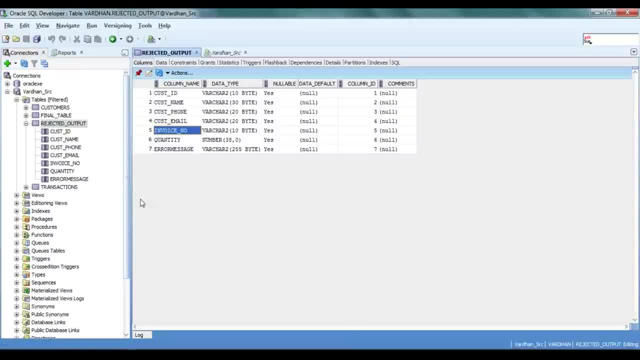 so, guys, that's how you get your data back into your database, right? so earlier I showed you how to do it and store it in an excel file. now I've showed you how to create new table and how to get your data warehouse data back into your. 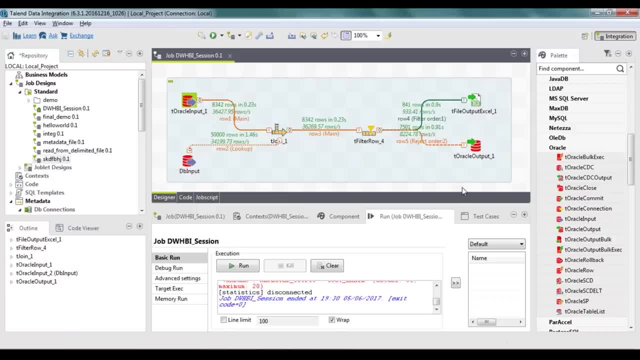 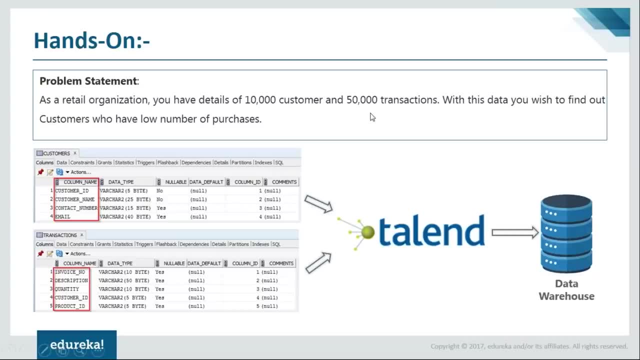 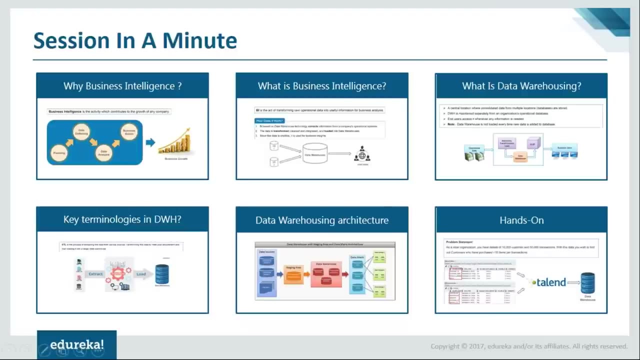 database. so that's the end of my demonstration. all my queries have been passed successfully. now let me just quickly go back to my slides for a minute. and yeah, this hands-on is what I completed: showed you how to get data and your data warehouse, so yeah. so I think that brings us to the end of the session. 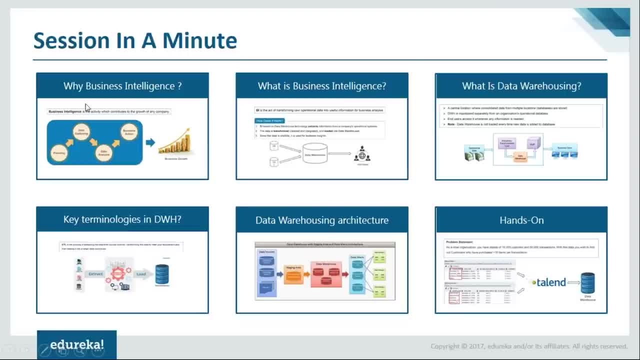 and let me just summarize whatever I did in a minute, right? so first of all, I spoke about the need for business intelligence, and then I told you what is business intelligence, why you need it for your business and what is the role of data warehouse, and then I spoke about data warehousing. right, I went into the 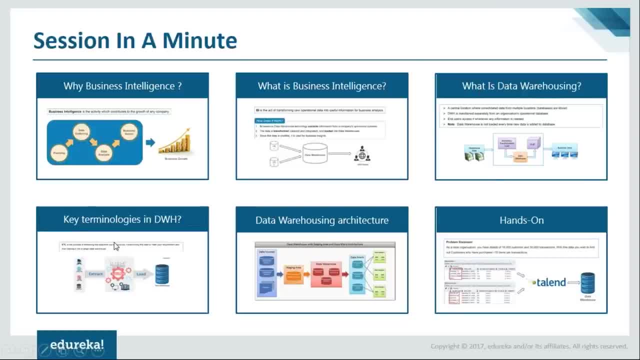 depth of data warehousing and spoke about the key terminologies in data warehouse. we have the ETL, we have data marts, we have the metadata and all these things. so that's the end of my session. thank you very much for watching and I'll see you in the next video. 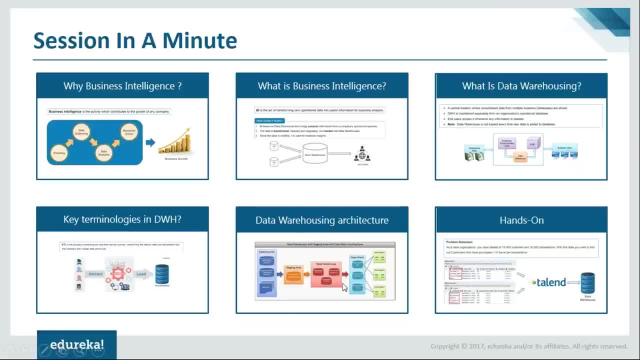 and then, finally, we spoke about the architecture of the data warehouse, and we finish off the session with the hands-on demonstration of how to populate your data warehouse using talent. so, guys, that's it, and thank you for being in the session. that brings us to the end of the session today, probably. 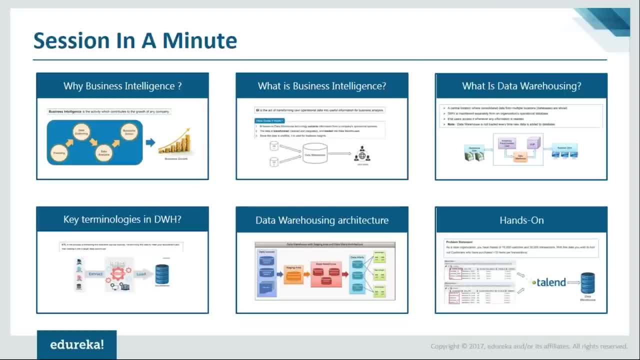 we'll have another session on data warehousing and I'll talk about more advanced concepts like schemas. right, I spoke about there are three different types of schemas, right, like star schema, snowflake schema, galaxy schema, all these things. so I will talk about all these things in my next session and probably 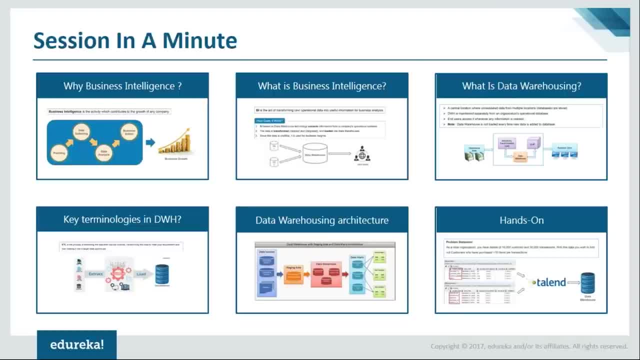 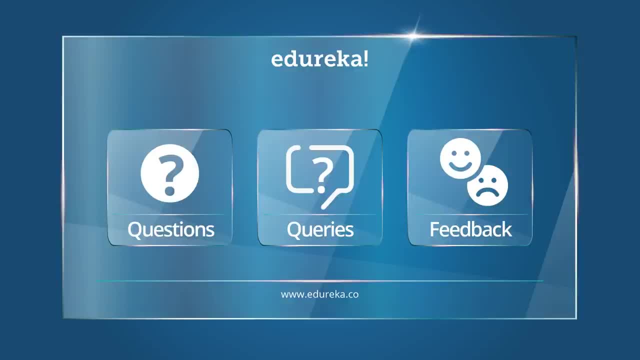 also I will talk about dimensions and fact tables and all these things, right? so it doesn't seem like you guys have any doubts. so if you do have any doubts, please put that in the chat box, right? okay? so, thank you guys. thank you for being in the session. probably I'll see you all until next time. okay, see ya I.